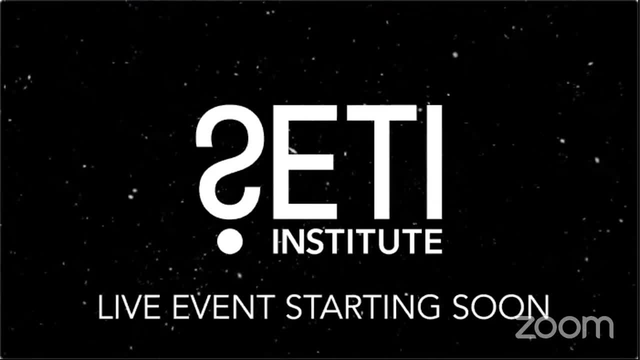 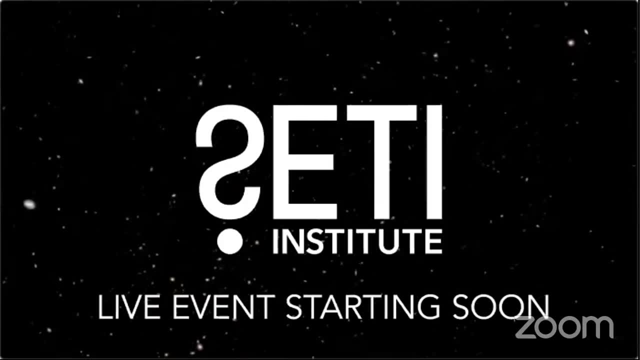 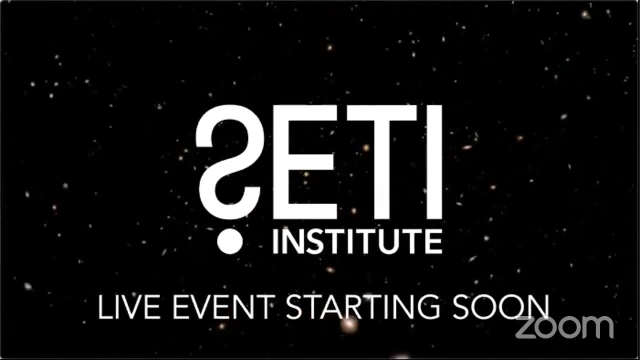 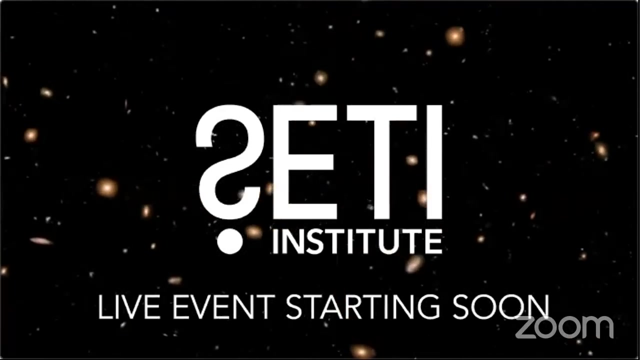 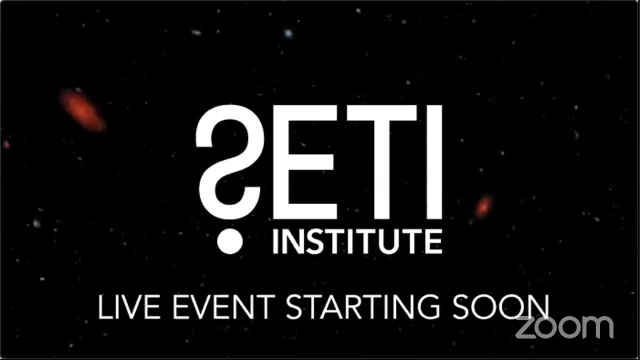 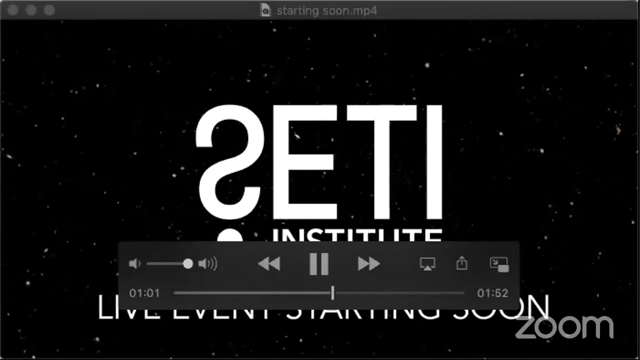 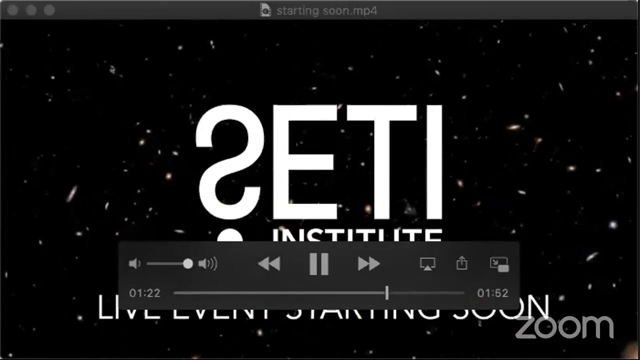 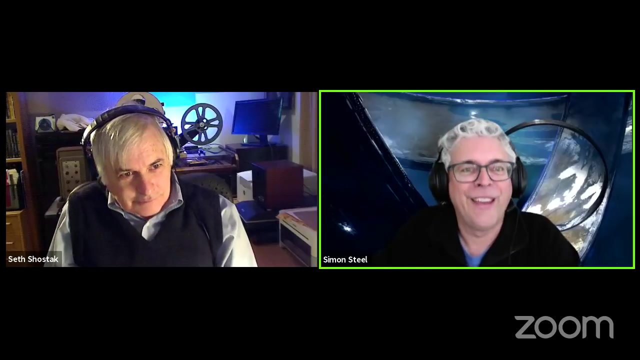 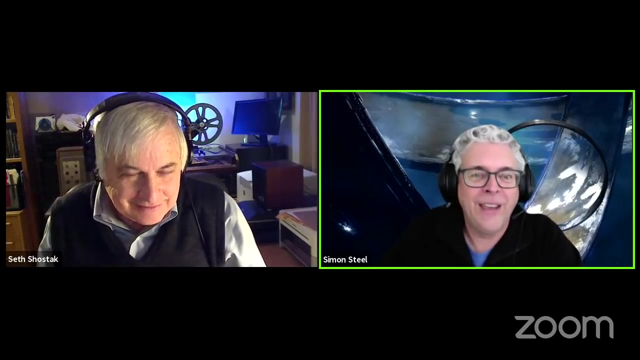 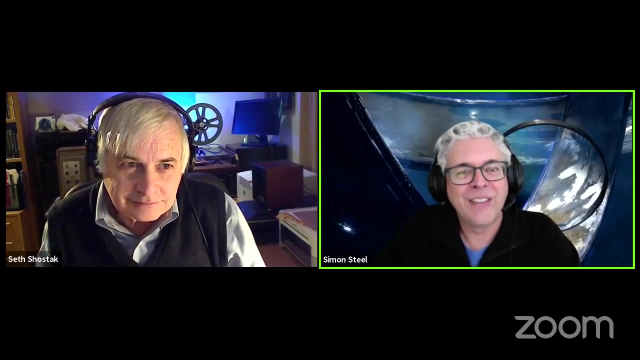 Thank you. Thank you Well, good afternoon, good evening, good morning wherever you are tuning in from, and welcome to SETI Live. My name is Simon Steele, I'm the Director of Education and Outreach at the SETI Institute and I am joined today by Seth Shostak. 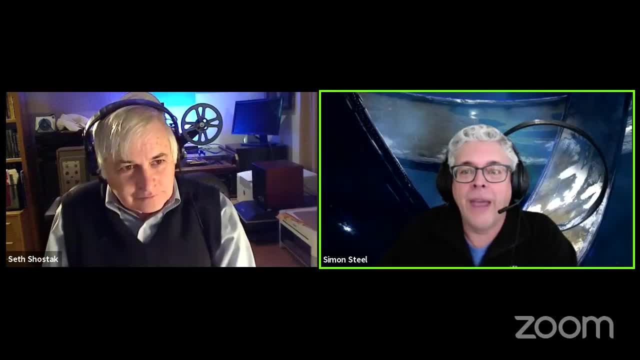 the Senior Astronomer at the SETI Institute, and we are going to talk about the results of a paper that Seth has published. The paper is called The Argument for Artifact Searches, published recently in the Journal of Astrobiology, And, of course, with a title like that, we have to do a SETI Live about it, don't we? 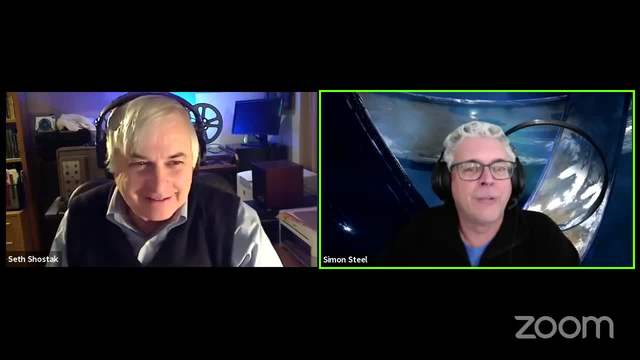 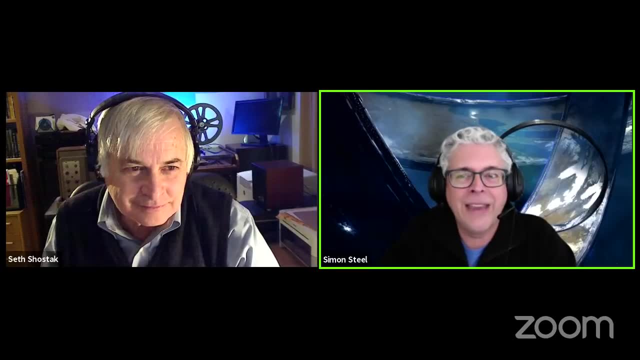 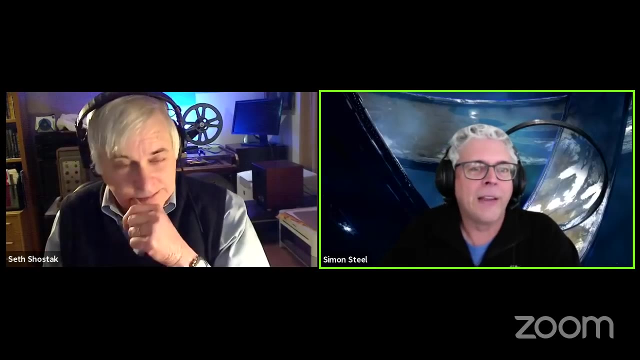 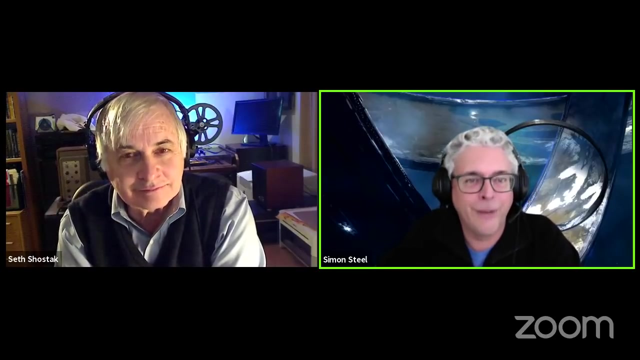 So maybe Seth disagrees. So it's great to speak to you, Seth. This is a fascinating paper and a fascinating discussion on the concept of alien artifacts, And I just want to, before we dive into artifacts themselves, maybe just sort of go back a little bit in time to talk about the traditional SETI searches that have been going on since the 1960s, started by Frank Drake, amongst others, of course. 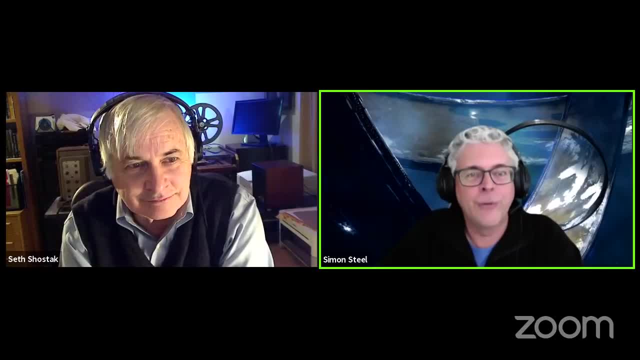 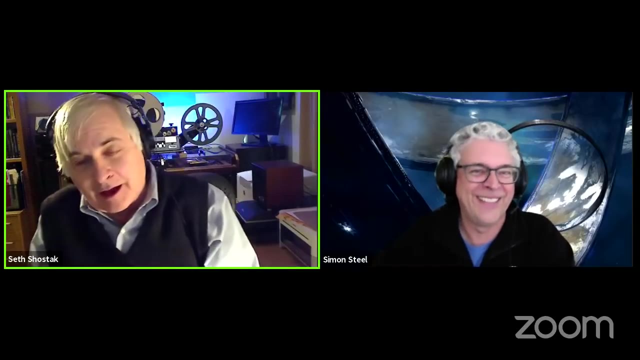 And we are now in 2020,- almost 2021, and we have not discovered technosignatures, signatures from alien civilizations. Why do you think that is? And, Seth, you're muted. Yes, Well, I intended to mute myself for the next hour, simply to spare the audience. 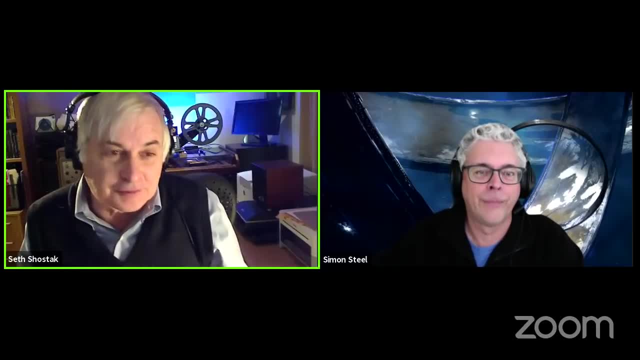 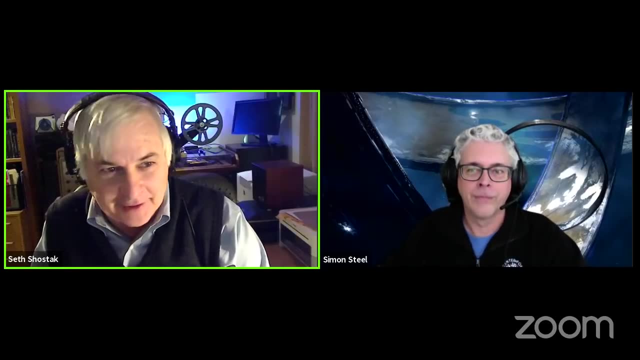 Why haven't we found anything? There are many possible explanations, of course. On the one hand, it could be that we are the only intelligent species In the galaxy. I find that a rather self-centered point of view. Probably not true. Let's hope it's not true, But the usual explanation is simply that we haven't looked at enough star systems. We've looked at, you know, maybe a few tens of thousands of star systems, And that may not be enough. You just have to. you know, if you're going to look for something, you can't give up when you've already only really scratched the surface of the sample that you might need. 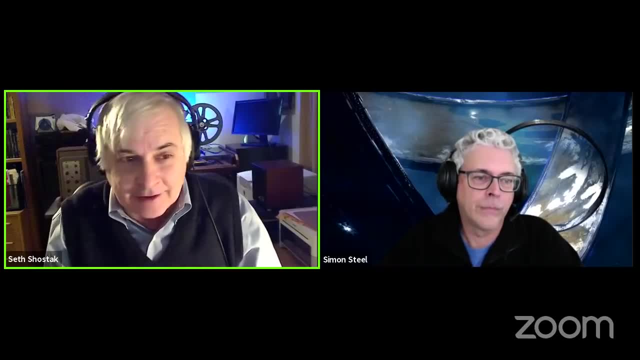 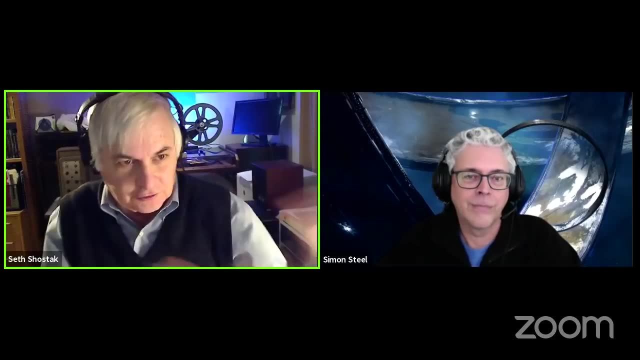 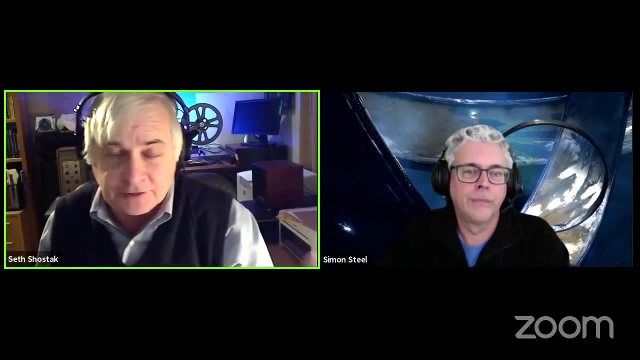 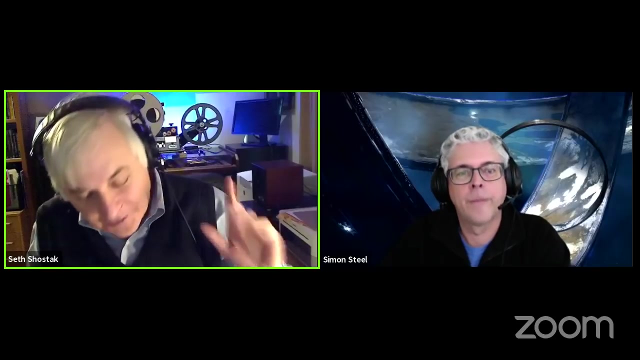 So that might be it. But in the context of today's discussion here's another idea, And that is that when we do a search, a radio search like Frank Drake's back in 1960, you know, we point these big antennas in the direction of some nearby star, hoping that there's somebody on a planet around that star who, for some reason, is broadcasting into space, with that signal reaching us just at the time that we're listening. 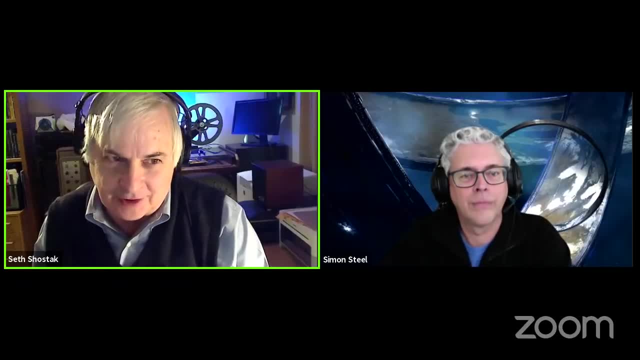 And that may be too optimistic a scenario. Maybe that signal reaches you know, 100 million years ago And our SETI searches aren't going to pick it up. So it was that you know, that sort of disadvantage of traditional SETI, that motivated this paper. 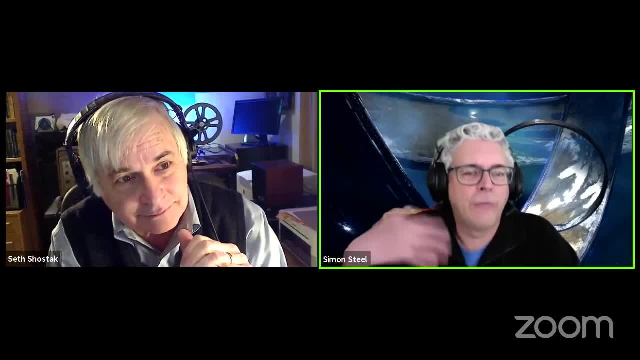 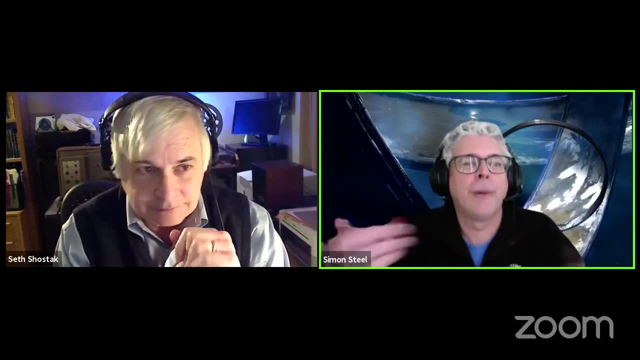 Yeah, And then there's two sorts of signatures you get when you're doing a radio search. of course We've been, as humanity have been, broadcasting sort of isotropically into space for 40, 50 years, And this sphere of radio information is spreading out. 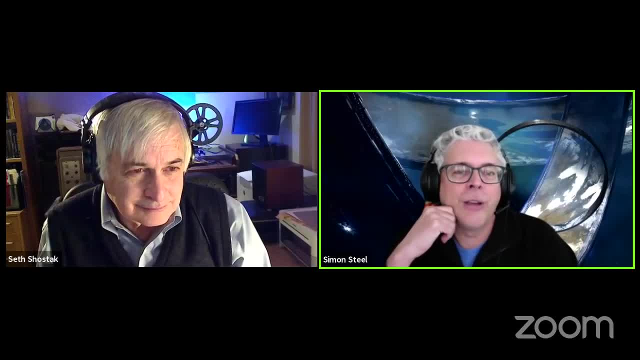 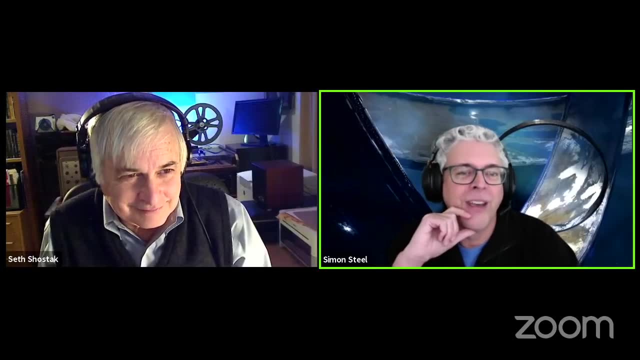 But it's not very strong, is it? And so you can't- You can't actually detect that from very far away. What you really need is a sort of pointed, targeted transmission, But that suggests you need to know where you're going to aim at. 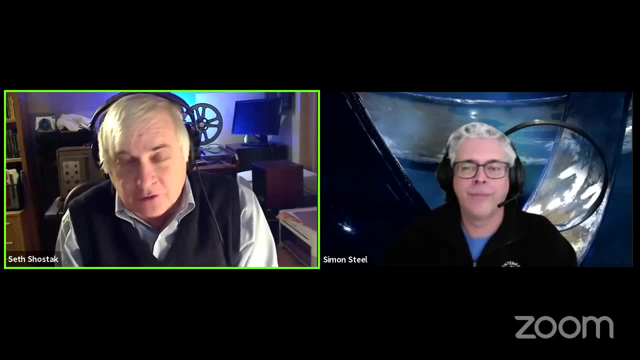 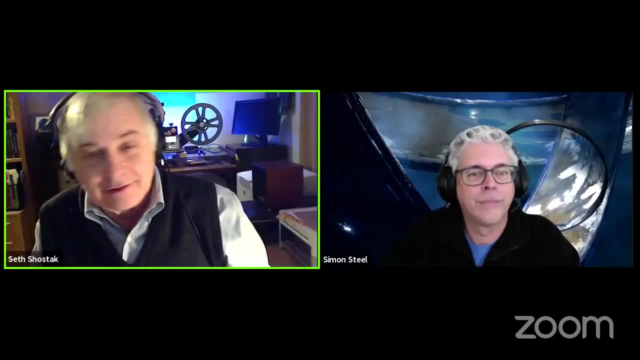 Yeah, exactly, Exactly. I mean, you know people will ask: okay, you guys are looking for signals coming from ET, But are you looking for, you know, just sort of this general noise that any high-tech civilization will make in all the TV stations, all the FM radio stations, all the radars? 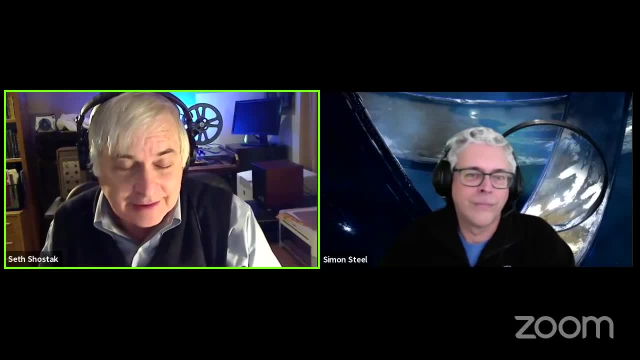 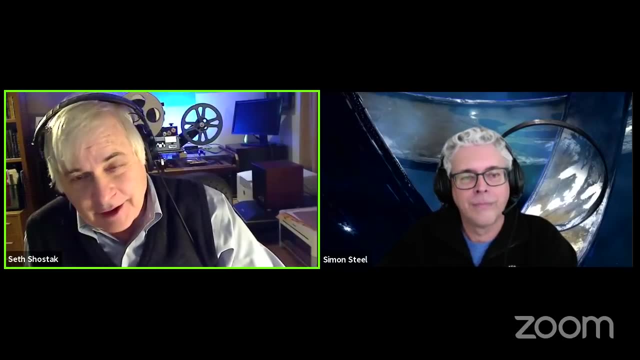 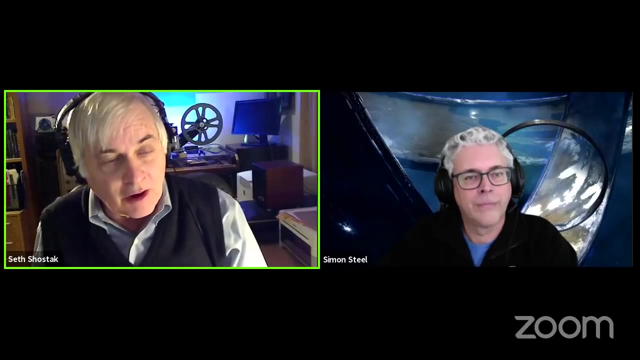 Or are you looking for somebody who's deliberately pinging up And you know, if you're looking just for general noise, that's really hard to find, because that requires much more sensitivity than any of our searches today. I mean, you can work out. could you detect, for example, all the TV stations on Earth from even the nearest other star system, Alpha Centauri, you know, using the best SETI equipment that we have now? 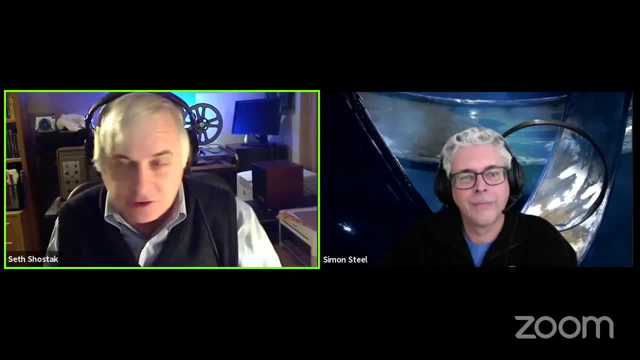 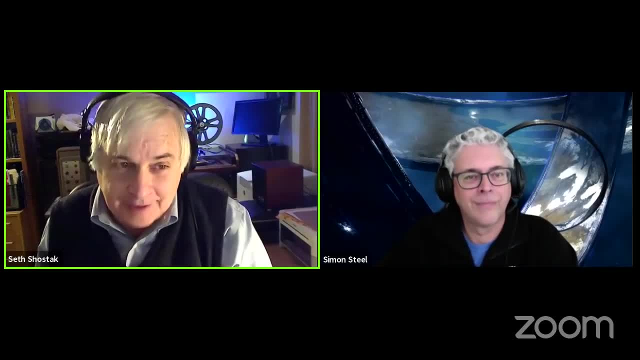 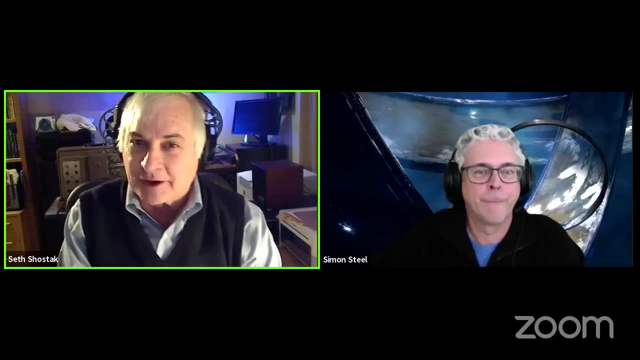 But not with the kind of equipment that we have now. So if we're going to succeed, it's probably not going to be finding that kind of leakage radiation. You've got to hope that they deliberately target us because they want to get in touch, or they've seen oxygen in our atmosphere, or they just have a lot of used cars they want to unload. 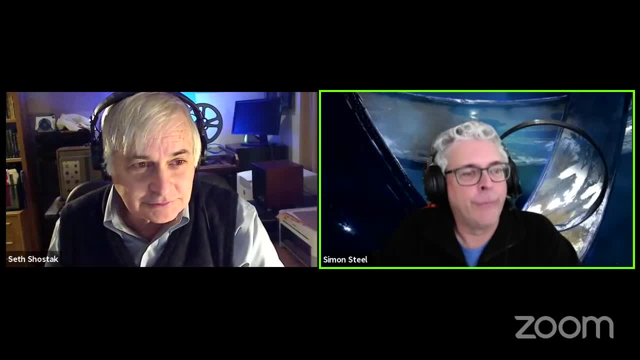 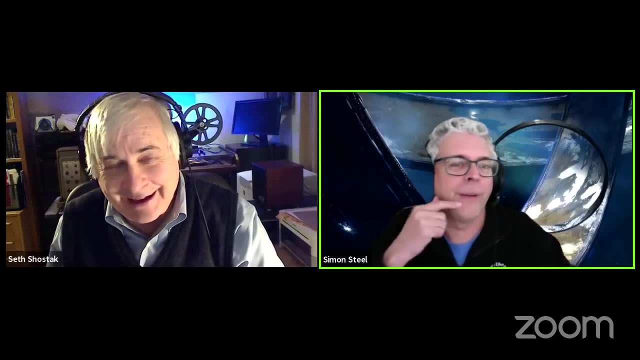 So, on that note, and yeah, as petrol-driven cars are being sort of phased out in the next 20 years, we're hoping that there is a big market elsewhere in the galaxy perhaps. So on that note, and yeah, as petrol-driven cars are being sort of phased out in the next 20 years, we're hoping that there is a big market elsewhere in the galaxy perhaps. 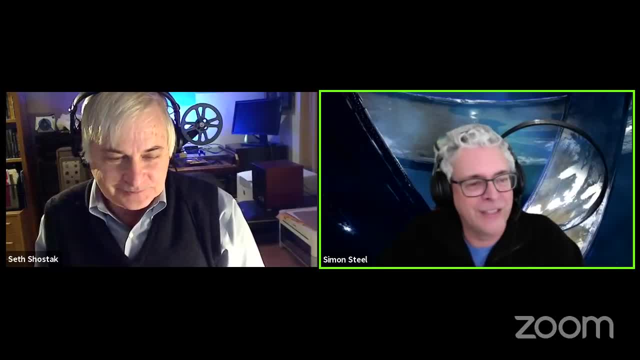 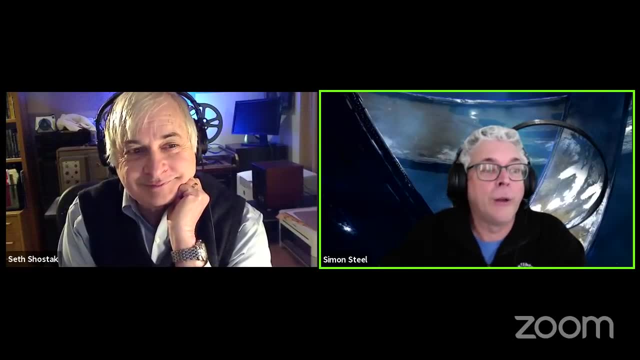 Thank you everybody. I've got a list. Rebecca McDonald is typing frantically telling us where people are listening in: from Berlin, Puerto Rico, Oklahoma, France, Utah, Vermont, Surrey in the UK, Monmouth in Wales, Canada, Estonia, New Zealand. 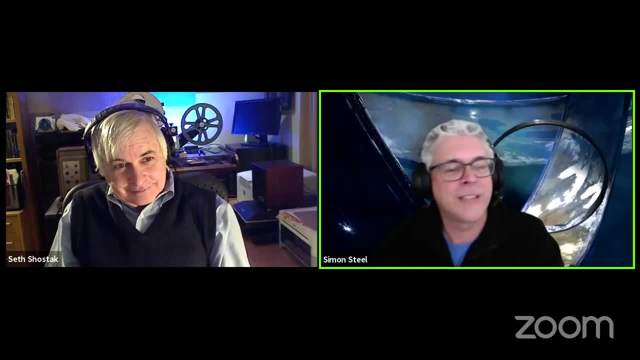 Thank you very much. We'll keep in touch with who's listening from where, And if you do have any questions as well, please type those in to Facebook and those questions will be passed on And we'll come to those in a little bit. 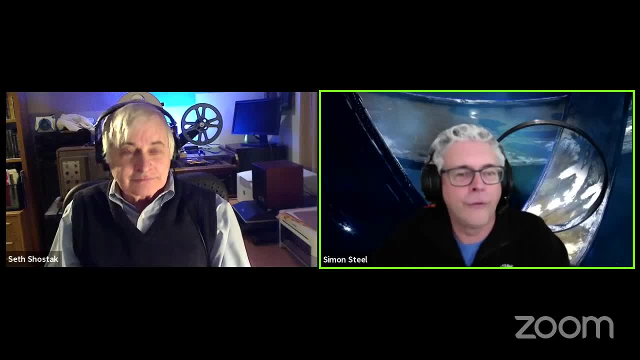 So, assuming that you know we're going to move on from traditional technosignature searches to looking for artifacts themselves, can you define what an alien artifact is? This isn't an Indiana Jones thing we're talking about, is it? 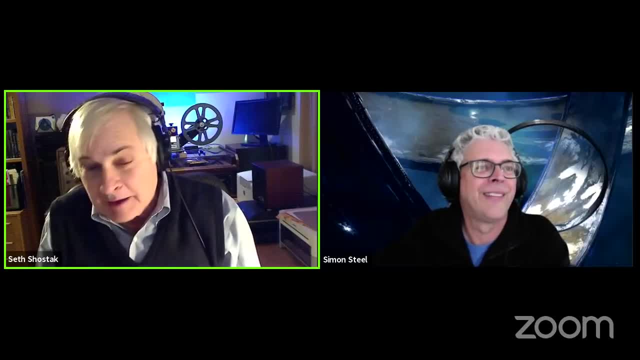 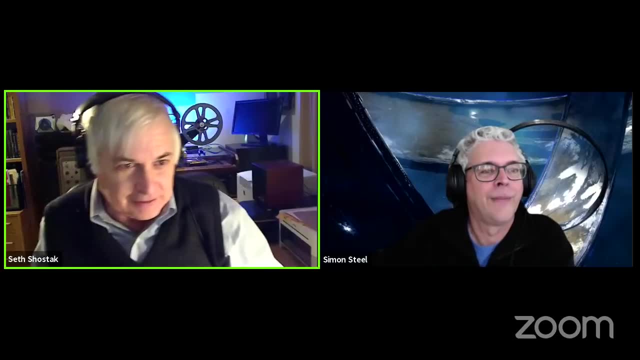 This is something else. Well, nobody actually knows what an alien artifact is. You know, you can look in the movies and they like to make giant monoliths And apparently… The aliens have done that in Utah recently. But you know anything that's out of the ordinary, anything that looks artificial. 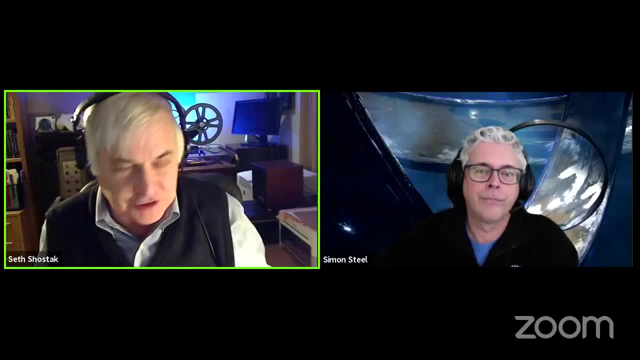 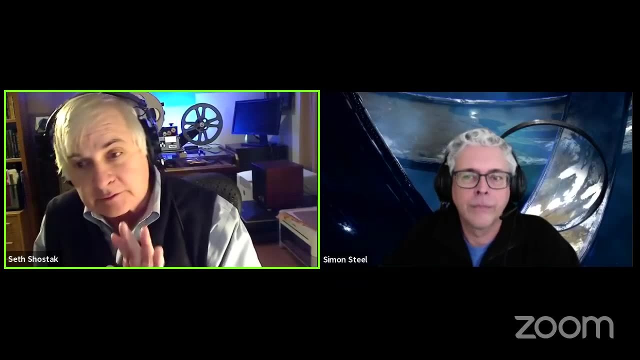 And the reason that it might pay to look for that. I'm not saying we get rid of traditional setting- far from it- But I think that we ought to consider looking for these artifacts, and maybe a little more energetically than we have done in the past. 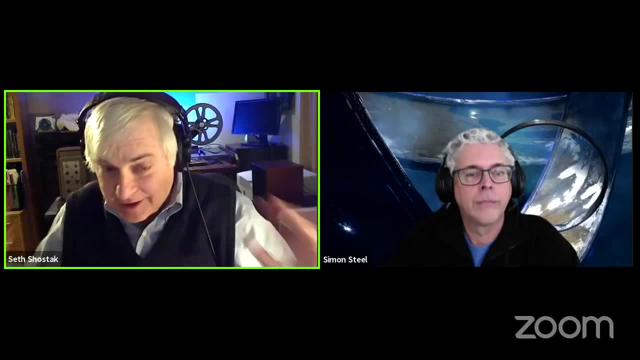 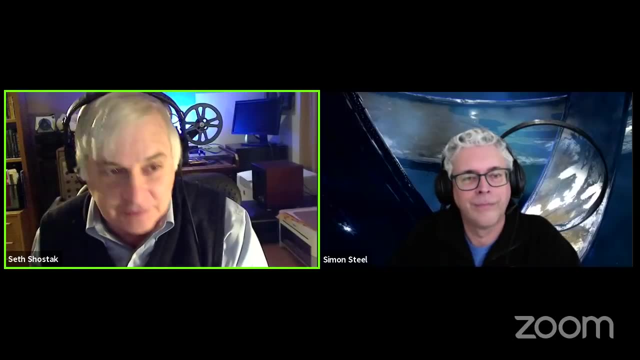 To begin with, they don't have to transmit in our direction. The second thing is, the artifact might be there all the time. I like to liken it to saying: all right, if you wanted to… Find the pharaohs of Egypt, right. 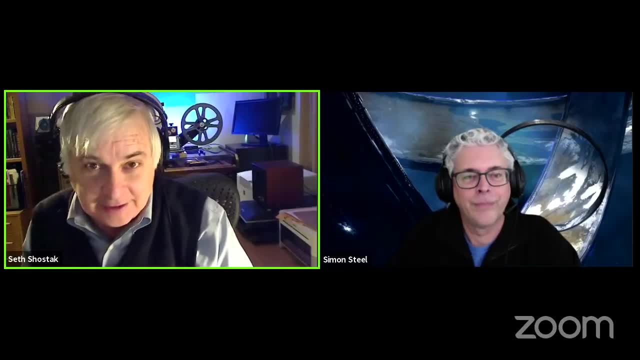 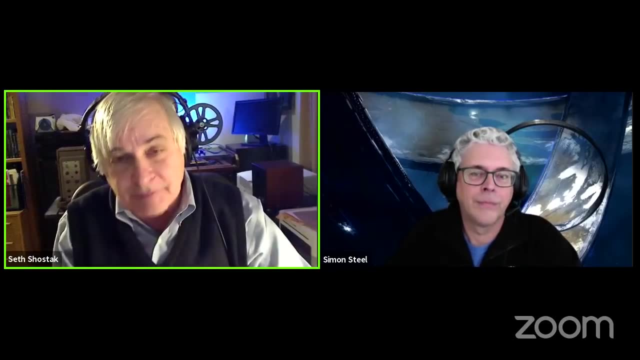 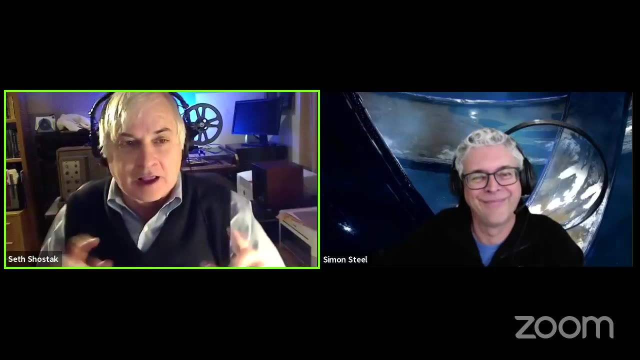 You could fly off to Cairo and look around, but you won't find any pharaohs. They're gone. But you could find the pyramids. The pharaohs have been gone for thousands of years, but the pyramids are still there and presumably will be there for a little bit longer, until you know. air pollution destroys them all. 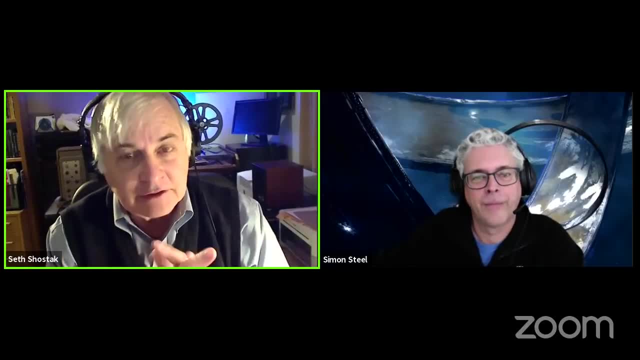 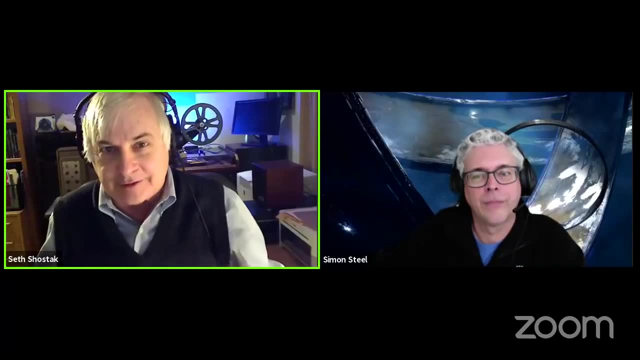 So the point is that if you look for artifacts, you might just have a higher chance of finding something. What could they be? Well, I mean, you know, they could be things like Dyson spheres Or Dyson swarms. 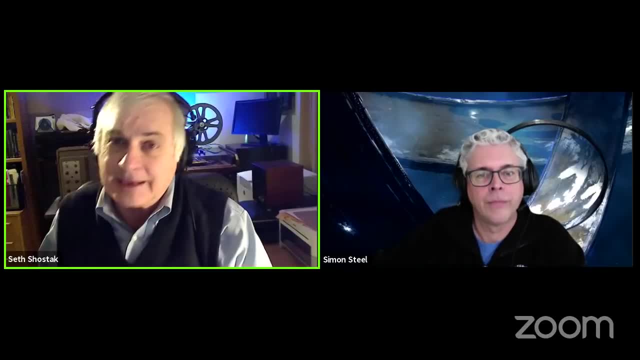 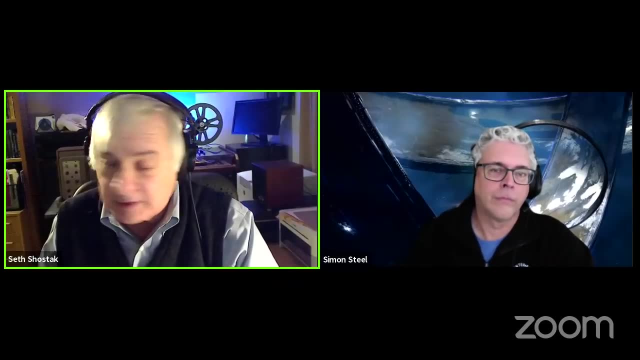 That's what we think of a lot when we think of artifacts, But it could just be anything that looks unusual. It's hard to find these things if you're looking at hundreds of light years' distance, But there might be something, And there are some experiments today that are looking for things that change in the sky that don't look like nature. 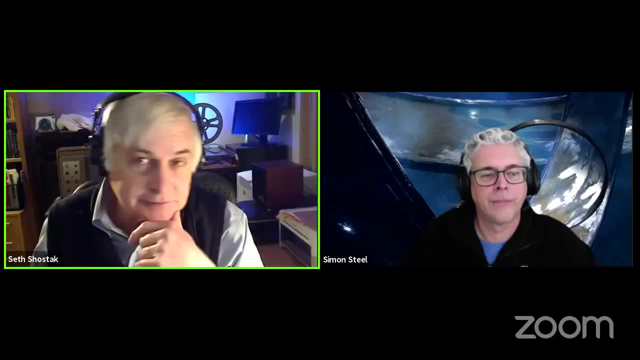 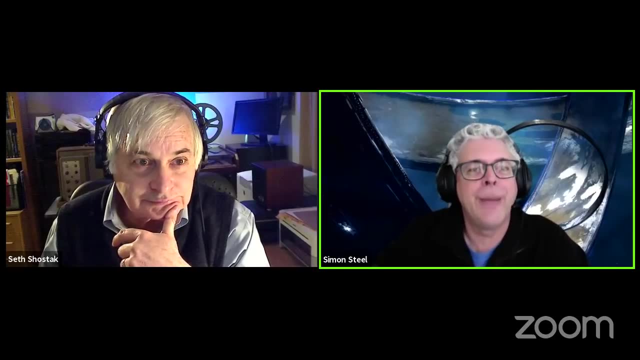 That's the bottom line. You look for something that's not nature. So it's something that, as you say, we think we know what stars… how the structures of galaxies, nebulae are, and they're natural phenomena, but you're looking for something a bit bizarre. 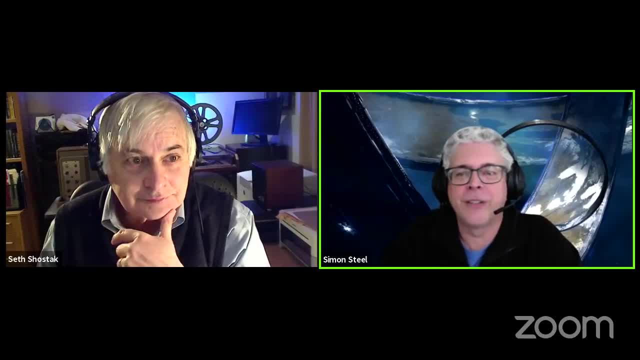 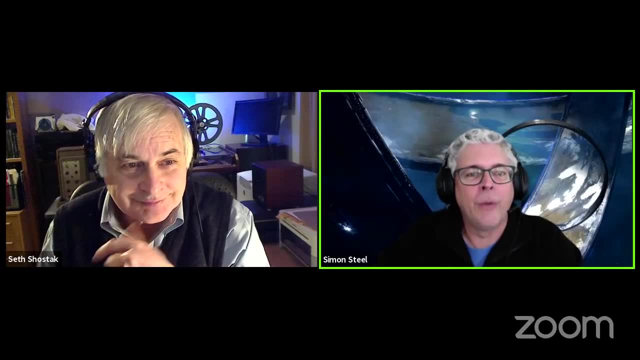 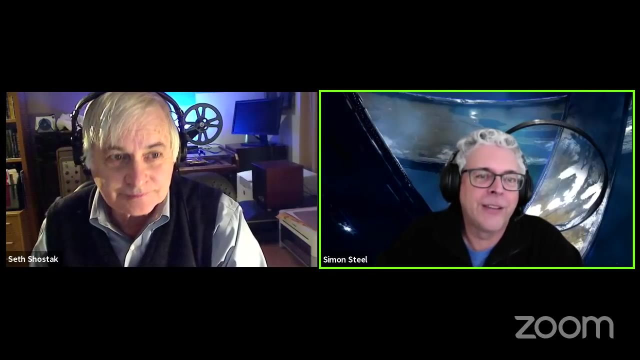 I suppose that maybe leads us on to the subject of something that probably isn't an artifact, and that was the discovery of Boyajian star. We now have, you know, an ability to detect planets around other stars, exoplanet searches, and we've now almost 5,000 planets around other stars that we've discovered. And planets around other stars. we've now almost 5,000 planets around other stars that we've discovered And planets around other stars. we've now almost 5,000 planets around other stars that we've discovered. Planets are an understandable shape. 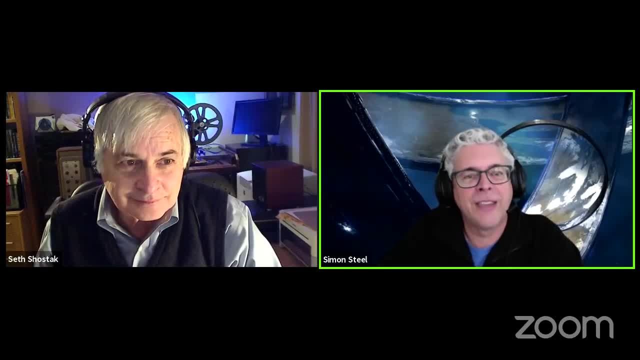 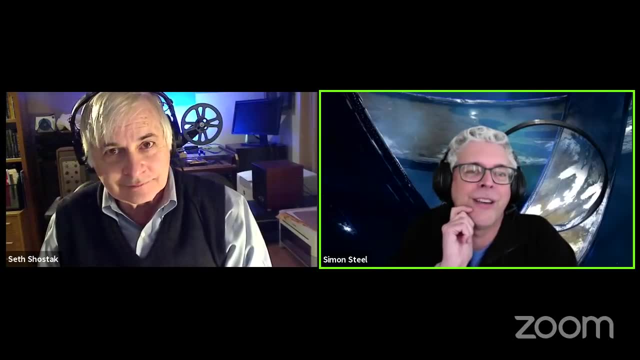 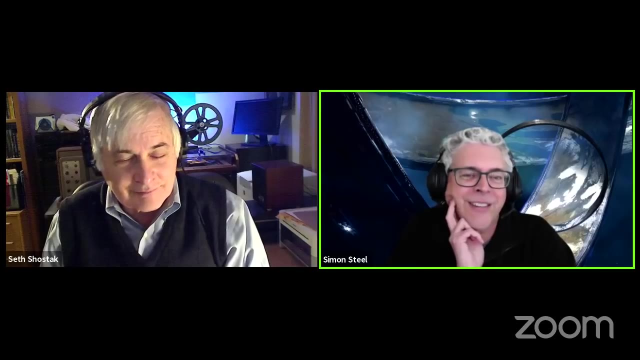 And if they are moving to eclipse their star, they have a characteristic signature of what happens when a planet passes in front of a star, And how can this lead us to some ideas of how we could possibly search for artifacts? Yes, this is a new project, as we know it, the SETI Institute, because one of our owners is involved. 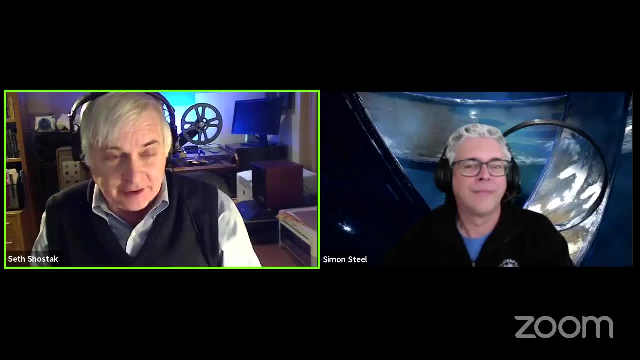 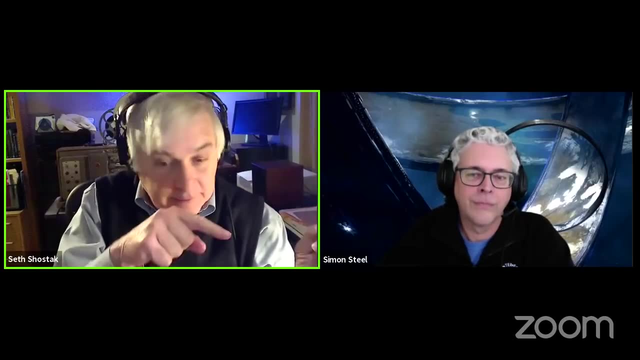 Anne Marie Cody has gotten some money from NASA to do this, this kind of project, and they're just going to look essentially at data from the test space telescope and maybe even kepler, but in any case the data that shows how bright a star is as a 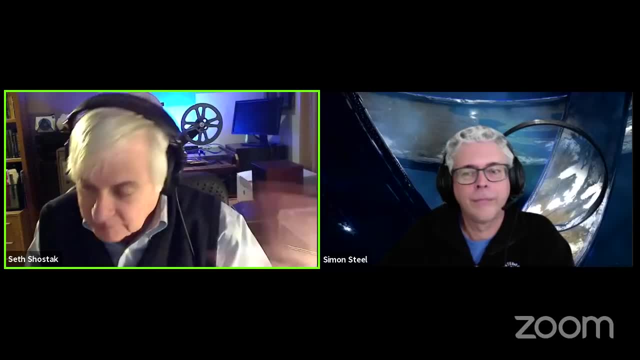 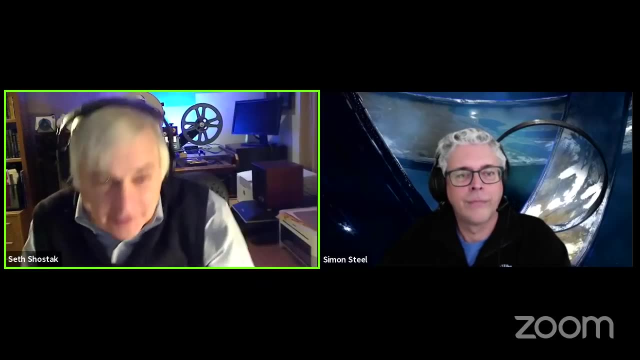 function of time. so if you were to go out every day and look at the sun- not recommend, it's not good for you, but if you were to do that- you would see that the sun is essentially the same brightness every day. it varies a little bit because of big sun spots and that sort of thing, but those changes. 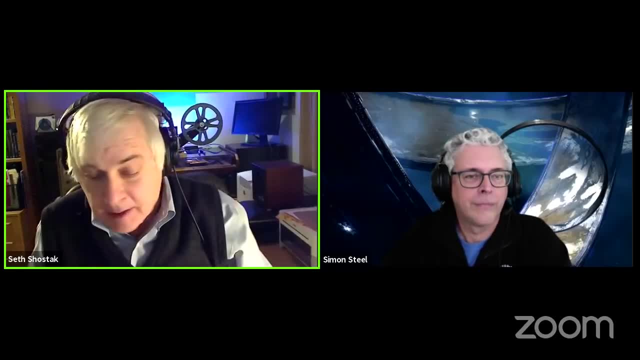 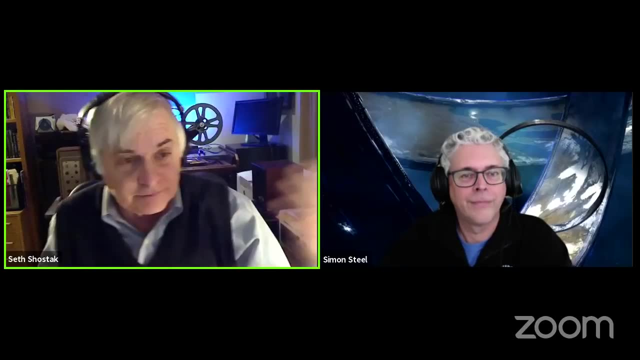 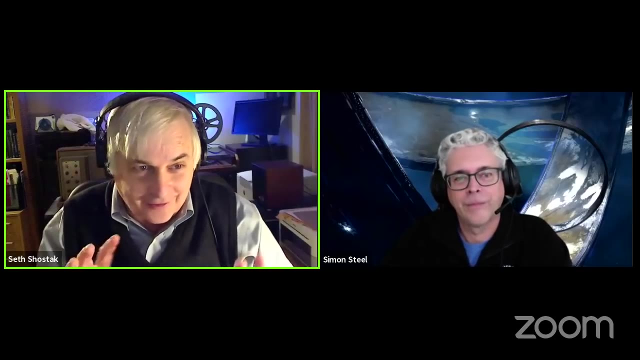 are very, very tiny, so the sun's light output is the same, but there are stars whose light output changes, and not because of a transiting planet, but for some other reason. something might be getting in the way- a comet tail or something like that, or it could be that the aliens are. 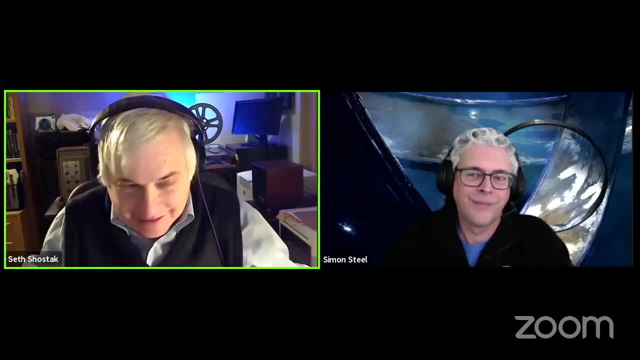 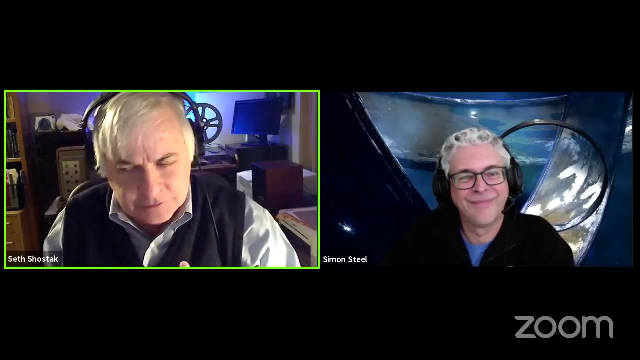 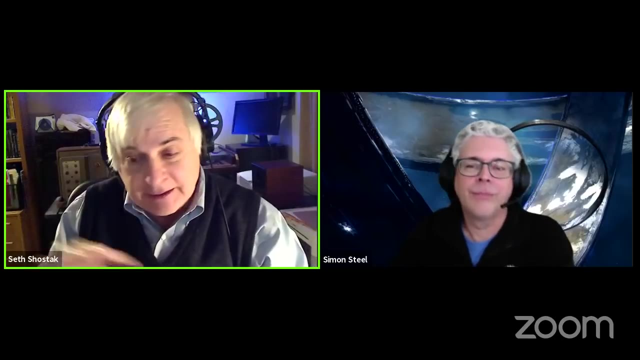 you know, in that system, and, and they built something big, really big, uh, as, as douglas adams would say. so no, like, maybe it's a shatner who says that, william chad, well, somebody says it in any case. and so you know, if they built something really big, if i'd. 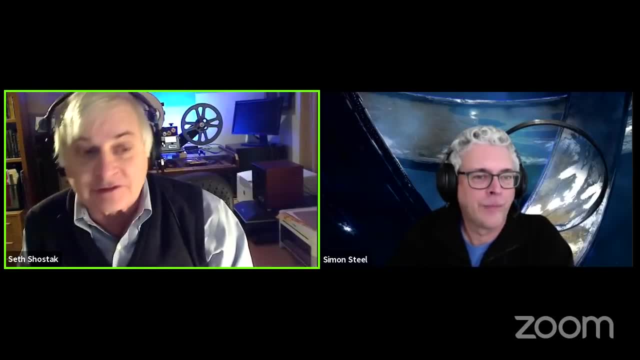 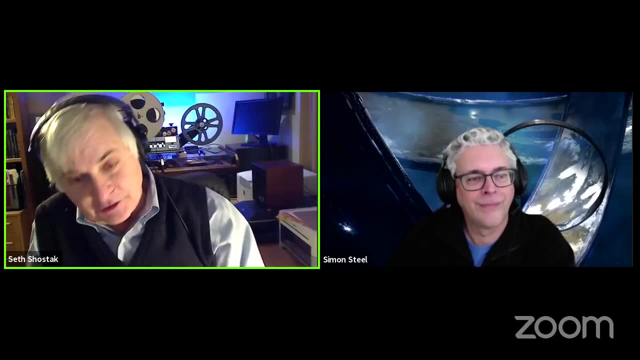 occasionally get in front of their stars, see from earth, and we might discover it that way. if you can't find a a natural explanation for this thing, then you have to say: well, bob, i still don't know what it is, but it could be aliens. so you've really got to rule out the 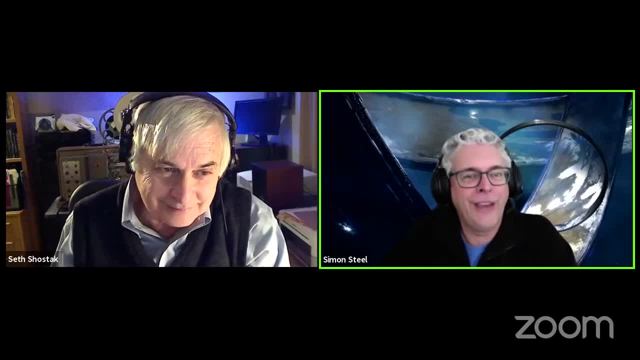 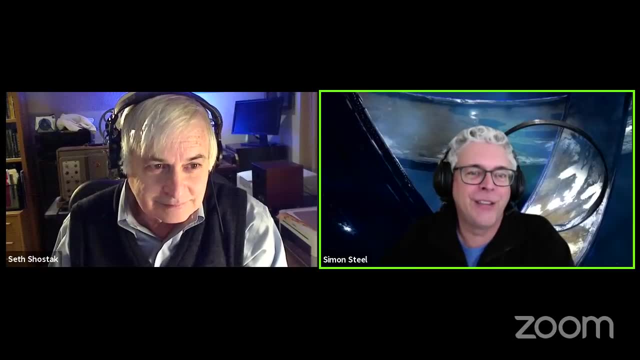 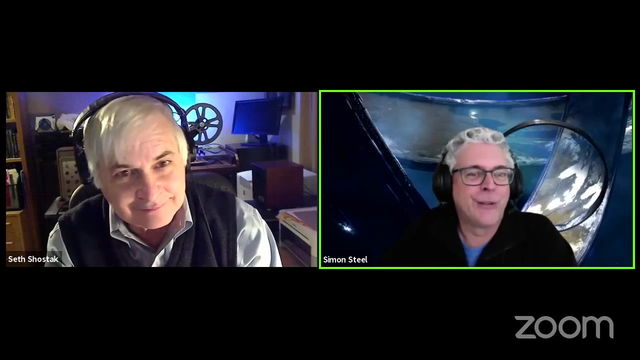 natural, and that's not necessarily easy, because they're still wonderfully, uh, one nature's still throwing wonderful things at us, um, an example being fast radio bursts that are the very, very rapid radio signals. um, you know, humans have have been optimistic about radio signals for some time and their, their origins, uh, that are not natural. uh, pulsars was one of them, and it turns. 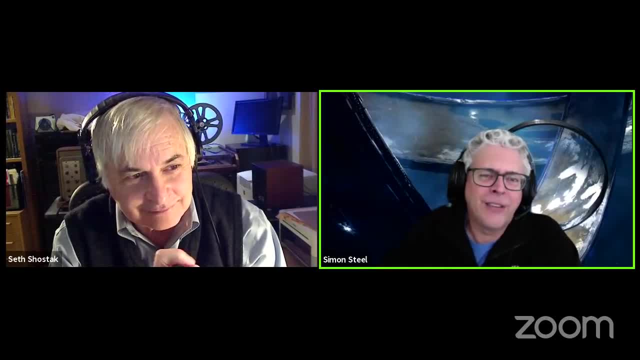 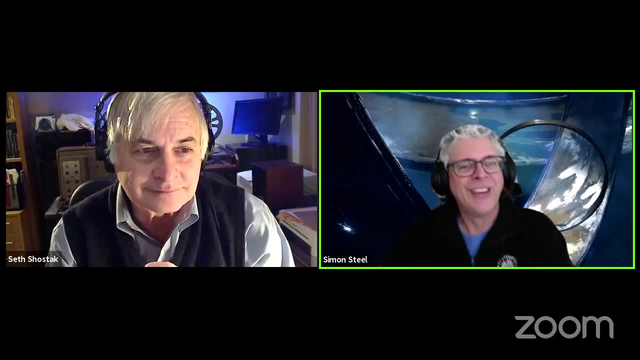 out. you know, frb is fast radio versus another one. uh, they, they seem. how can, how can nature make these weird and wonderful things? but nature has a way of of making weird and wonderful things and confusing us. um so, uh, dyson spheres you mentioned now that. 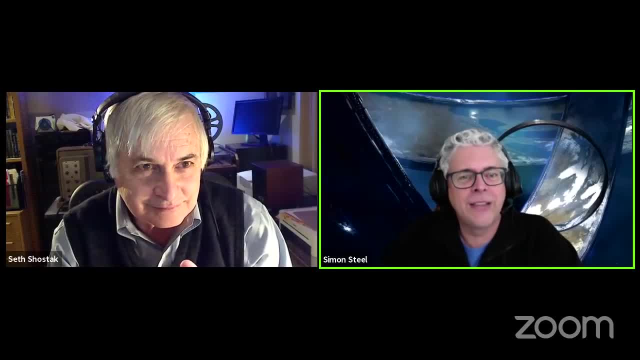 you know, if we're going to find these things around other stars, they have. these things have to be pretty big, don't they? you're not going to detect, um, elon musk's tesla, uh, anytime soon. so what? what's the what's the limiting constraint of finding uh artifacts if you're looking around other stars? 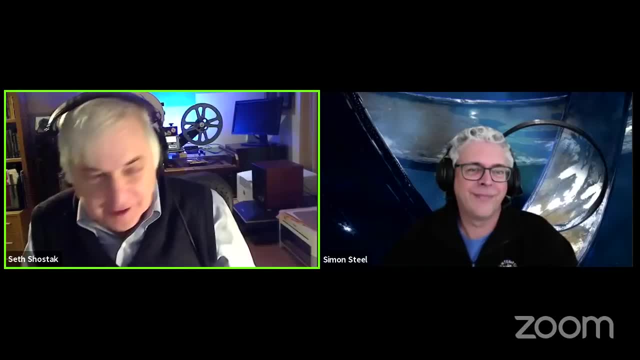 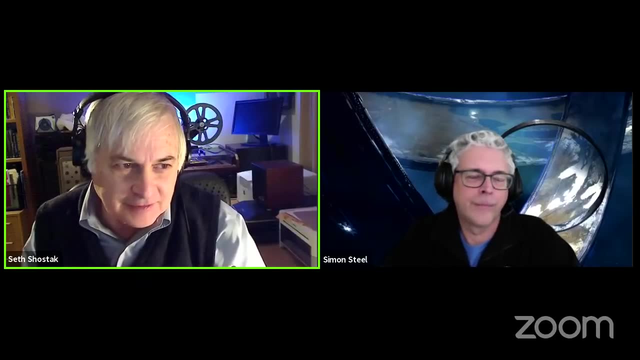 well, if you're just going to deliberately image them, maybe that'd be the way to find uh, mr musk's tesla, you know, just take a big telescope and just look for it. but if you're talking about something the size of uh, well, something big. 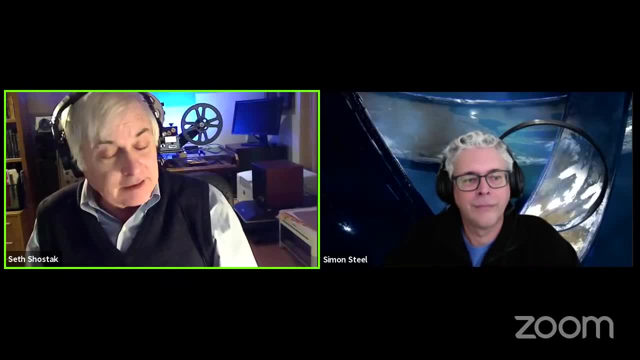 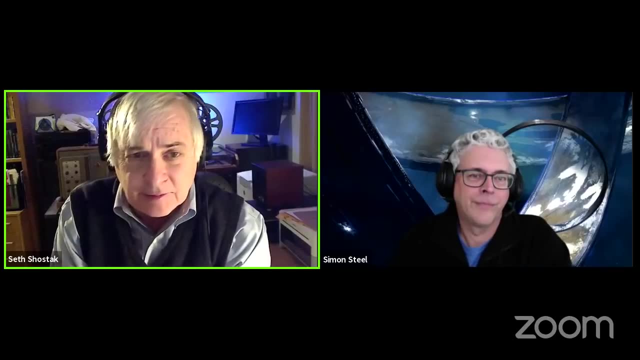 let's say something big and it's hundreds of light years away. even our best telescopes are going to have a hard time seeing it directly. in fact, there's a little calculation in the paper, i think, where, if something is 300 light years away- and i take that as a distance to the nearest- 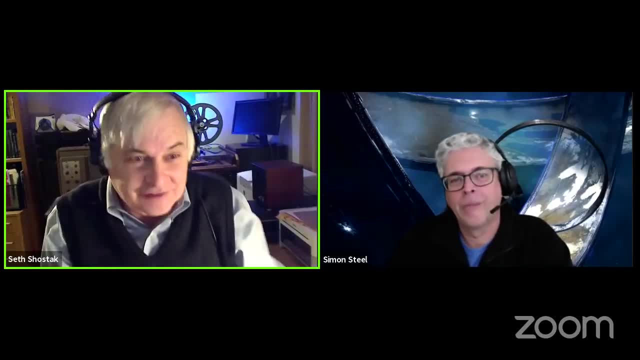 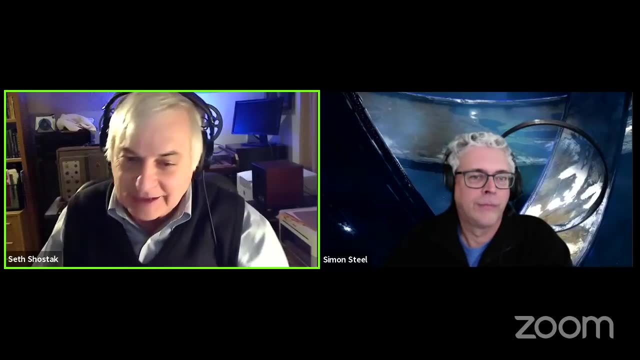 aliens, because i figure that's- you know that contains a million star systems. there are million stellar systems within 300 light years. so if you say, okay, you know you need a million to find one alien inhabited planetary system, then there's a million star systems within 300 light years. 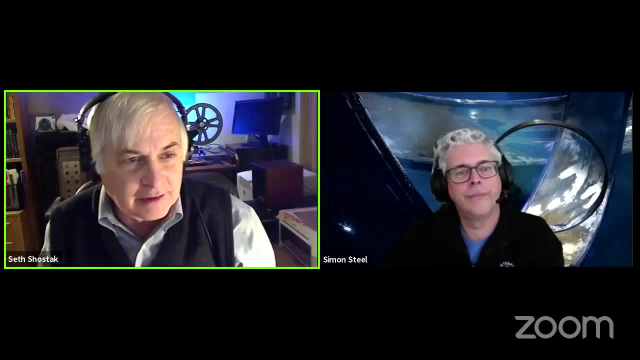 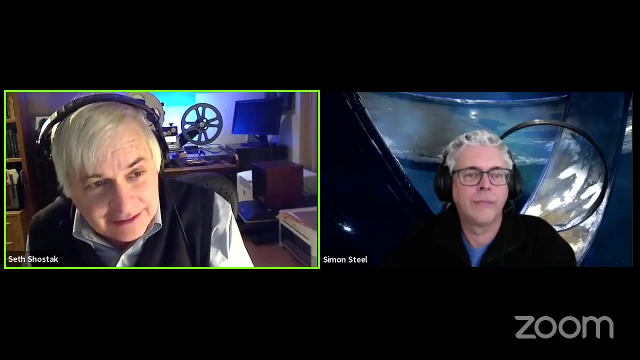 300 light years away. So what could we see with our best telescopes at 300 light years? Well, it'd have to be the size of the state of South Dakota for us to be able to see it, and also have to be bright enough, And maybe that's too big for the. 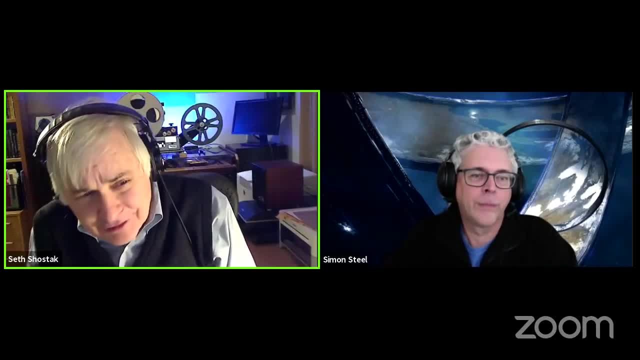 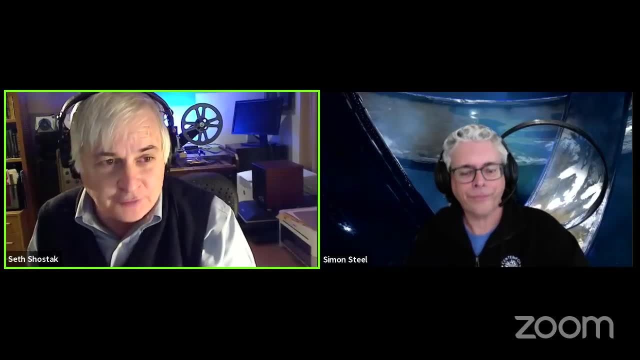 aliens to build. you know to build, But is it really? I mean, you know we've had a technological civilization for hundreds of years, but the aliens may have had it for millions, conceivably billions of years. So don't sell them. 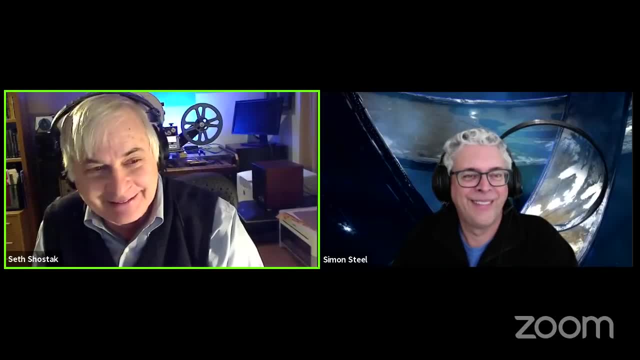 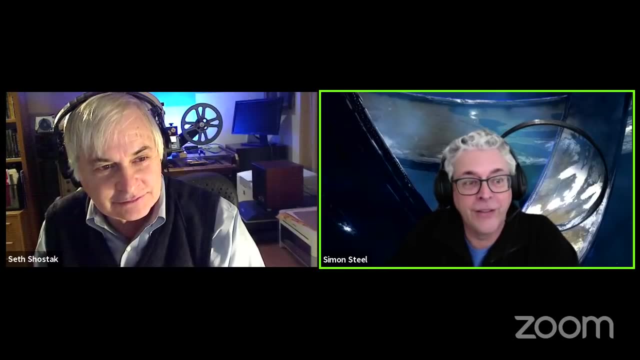 short. Maybe they really have built something very big. Yeah, We got lots more listeners coming in here. Thank you very much From Estonia, New Zealand, the Netherlands, South Devon in England, Ohio, somebody from the Bay Area. We've also had a. 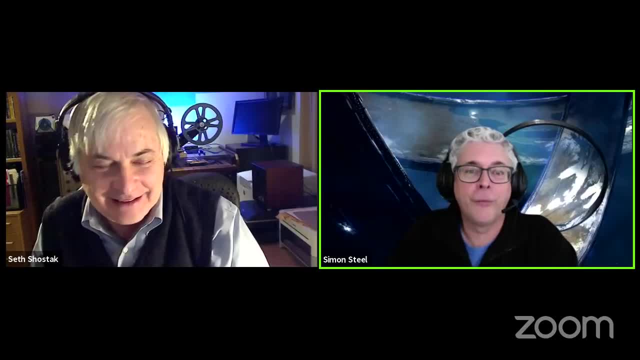 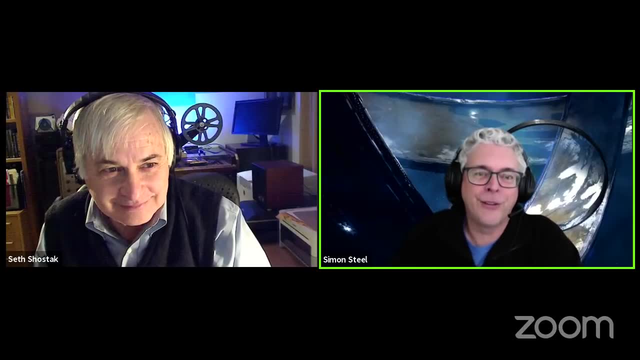 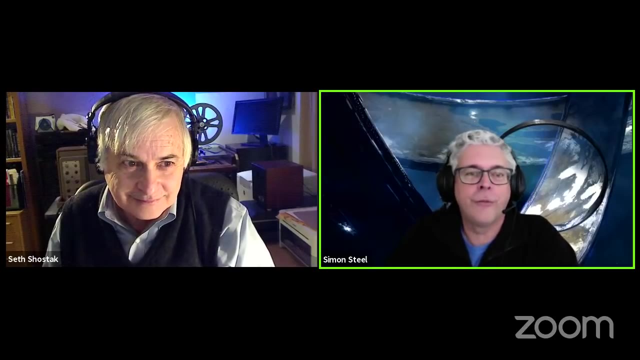 donation. Scott, thank you very much for making a donation. You can make donations on Facebook. I just remind everybody that the SETI Institute is a nonprofit organization. We rely on donations to keep us going. We get money from NASA contracts as well and NASA grants, that's true, But a lot of our 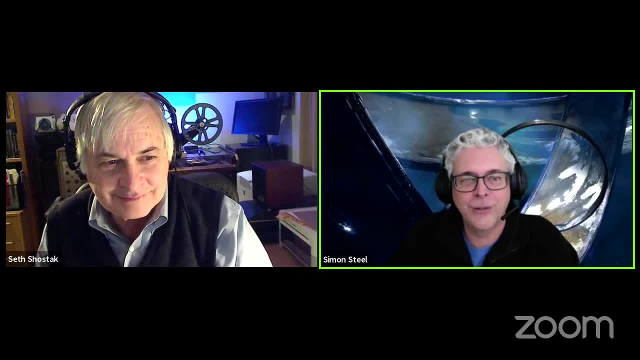 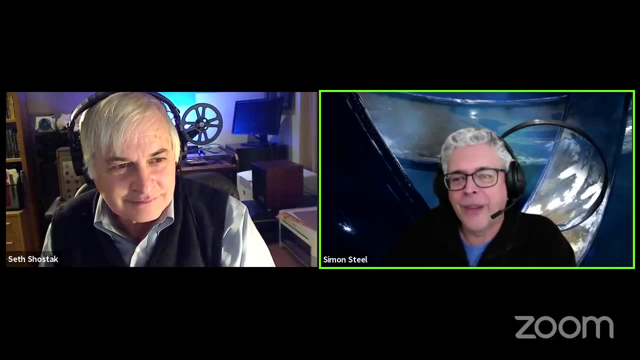 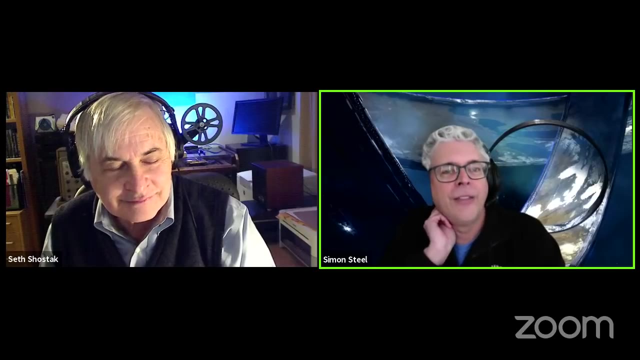 functioning happens from generous donations to viewers like you, to use a cliched expression. So thank you very much. It all helps. So we're not going to be able to send something set the size of North Dakota up into space for a little while. So that sounds as though we are by definition. 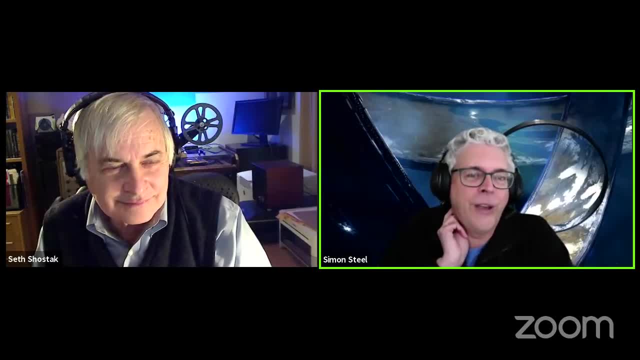 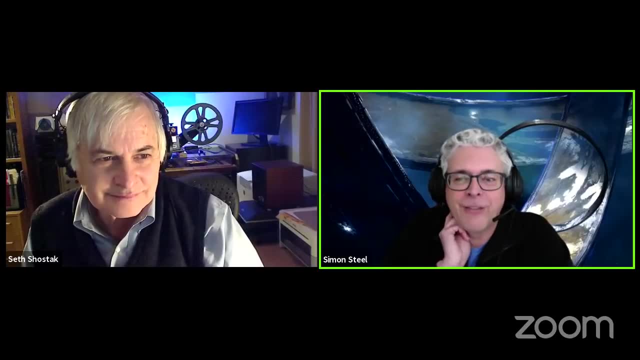 dealing with a more advanced civilization than we are And, as you say, it's difficult to know what other humans are thinking up, let alone an advanced civilization. There is a scale of civilizations, isn't there? It's called the Kardashev scale, And 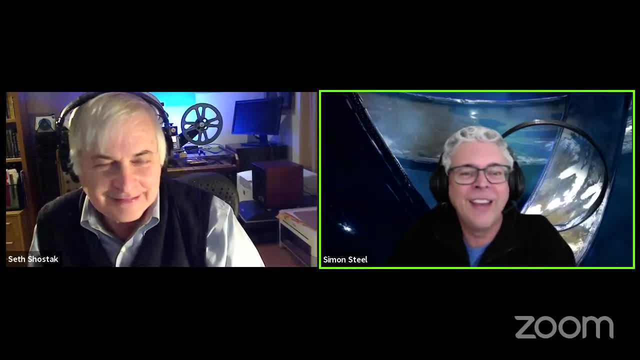 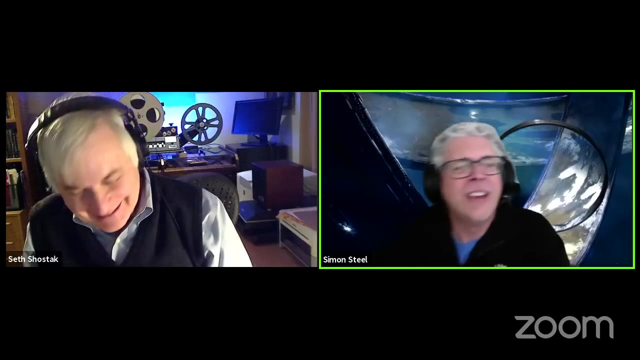 maybe you can say a little bit more about how you define the level of civilization, one, two and three of which the humans represent the sort of the lower tier, as it were. Can you say a little bit more about this sort of this distinction, or how you 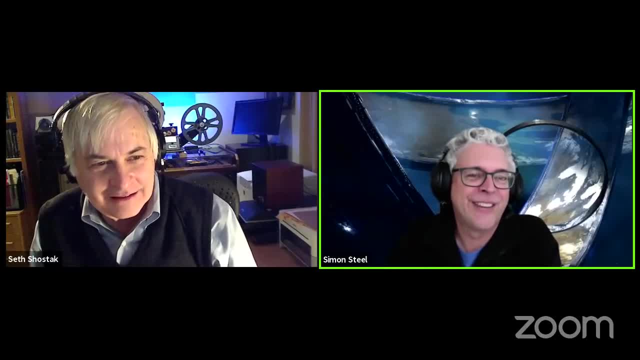 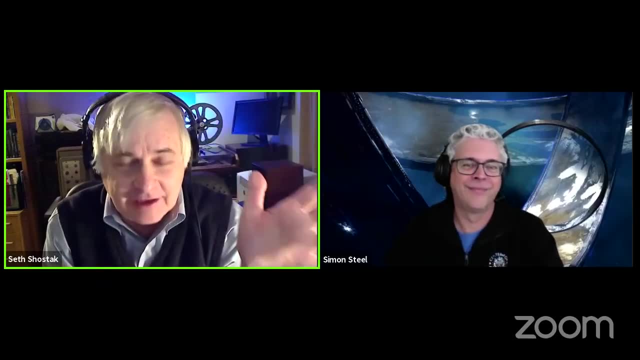 how you pigeonhole civilizations. Yes, the Kardashev scale which was actually- you can find it in his bathroom. The Kardashev scale actually was. you know, it was an invention of Nikolai Kardashev, who was this? well, I think he's. 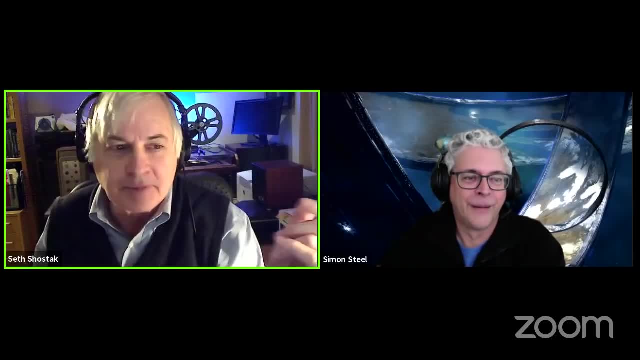 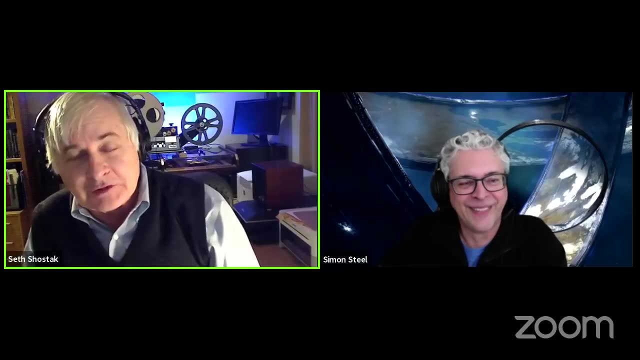 still alive. Maybe he's not. I better not say anything there, But we'll see. if he writes in, he might have something to say about that. You didn't mention Moscow and this is the people who look here. Yeah, you just said look basically there, must you could? 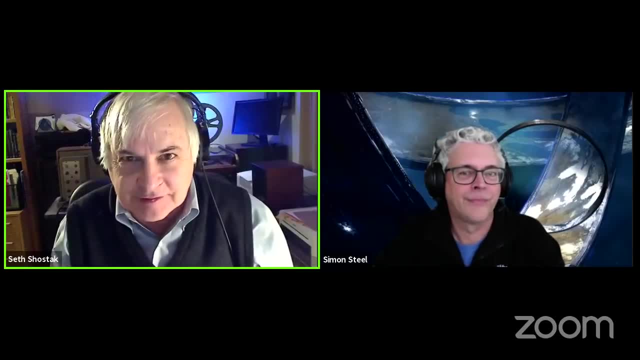 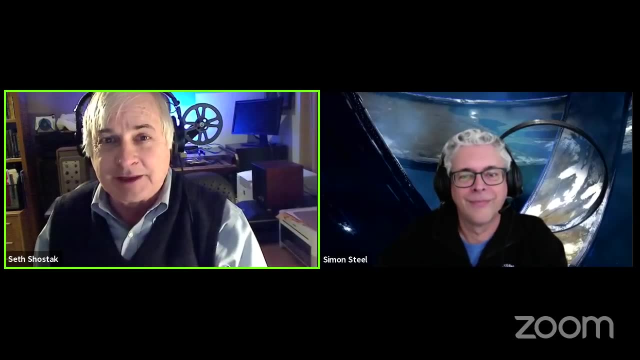 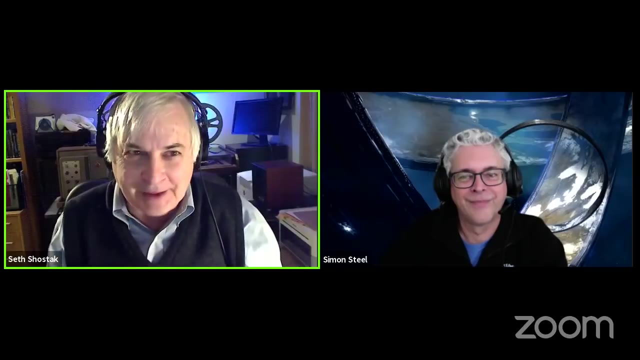 say there are three conceivable types of civilizations based on their energy use. right, So a type one civilization, the lowest of the low, uses the energy reserves of their own planet. Now think of humanity. you know we're using the energy reserves of our planet And you know whether that's the wind. 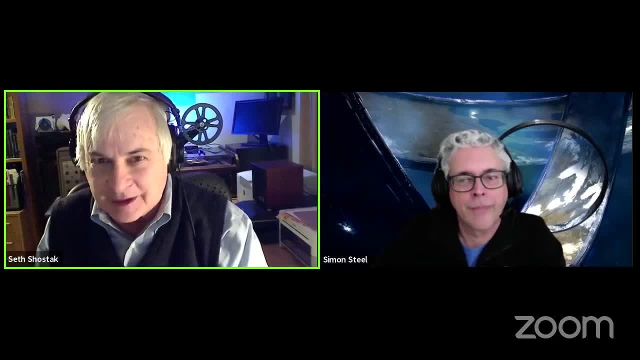 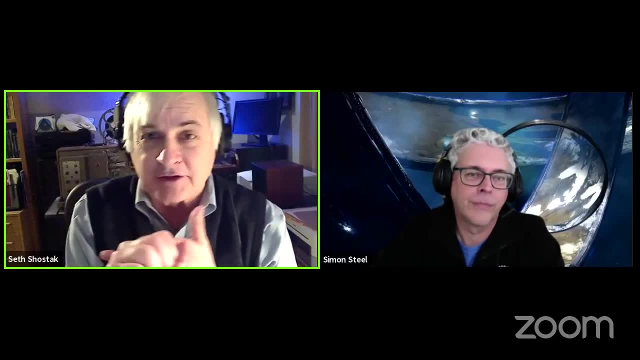 power, the solar power. well, solar power maybe not the energy of the planet, but certainly all fossil fuel use. That's the energy of your planet. Type two civilization uses the energy of its star. So if we build a giant swarm of solar 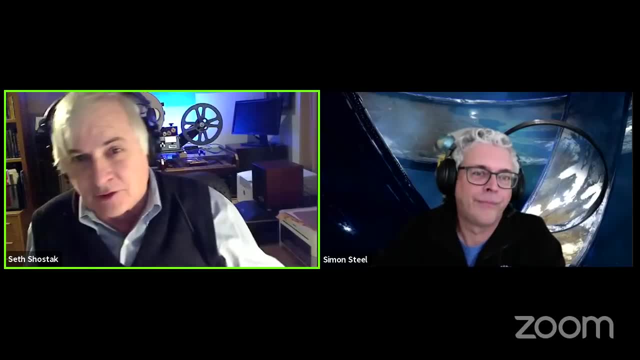 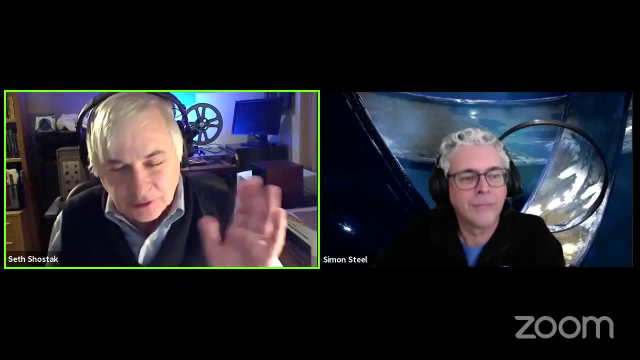 collectors, a kind of Dyson swarm, you know, out beyond the orbit of Earth to collect energy. well then we become a kind of a type two civilization where we're using much of the energy produced by the sun. a type three civilization uses the. 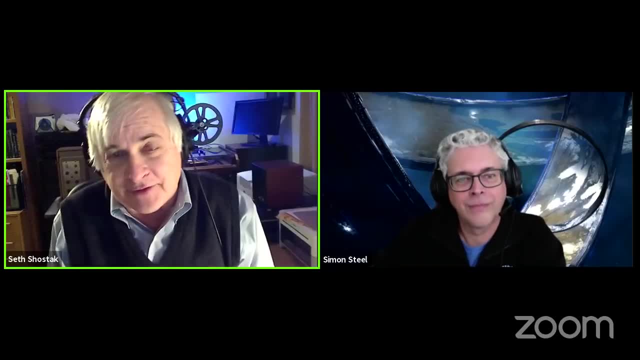 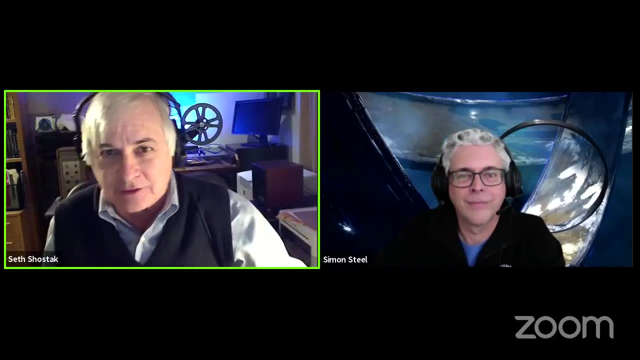 energy produced by its entire galaxy. Now look, the whole point about artifact searches is you forget about looking at the nearest other star system that might have a planet sort of like the Earth? That's, that's old thing. See, new thing is to say: look the. 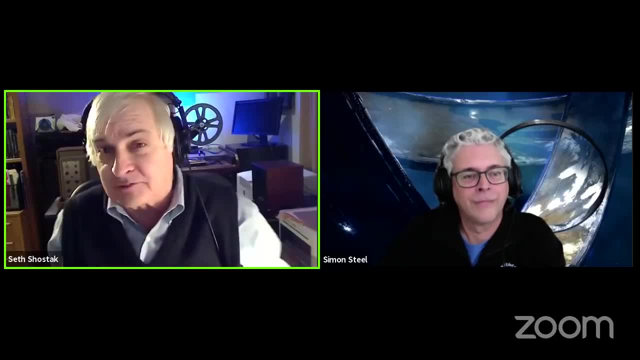 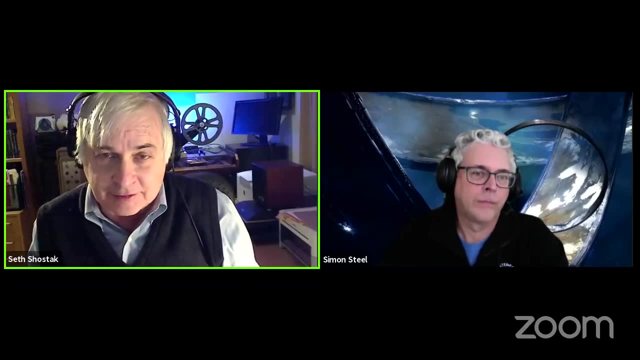 universe is very old: It's 13 billion years old. So there are some societies out there, presumably, that are incredibly farther along than we are from a technological perspective. right, Maybe 80%- 90% of them blow themselves up or get bored. 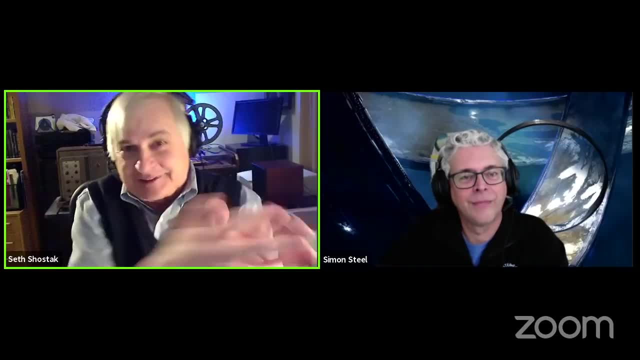 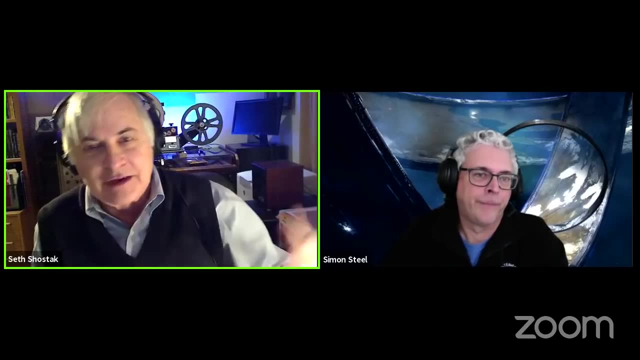 with television or for some reason go away, But that still leaves some. So the idea is, instead of trying to find a planet that's, you know, sort of like ours, maybe 100 years more advanced, maybe 1000 years more advanced, go look for the. 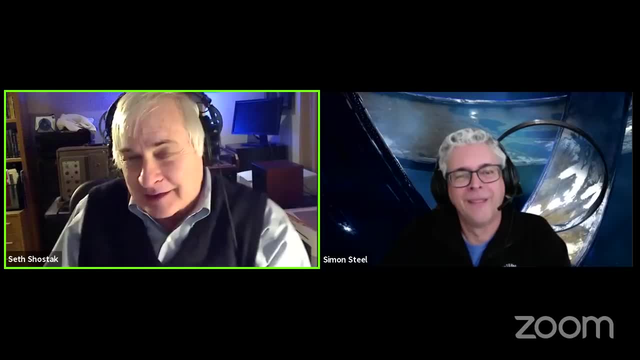 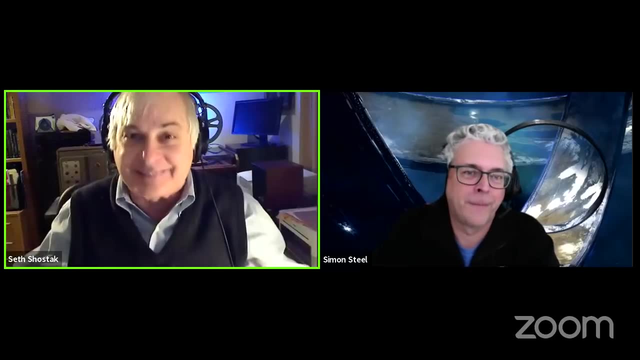 really old guys, right? That kind of leads me to a joke. So you go, look for the oldest civilizations. they may be building the biggest things, And you know that's another thing about artifacts. Yeah, there's a little bit of a time constraint, isn't there? I mean that human civilization is based on a 4 billion year old- 5 billion year old star. Yeah, that's a lot of evolution that's happened for 4 billion years. So so if you, there are a lot of stars are younger than. 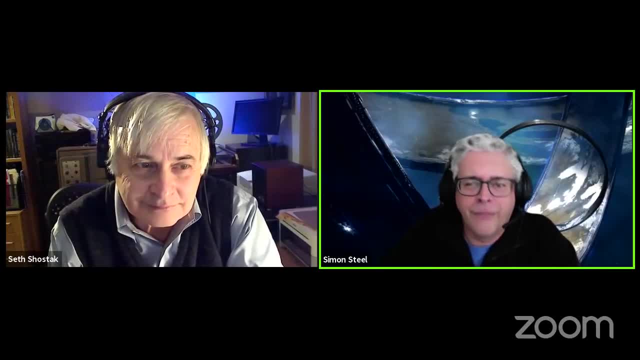 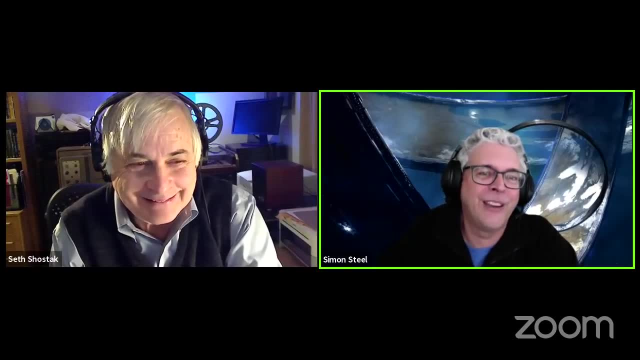 that. but there are a lot of stars older And a lot can happen in a million years of evolution, which is a very small part compared to 4 billion. So really you're thinking about targeting older stars. So you need to think about you know. look at the star system and figure out how old the star is. Do you think red dwarfs, which, which you know, tend to be a town for a very long time, Are they a good place to look? Well, I think so. I'm partial to red dwarfs, And it was also a 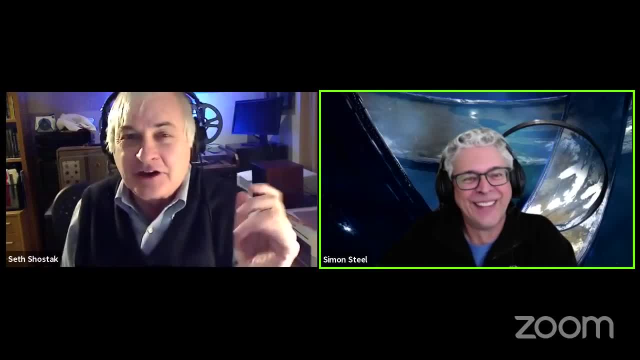 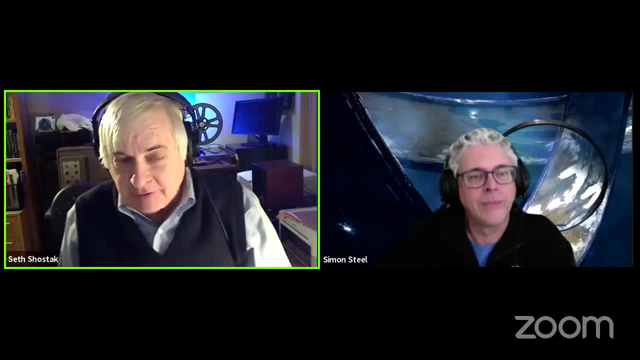 British TV show. It was Red dwarfs. you're right. Red dwarfs live for at least 10 times as long as a star like the sun will live. So every red dwarf that was ever born in our galaxy is still out there now enjoying. 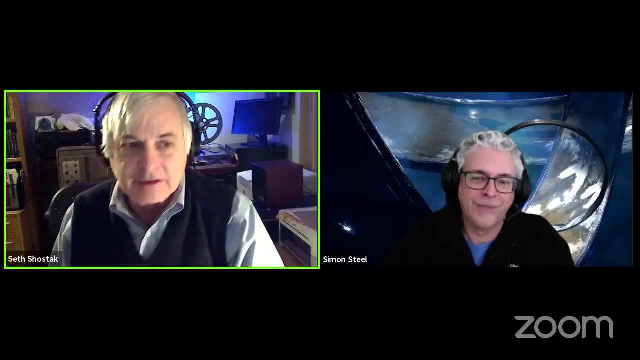 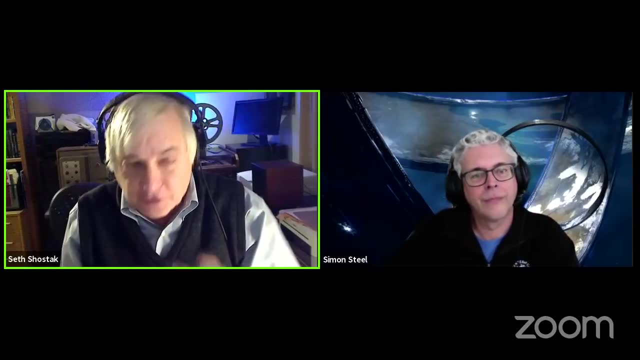 its youth. And as soon as the pandemic eases a bit, those stars will be able to go to the local bars and, you know, just enjoy life. So those stars have been around for such a long time And there's so many of them, right, Something like nine out. 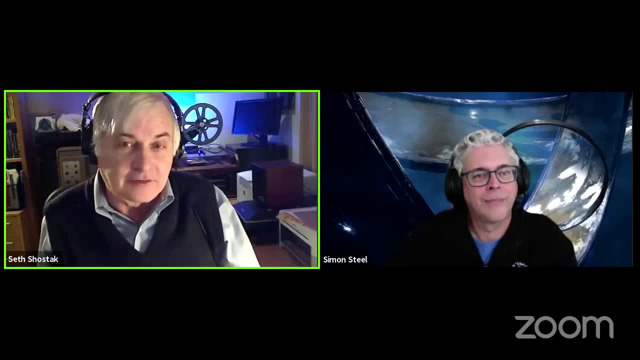 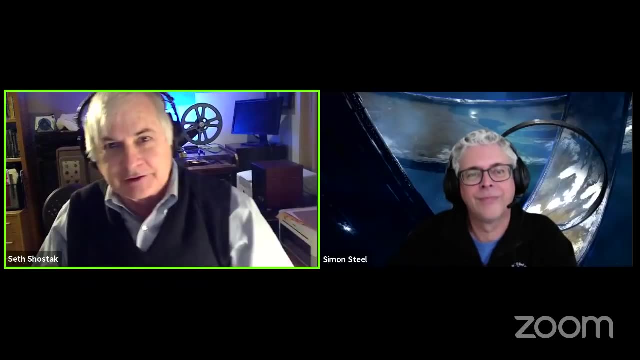 of 10 stars is a red dwarf? That may be. indeed, that's where ET is hanging out. Now you can say: I don't want to live around a red dwarf because it's so dim. right, It's trouble enough to live in a neighborhood with where everybody's kind of dim. 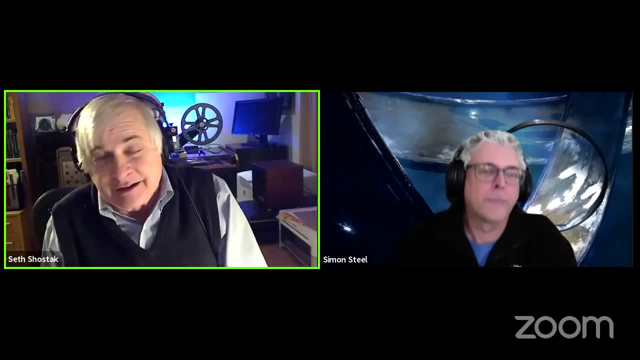 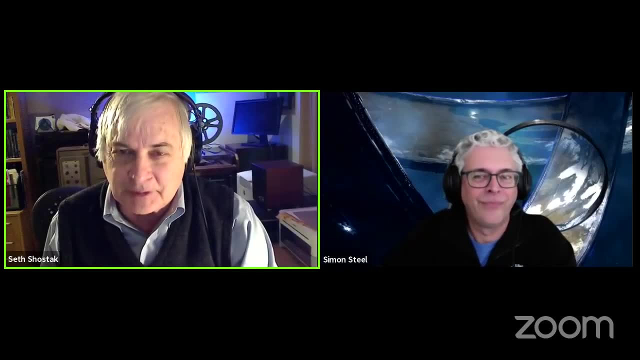 But to live around a red dwarf. you know you might think I'm not going to get enough energy to grow my crops and so forth And so on. Those are all very provincial concerns. You can do all that. They're still putting out energy. You can. 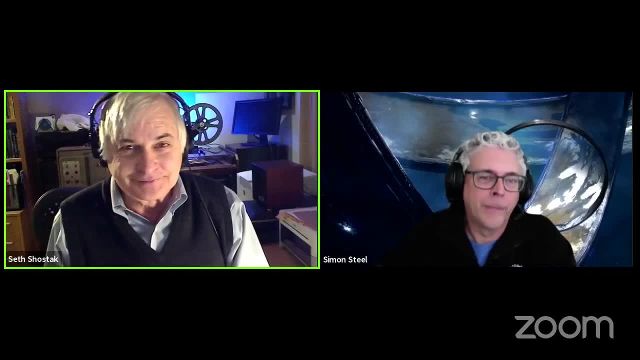 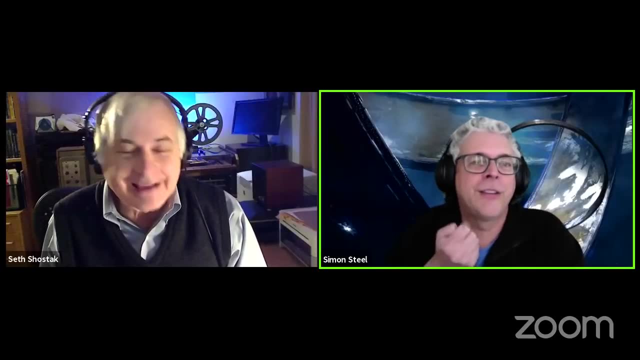 live around a red dwarf. So yeah, let's look around red dwarfs. Okay, Let's think maybe some more examples. We talked about Dyson Spheres. I've got a ring world behind me in this illustration that I nabbed from the web, So unfortunately I can't offer to. 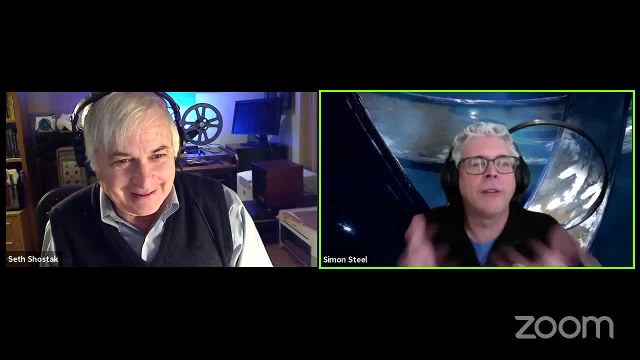 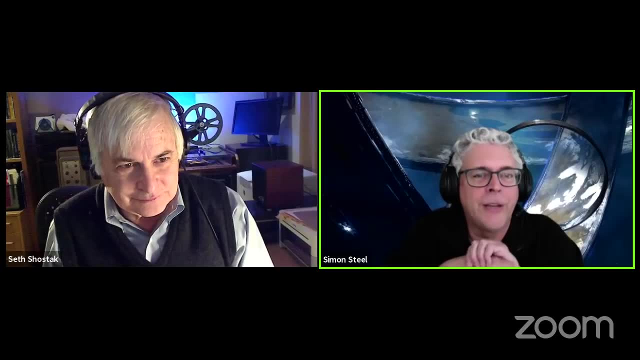 sell it to people because it's somebody else's. But what other examples have you got that of, say, a Type II civilizations, one that can build Dyson Spheres, or even Type I's? What other things could we potentially be looking for? 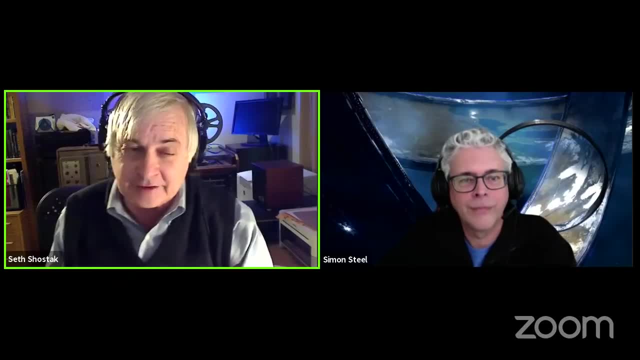 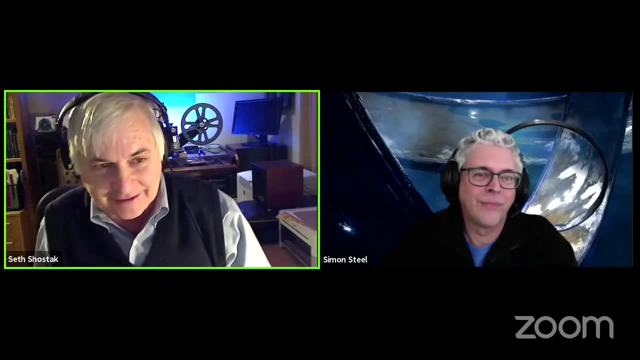 Yeah, well, it's hard. You've already mentioned this, Simon. I'm not trying to duck the question, But it is hard Because if you would ask this, if we were having this discussion 110 years ago, say in 1900, right, people were talking about the canals on. 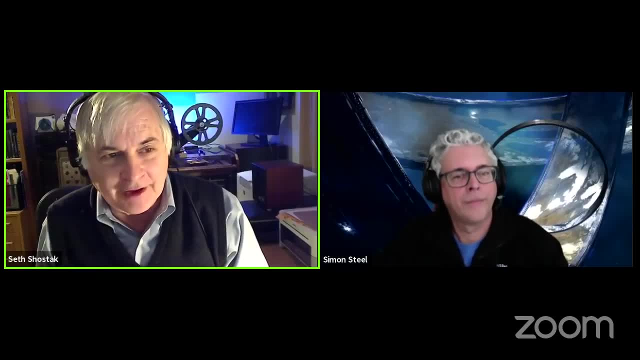 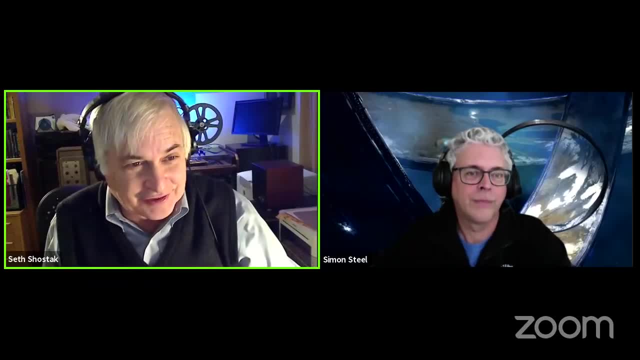 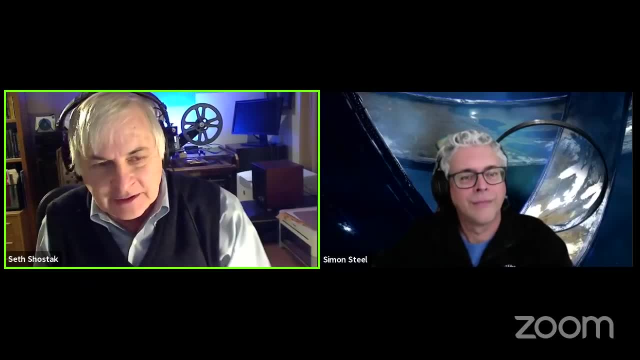 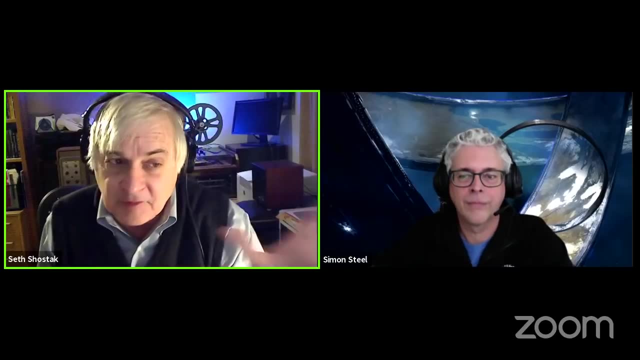 the idea of being able to predict what really advanced societies would do is quite difficult. But you know, the Dyson Spheres is certainly one possibility, Dyson Swarms, whatever these very big structures to collect a lot of energy. Now there's a fellow here. 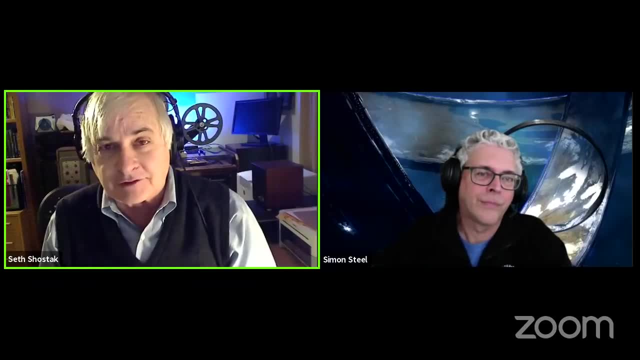 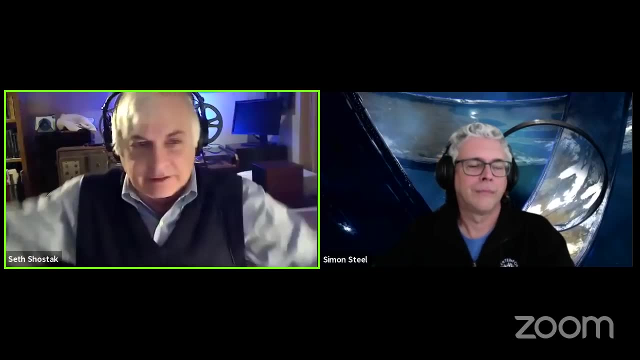 in the Bay Area by the name of Gerald Nordly, who also writes science fiction. He's a very clever guy And he gave a talk, two years ago I think, in which he pointed out, if you did build a Dyson Swarm or Dyson sphere, not only would you have all the energy you could possibly eat. I mean, that's a lot of energy you could collect with something like that, But you'd also have a really big baseline. In other words, it's a long way from the. you know one side of the Dyson. 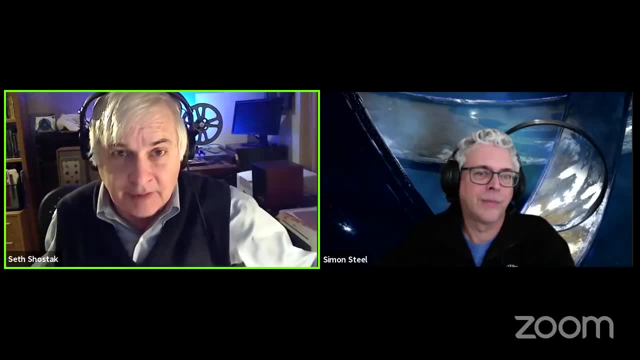 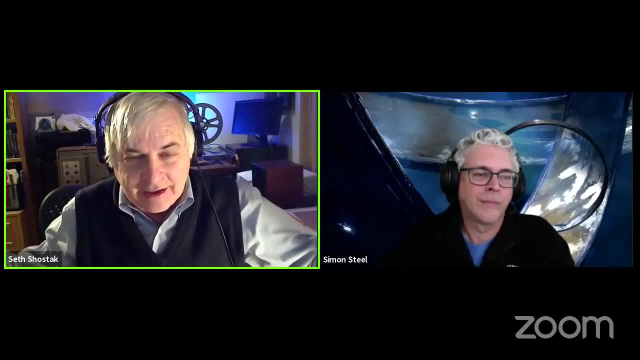 sphere to the other right it might be a couple 100 million miles. That's the dimensions of these things. So you have all this energy and you have all this real estate, And that means you could build transmitters to convert that energy into whatever. 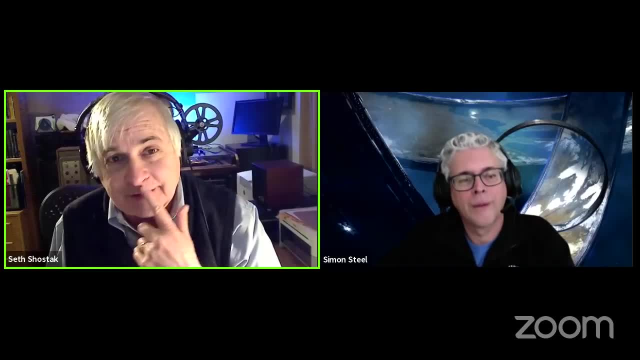 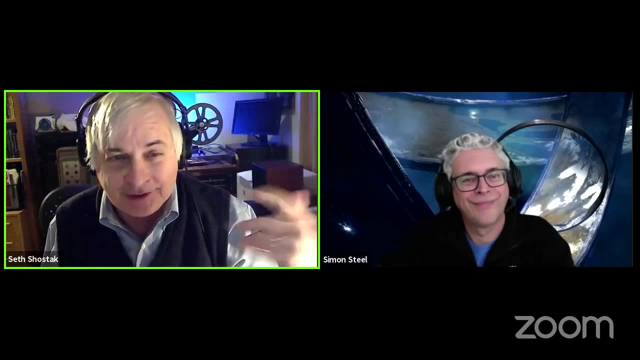 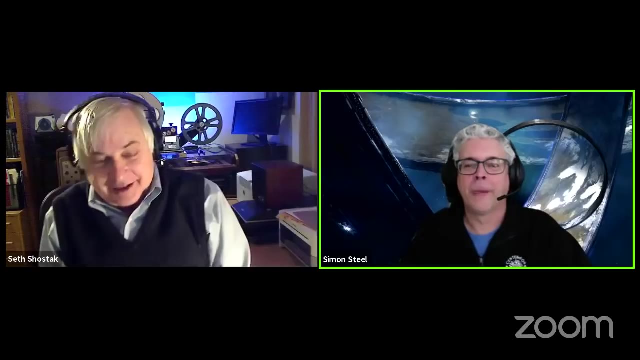 microwaves, infrared something, And you could easily take out you know a planet hundreds of light years away if that was on your agenda. So he was suggesting that actually Dyson spheres are probably illegal. Yeah, I just got to ask one more question, then we'll go to a lot. 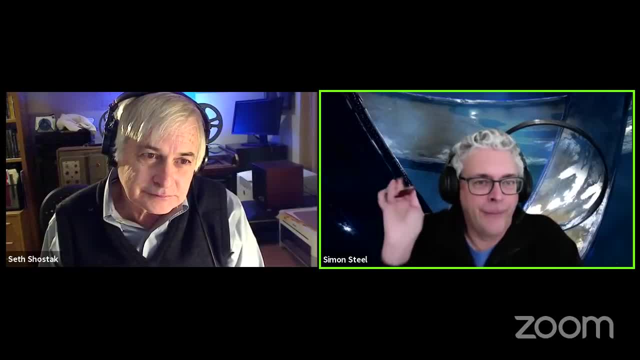 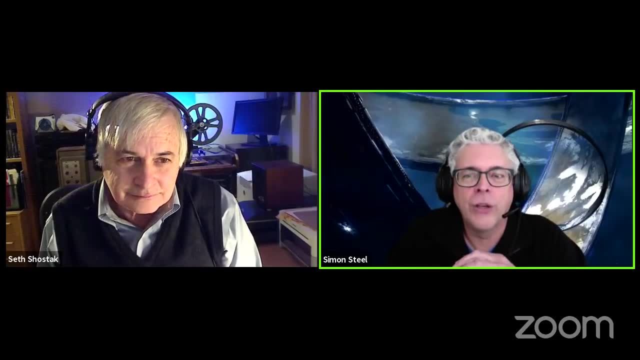 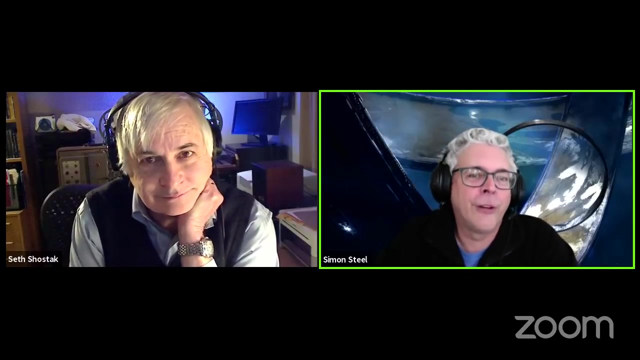 of questions coming in. Dyson spheres, stellar disks or rings- these are all constructions that would result in an unplanned detection. nobody's going to build a Dyson sphere to be recognized. If you wanted to have a deliberate, we are here. moment for an advanced alien civilization. what sort of 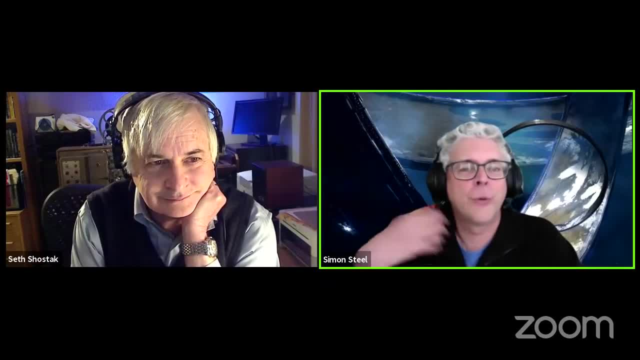 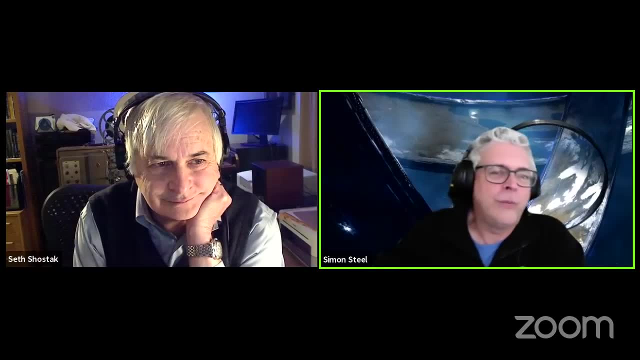 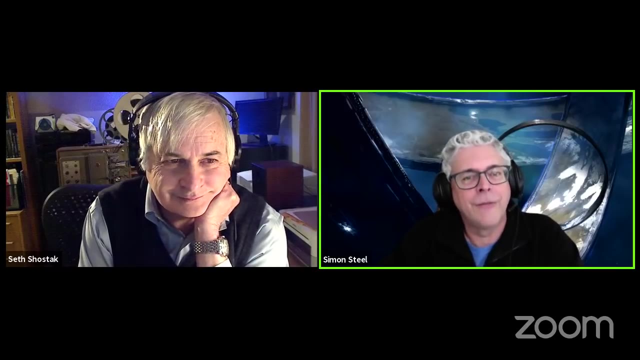 thing again. we're projecting 21st century human brains into what an advanced civilization would do. You know what would? what do you think we would be looking for? something that would be deliberately recognizable, that, you know, maybe is passive? Yeah, well, if you want something that will forever mark your existence. 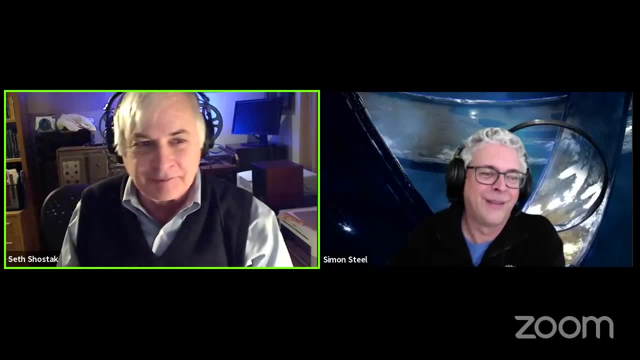 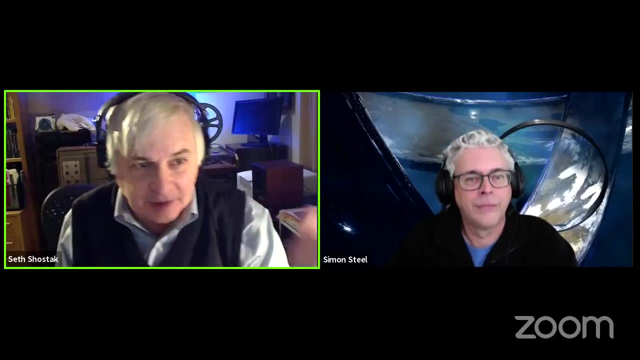 like a tombstone. I mean, that sounds a little lugubrious, but you know what I mean And all you want to do is tell whoever is out there. somebody is here. This is a monument. It's like a cairn, right, You know, stack of stones. Somebody was here in this part of Antarctica. 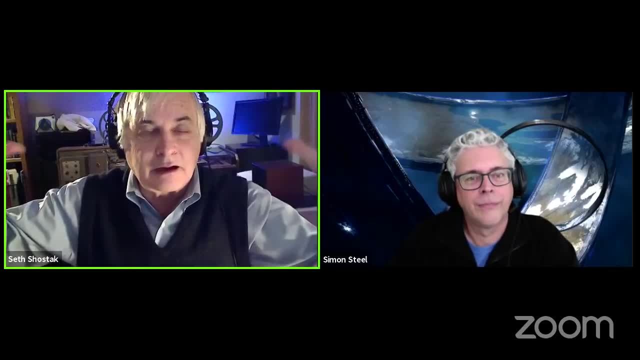 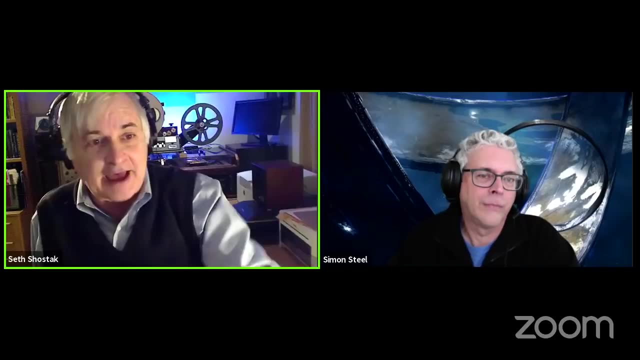 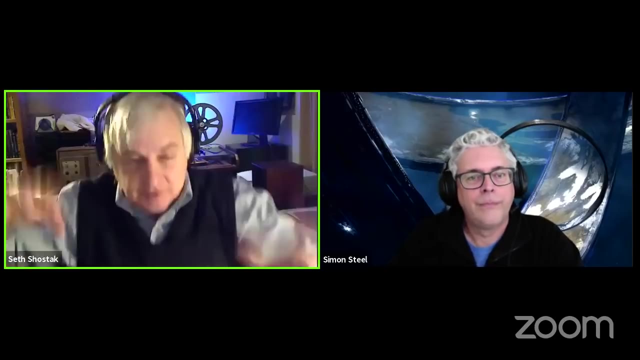 You could just build a big, obscure. you know it, just a big sheet of metal, very thin metal, so you could eventually construct it in space and have it orbit your own star and then have another one orbiting in the other direction, And anybody looking at the sun would suddenly see it get very 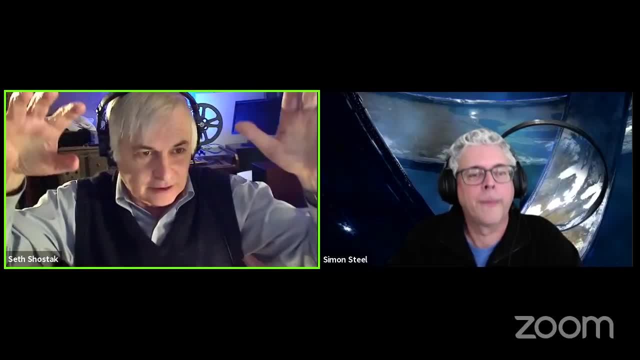 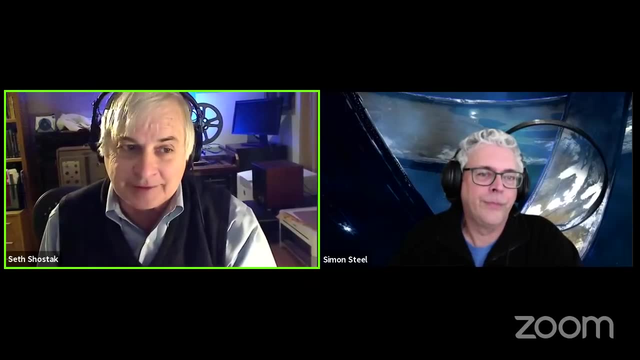 much dimmer and then go back up and then get dimmer And then, you know, brighten again, on a very regular basis And with some very simple geometry, you could convince yourself. this is not a planet doing this. This is something else. 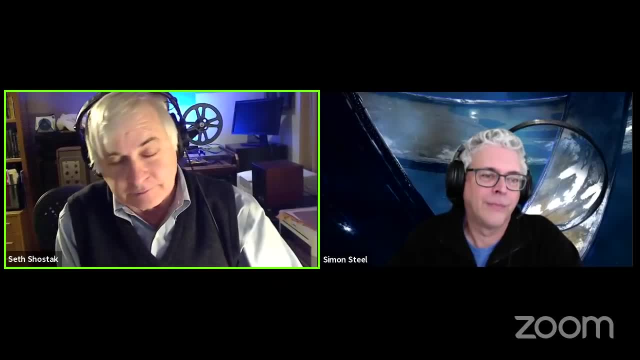 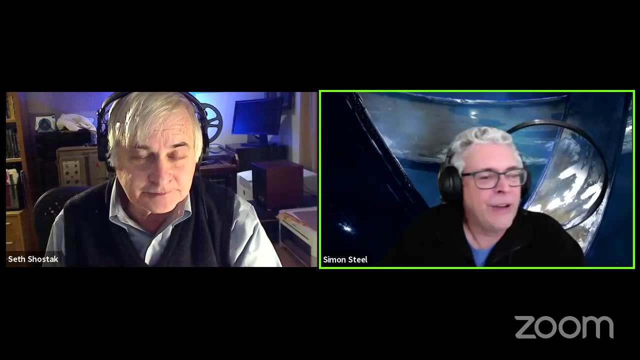 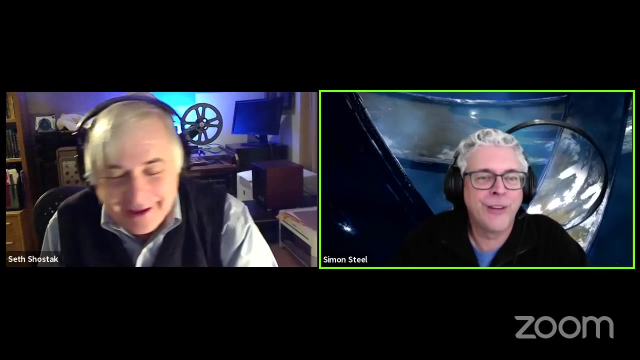 And so that would mark your stellar system if you, you know, do that and are not afraid of the Klingons. Okay, we're going to turn our attention to some of the questions that are coming in. We also have another donation, Massimo. thank you so much for your donation. 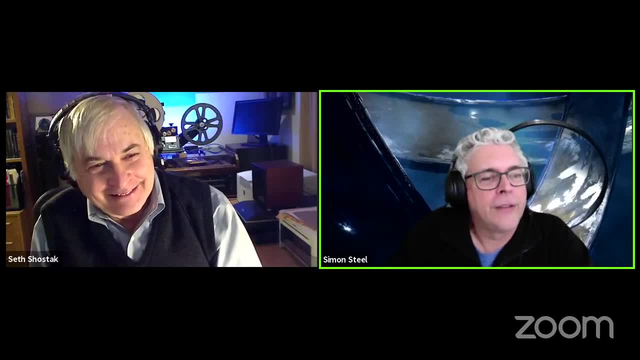 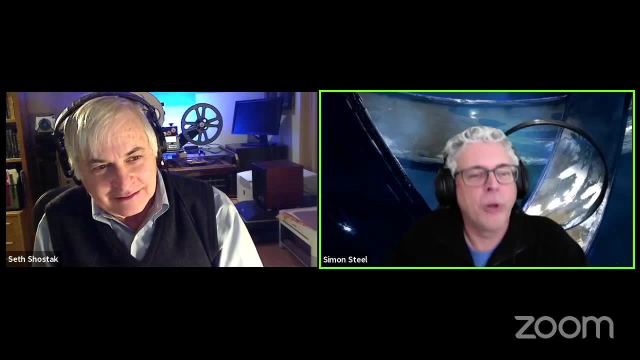 Now this is a question actually close to home. This is something I was interested in. You know, if a robotic system or an alien system is going to be a robot, would you be able to produce a robot? civilization passed through. would they leave something behind? We've all seen 2001.. There's 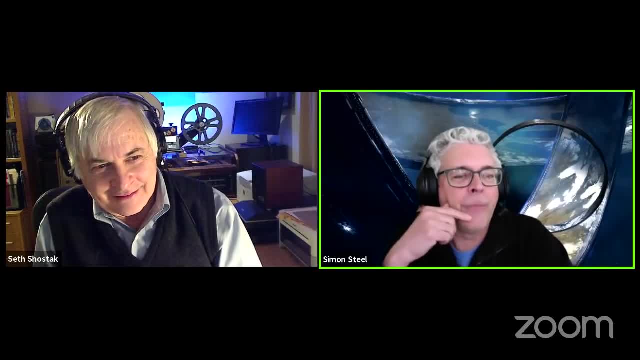 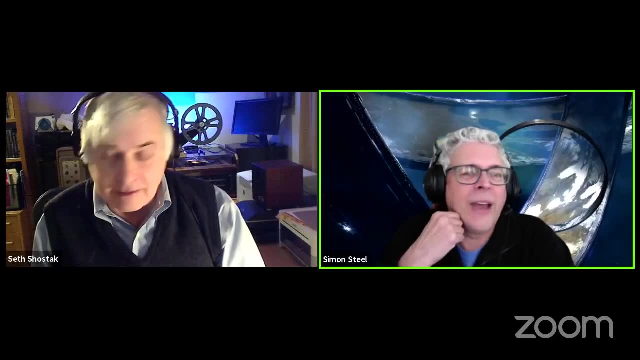 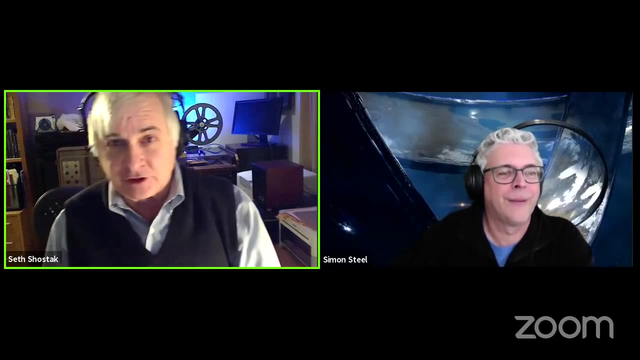 a good thing to stick on the moon, And one of the questions is: how difficult or expensive would it be to do a search for artifacts on the lunar surface, And how would you even go about knowing if something was an artifact or natural? Well, once again, this sounds like a Stanley Kubrick. 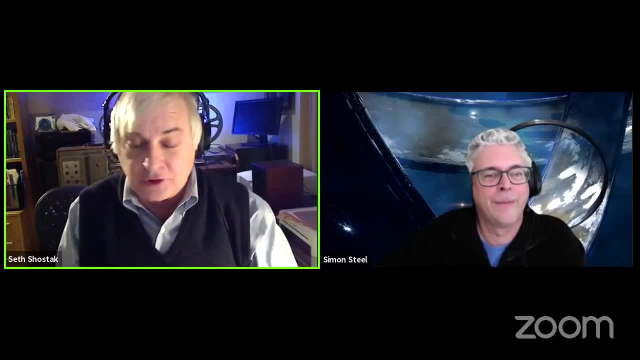 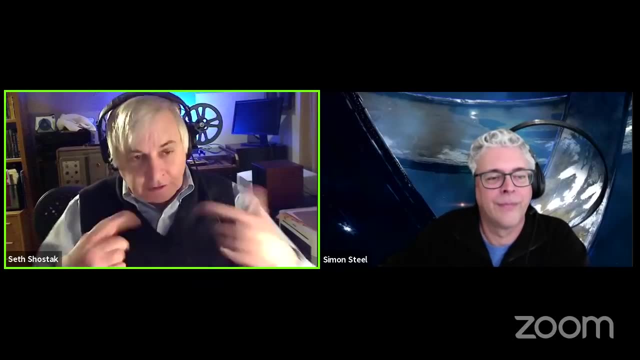 movie. But in fact I mean, you know, you could say that the moon is better mapped than you know the sub or the bottom of the oceans here on planet Earth, because we do have orbiters orbiting the moon and they do make photos And I forgot the best resolution, In other words, how much detail? 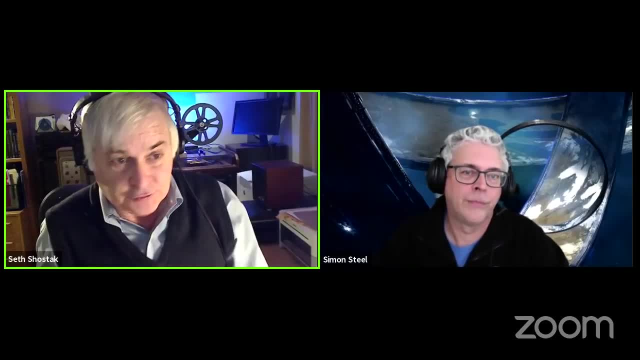 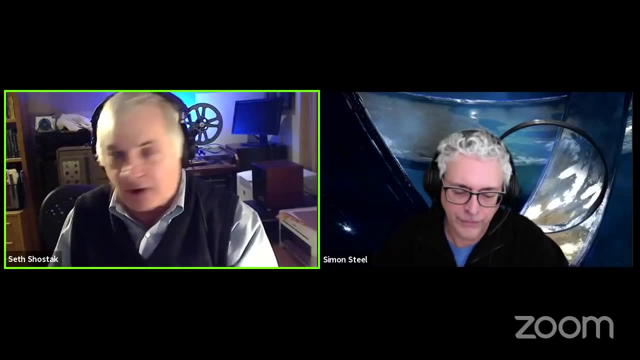 can they see? but they could see something the size of a small house for sure, And maybe you know the size of a school bus. you have to look it up So you could say, all right, there are all these images. Well, who's going to sit there and look at the moon? And I think that's a good thing. 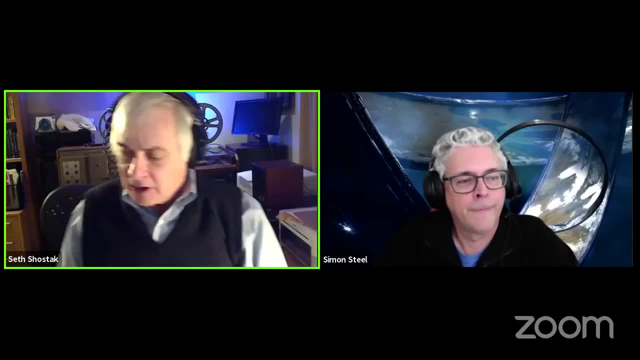 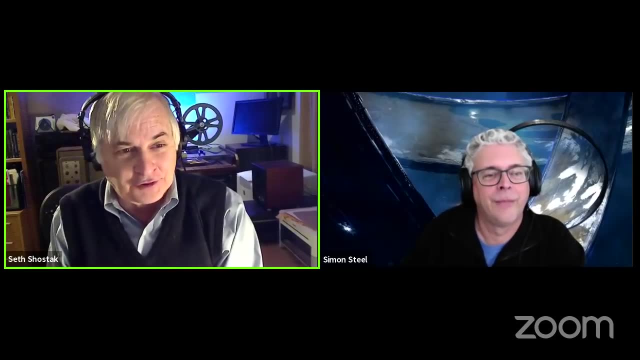 Look at these tens, hundreds of thousands of detailed photos of the moon and say, oh, look at that, You could make it a citizen science project. People are forever looking at the photos made by the rovers on Mars, looking for signs of life. But you could do it that way. But today you would. 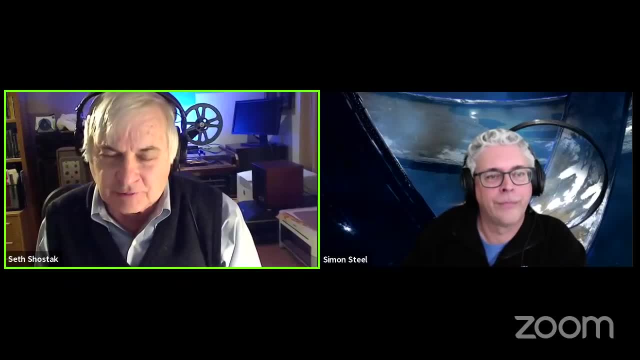 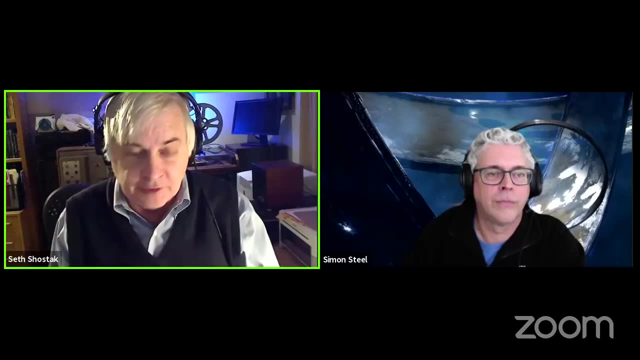 just have you know, artificial intelligence, machine learning, really- and just scan all these things And I'm sure 10 years, 20 years from now we'll have orbiters around the moon that'll be able to see something on the scale of what you can see with Google. 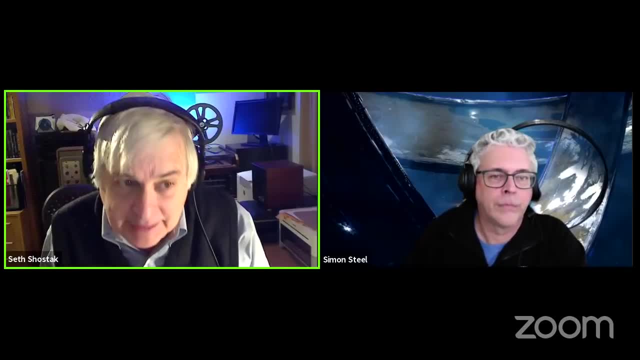 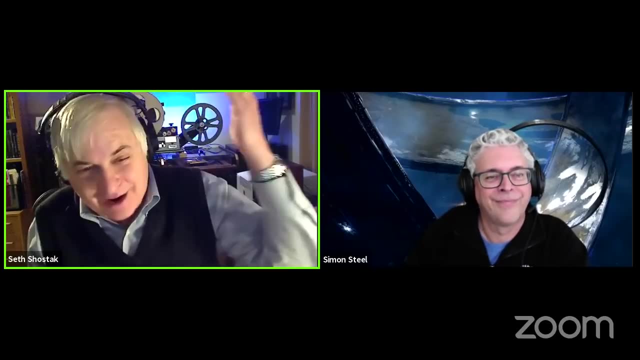 So if there's anything that's that big and that is recently enough, put there so that the rain of micrometeors hasn't wiped it out, then maybe we'll find it. If you think the aliens have been to the moon, 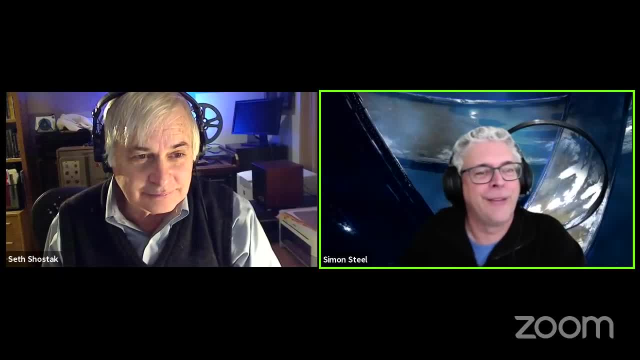 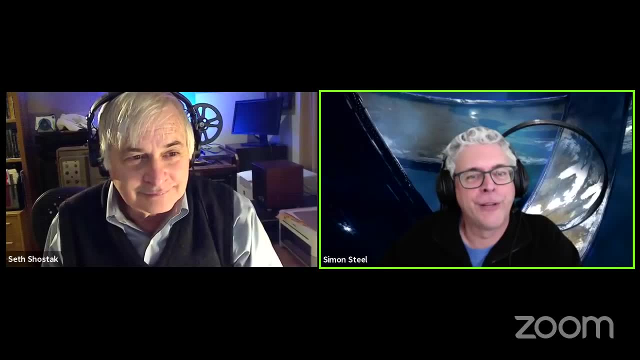 Maybe Utah, I don't know if you want to comment. There's a question about the monolith that somebody's found in Utah just now. Maybe the same people who did the crop circles in Wiltshire, I don't know. But well, maybe we don't even want to go there. 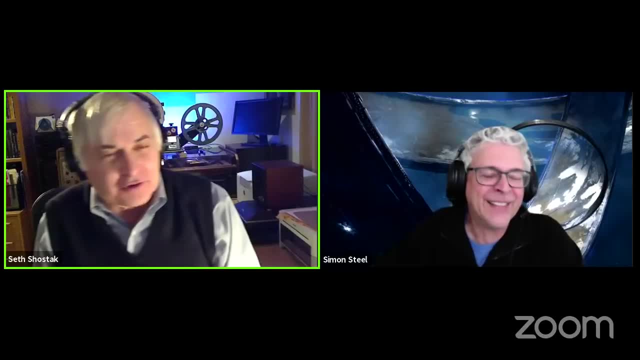 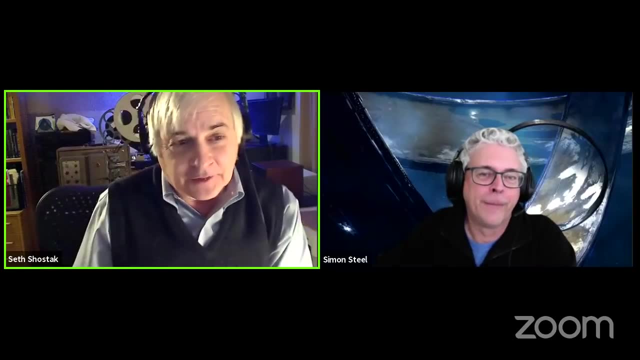 What Wiltshire? Yeah, you know, Southern Crop Circles are either in Wiltshire or Hampshire, But the rest of the UK but somehow, yeah, well. well, this model in Utah. it may be that somebody is expecting a whole bunch of. 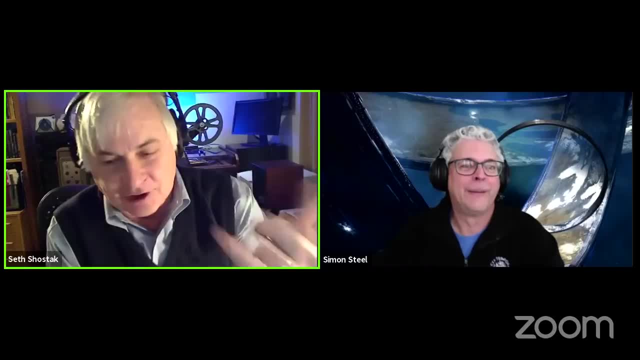 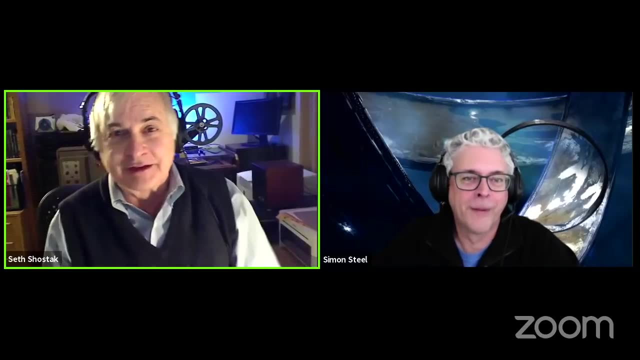 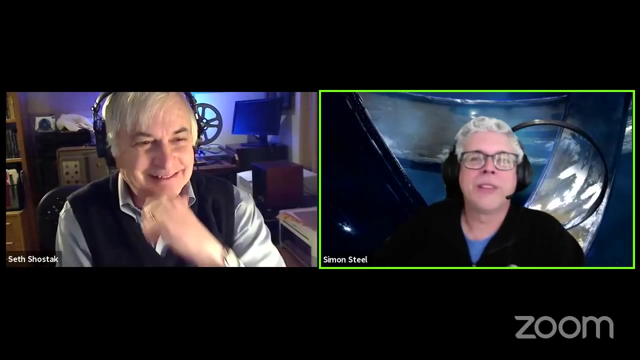 primates to go to Utah and you know sort of rally around this thing. I figured it was a Wi Fi hotspot for the aliens, But I think that your assumption is probably the correct one, Simon, that this is a bit of art, yes, very imaginative. there was a uh coming close to her. there was uh not that close. 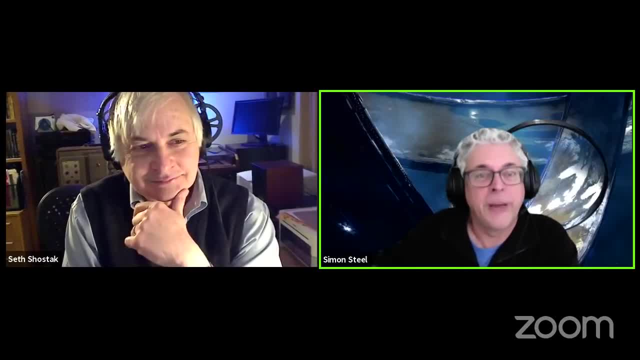 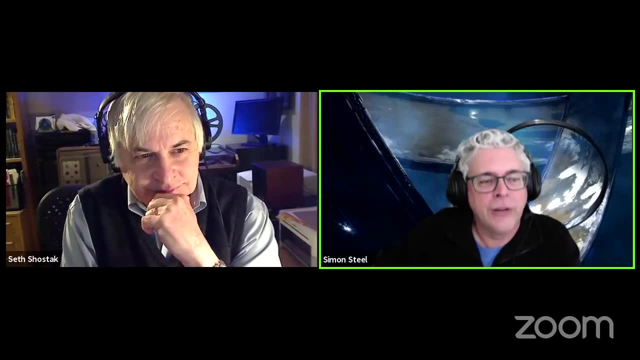 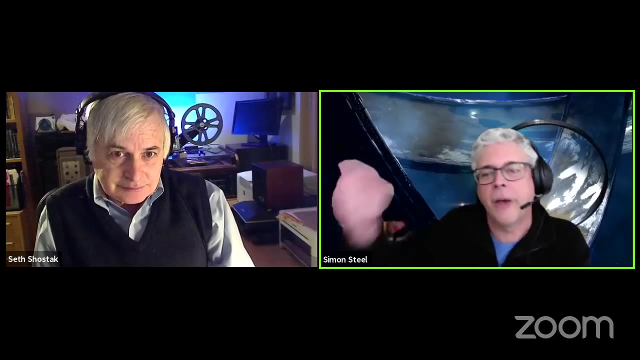 but, um, there was a, an interstellar visitor. there's been a couple now, where the first one was called umur umur, which which, uh, had had the impression, you know it's- it was probably an asteroid, um, that had been flung out of another star system. um, it passed by, you know, the, the earth, and and or passed. 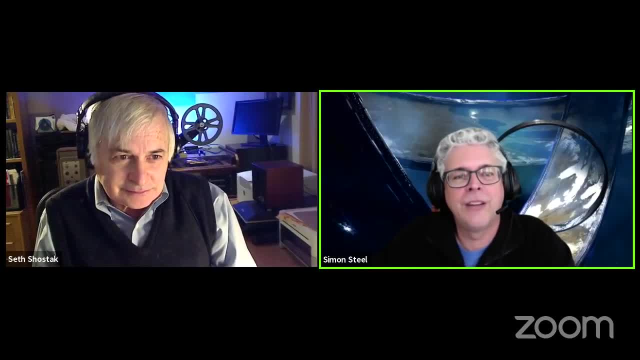 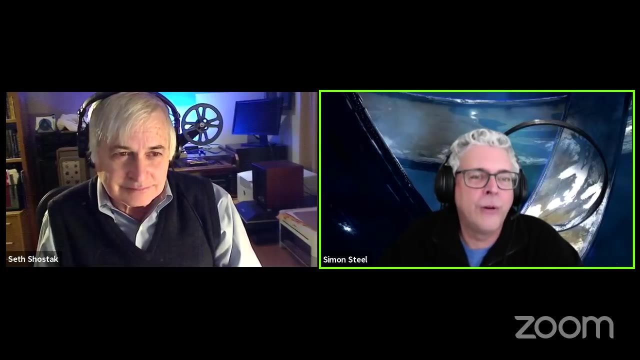 by the solar system and flew out again. i know it was studied in reasonable detail and, uh, i- i believe that green bank did- did an analysis to see if it was transmitting. um, so you know that there are possibilities. i suppose, uh, we don't know what what alien civilizations are doing or how they're. 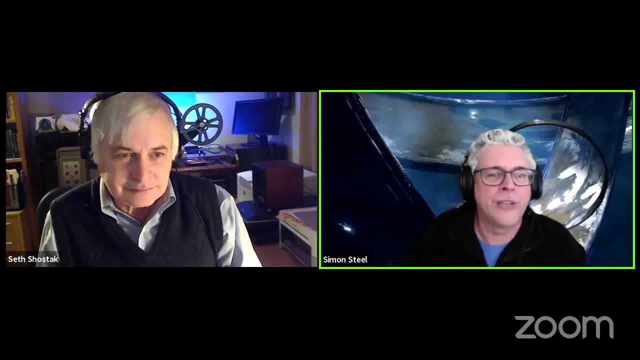 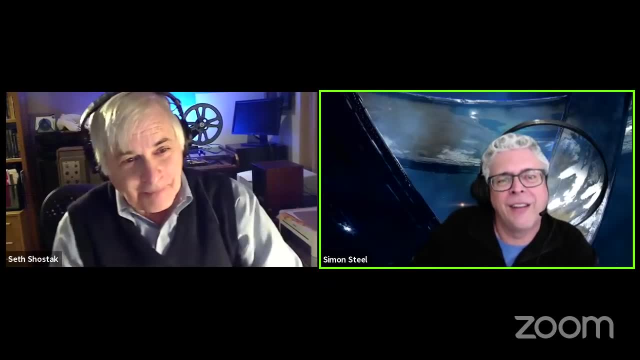 influencing, um, or want to, you know, influence us, or make themselves apparent. um, so a little bit about umur, umur, what, what's, what's your feeling on, on that? and- and that is a technique to to come and visit in a sort of stealthy way- 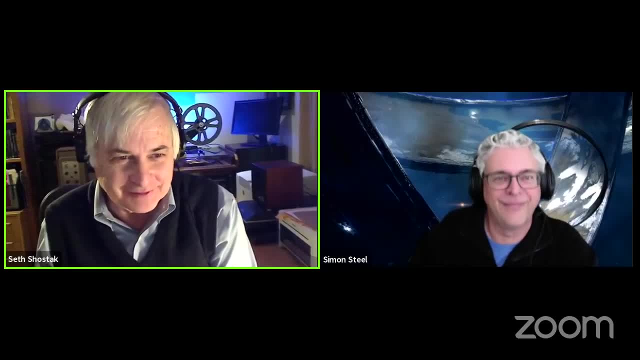 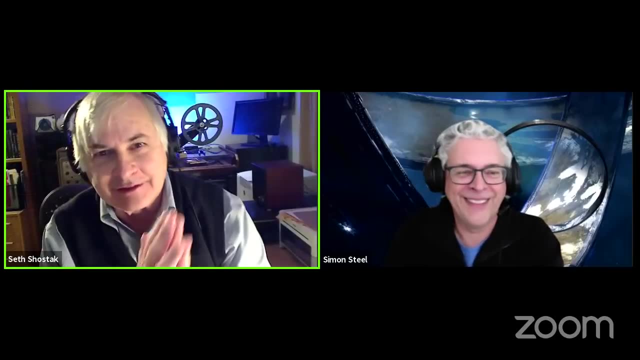 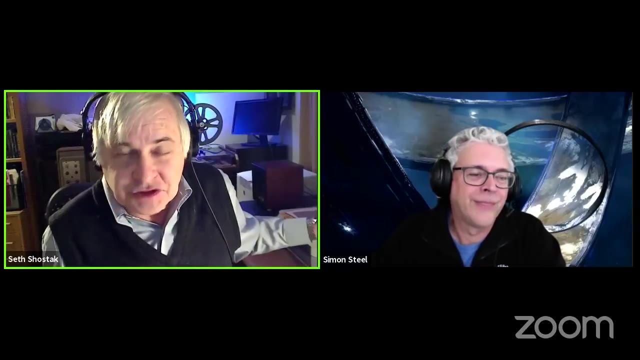 yeah, i think arthur c clark wrote a story, right whatever with rama. yes, yes, it's a good book. yeah, they all. after a while it's just. but indeed the aliens might have hollowed out an asteroid, put a an engine on the back and used it. 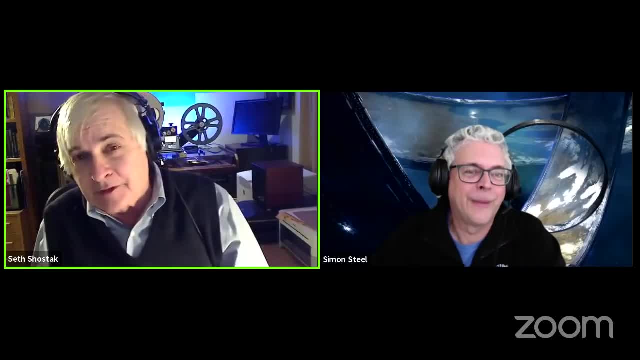 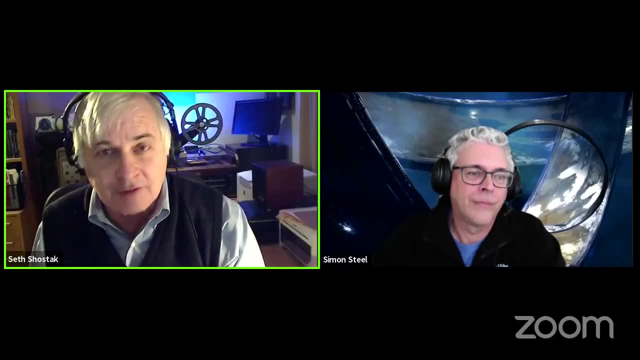 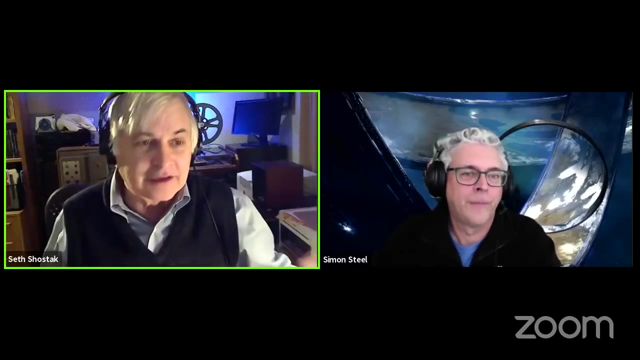 as a a vehicle to come visit our solar system. now the problem with the mua mua who, by the way, that idea was seriously suggested by the well, the chair of the harvard astronomy department, abby lope, and he pointed out that unless there are a lot of these things, you can say it's in an interstellar. 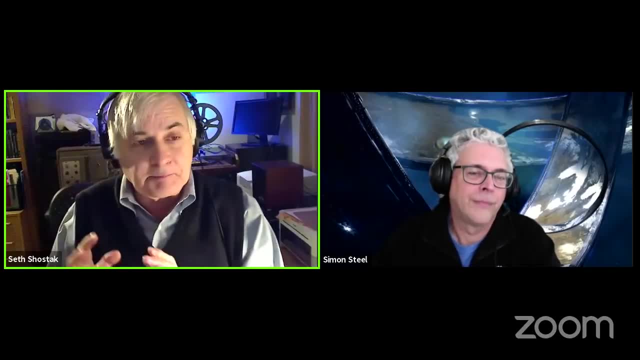 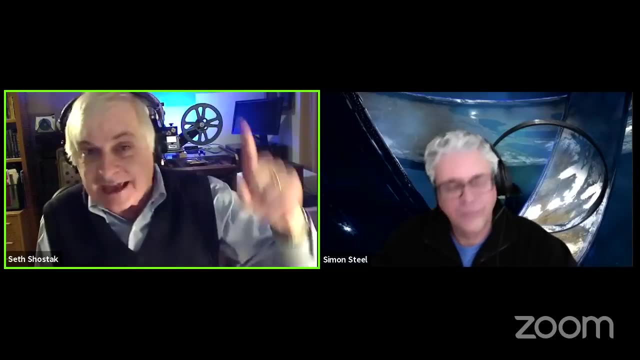 asteroid because it came from outside our solar system. but unless you assume they're just lots and lots of them, you can't argue that, yeah, this is just an interstellar asteroid that, just by chance, absolutely happened to zip through our solar system, you know, coming right into the nearly the center of the. 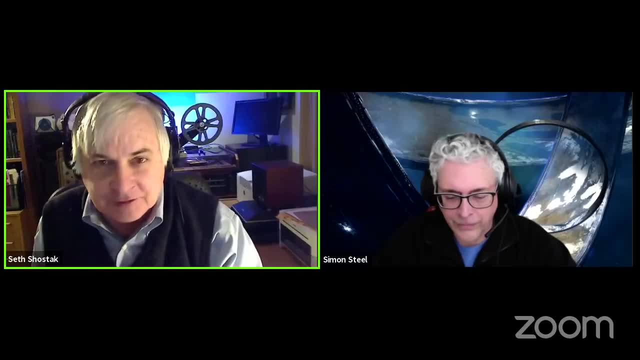 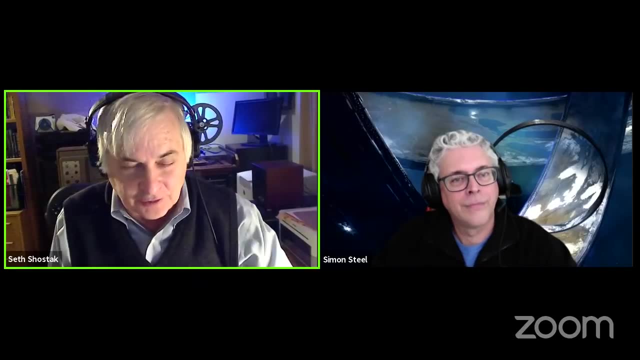 solar system, the sun, and then on its way out. i mean, that's terrific, targeting for a random process. but it turns out that another one was found a year and a half later, so probably it wasn't asteroid. but this thing was so far away we never saw it as anything more than a dot. 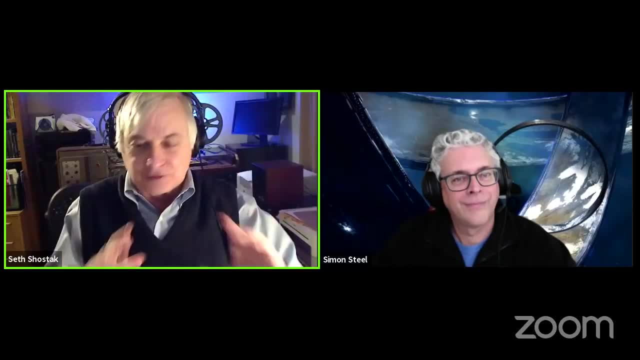 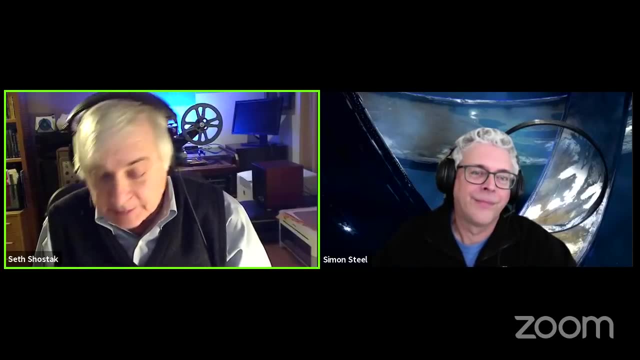 and some people say, well, why don't we launch a rocket? go look at it up close. maybe you'll see portals with little green faces behind them, maybe. but we didn't have the rocket tech technology to do that. but if you know in advance, you know if you have more warning for the next one. 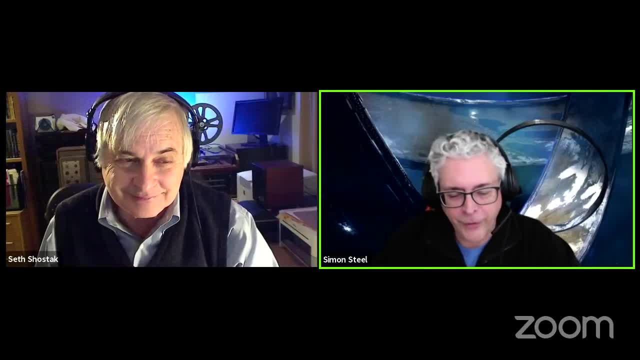 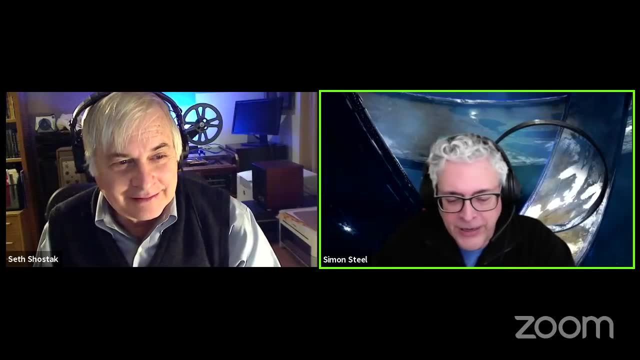 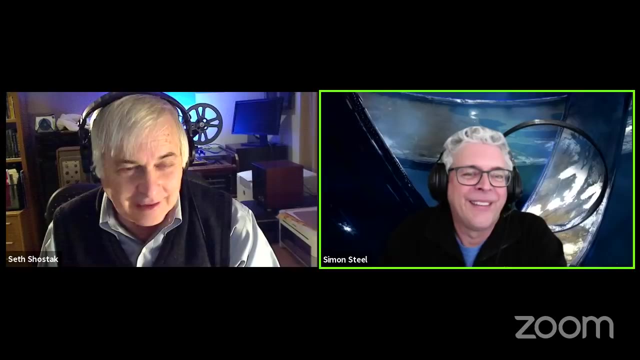 then maybe we will do that. yeah, i have a question here from from a writing question from tara in woking: um, could aliens communicate with us by sending comets and asteroids to earth? um, how? how would we look for clues? uh, much closer to home. yeah, well it's, it's the same problem if 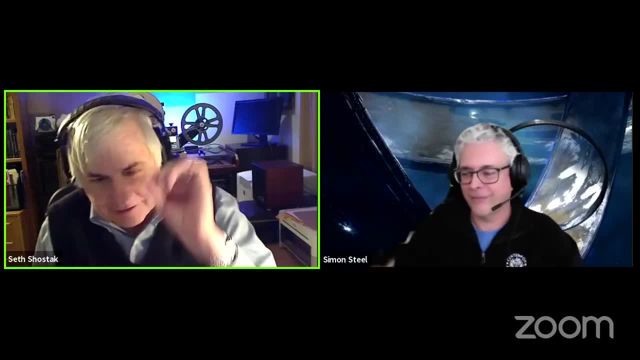 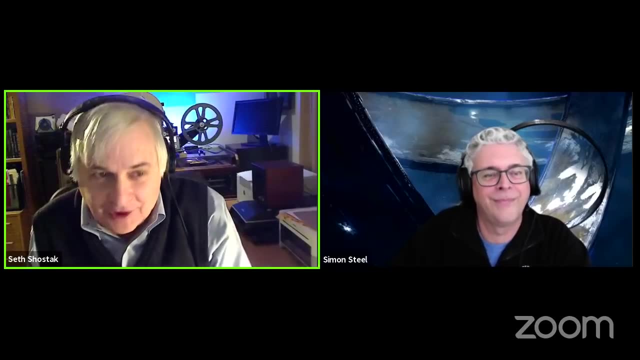 it's close enough that you can actually get a good picture of it, say a mool mool- it was always a dot. you everybody saw that artist's impression looks like a kind of a bumpy cigar. but that was an artist's impression, that wasn't a real photo. but if it's close enough, tara, then you could, of course. 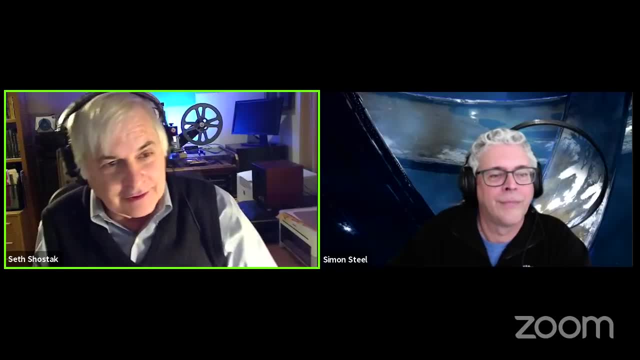 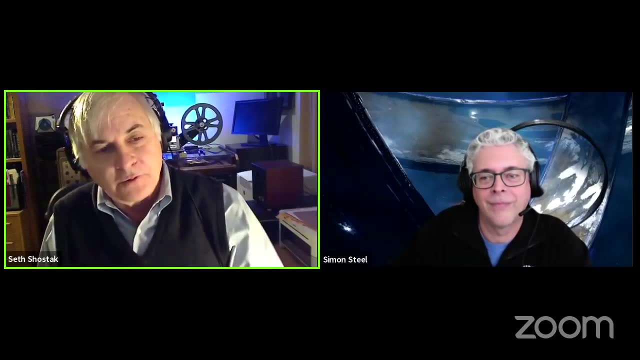 see, but there are other things. if it's, you know, got a bit of a tail or develops a tail when it gets near the sun, they can say, okay, it's probably a comet, and so what? we probably could recognize the colors. that's another thing. we could probably recognize whether it's an asteroid or a comet. 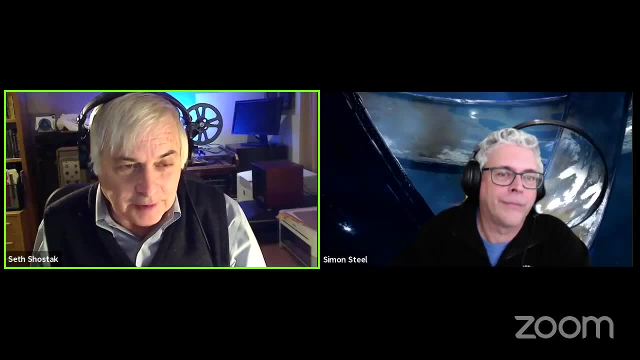 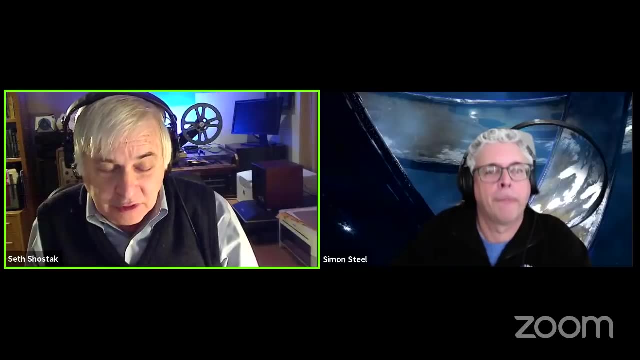 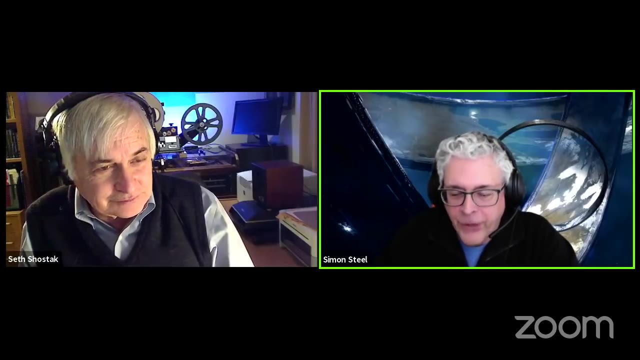 as a method of communication. i don't know. i mean you could do it, but why you might as well build a rocket right. the rockets don't have all that stone you have to carry around. and, of course, what's interesting is, uh, the um osiris-rex mission um is returning a piece. 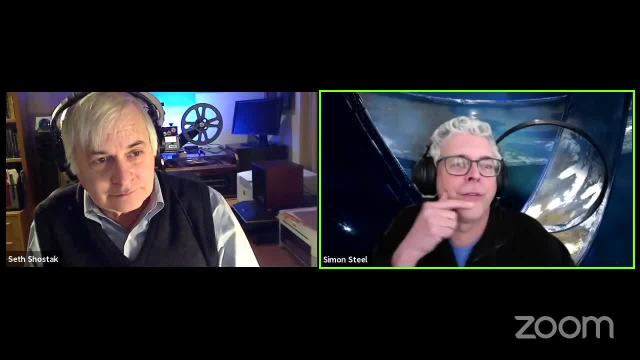 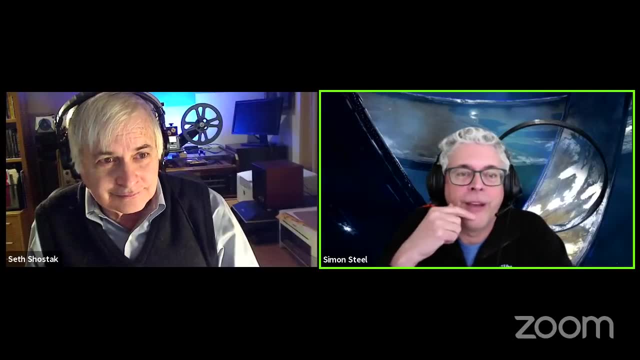 of cometary material, a piece of asteroid material, rather from from, from uh benu, and that will be in a couple of years time, um, and so we'll have a better idea of what's what uh asteroids are made of by sampling that material. uh, in a sense, i know this is uh, you know the various 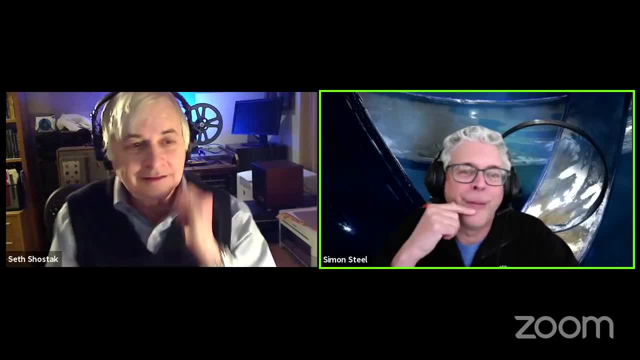 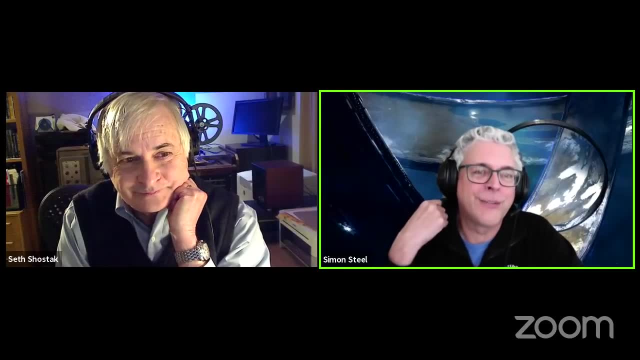 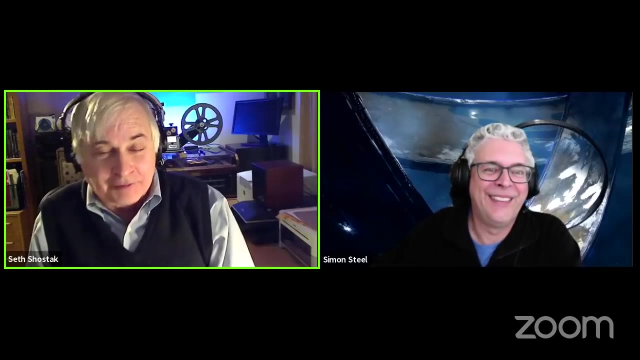 ways of thinking about life emerging on earth. um, one of the big possibilities is that some of the organics were delivered to our rock, uh, in this process very early on the solar system. so you know, that's, that's the sort of message. um, well, that's a good astrobiology project. 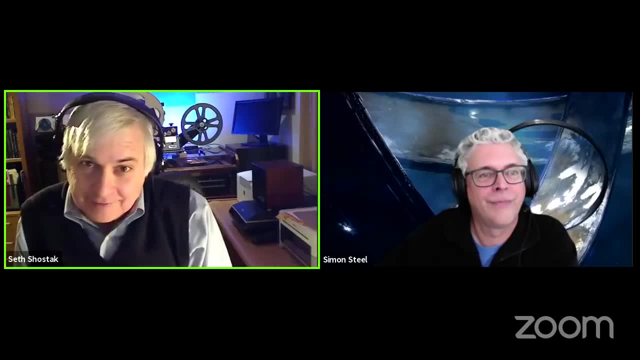 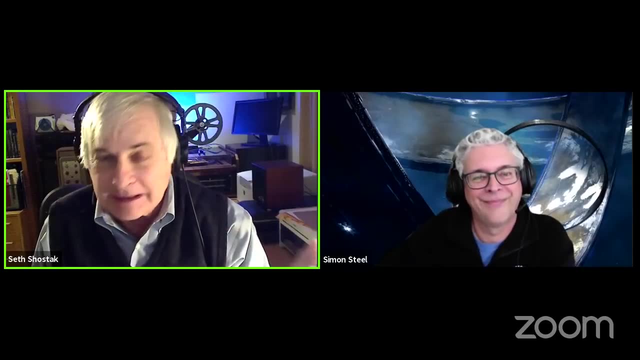 but there are people who have suggested that if you're a really advanced society, you want to spread your species around. it sounds like a well-known sci-fi film, but if you want to spread your species around, the thing to do is, rather than you know, jumping into their tummies. 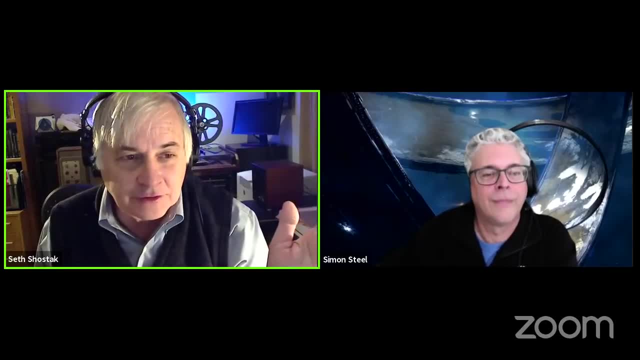 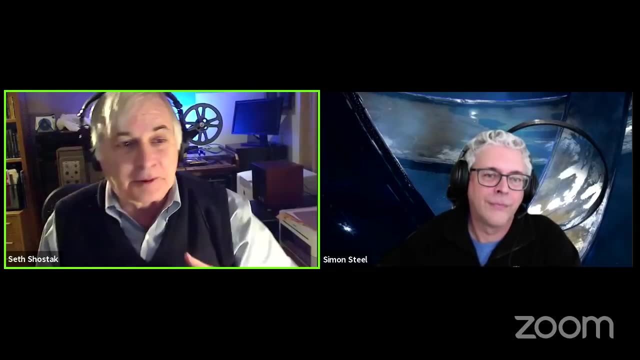 and exploding out and all that kind of thing. that's really difficult. that you just put genetic material or whatever is your genetic material might not be dna, of course- and you just put it in rocks that go from one solar system to the other and occasionally hit something and you 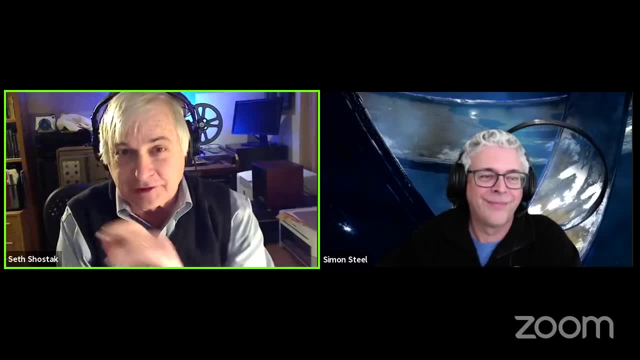 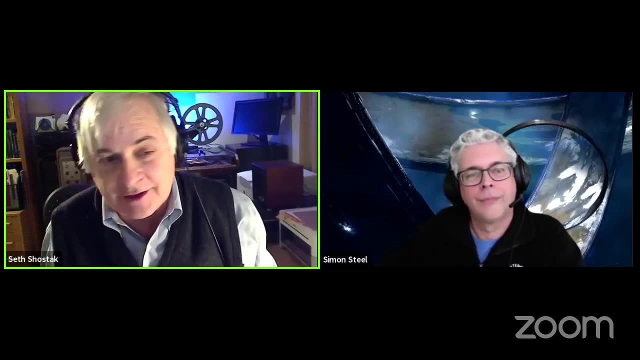 know, infect that world with your species. this has certainly been used for a number of reasons by hollywood, and you know it. it might happen, um, but you know, the problem i have with that is that again, it's assuming the aliens are biological, uh, and, and i think advanced aliens might much. 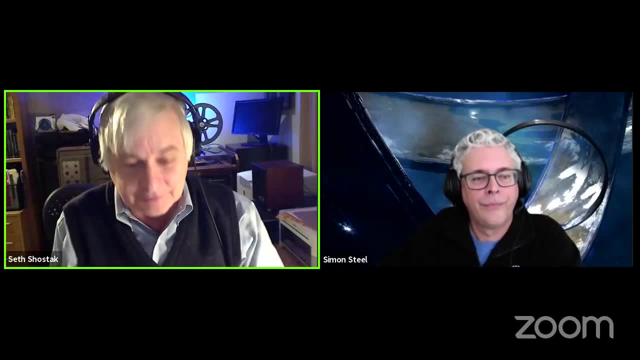 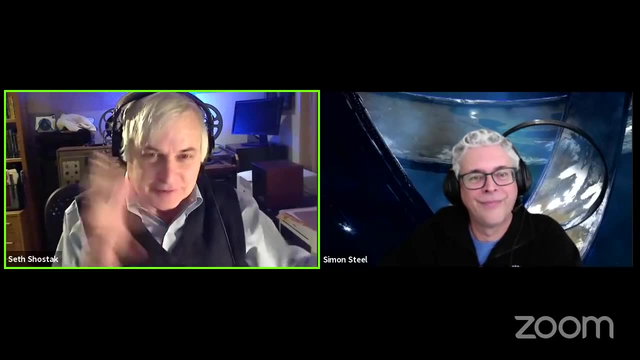 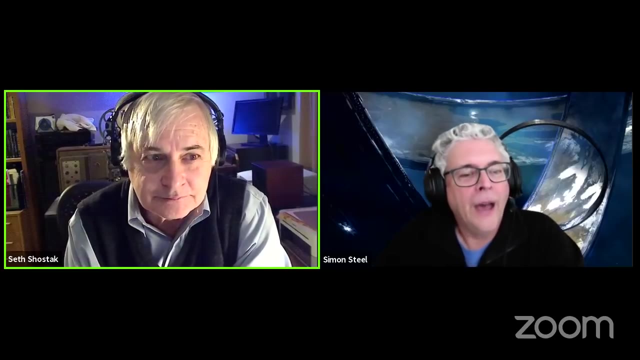 more likely be machine intelligence. but you know, maybe they just put some little self-replicating machine into a whole bunch of comments and send them out there and wherever they land they reproduce and build something, you know, impressive like the city of akron, ohio. um, here's another question, uh, about new ways. you know we've talked about radio astronomy and that. 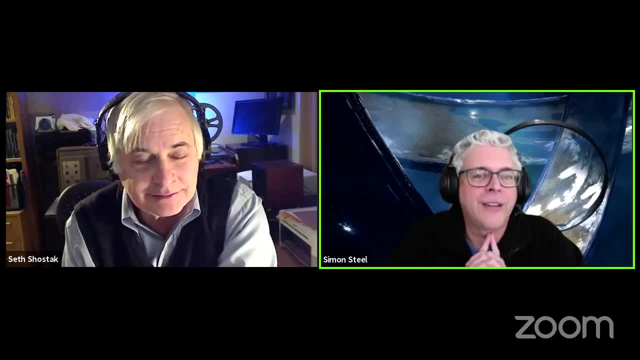 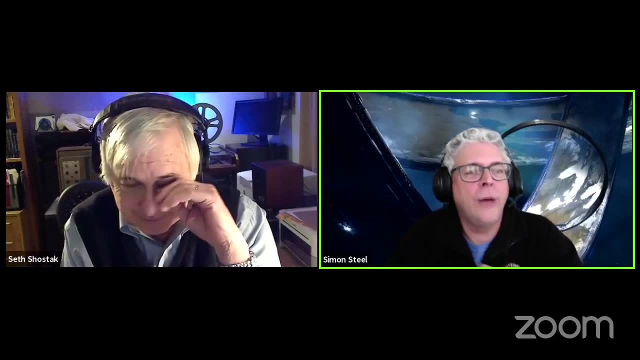 has been the the, the fundamental way to to detect techno signatures, and maybe that's a good time to to talk about the laser seti project at the seti institute. that how is it? how is new, how are new kinds of astronomy being used and how could they? they potentially be used for artifact searches? 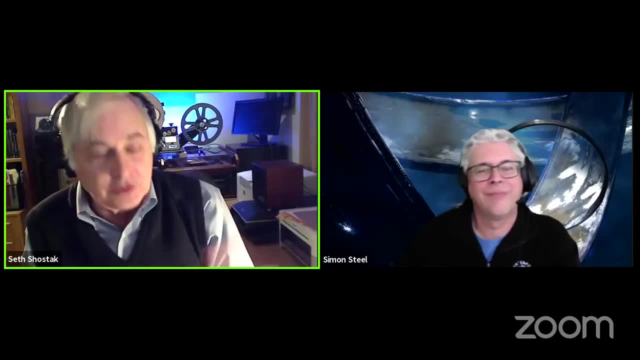 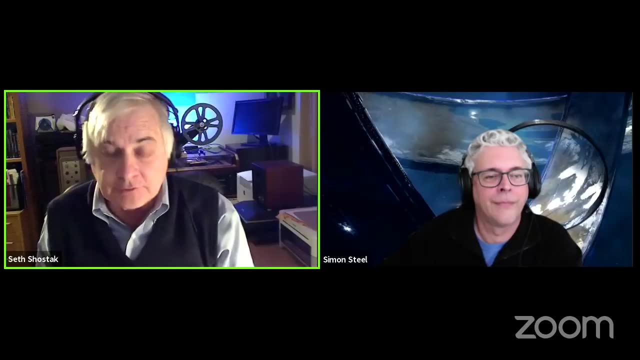 well, i think that there's hope here. i mean really there is. you mentioned laser seti and that that's a project of the seti institute as well as the university of california, berkeley, and others, and the idea is, instead of looking for radio waves, you look for flashing laser lights. now that has the same problem that i. 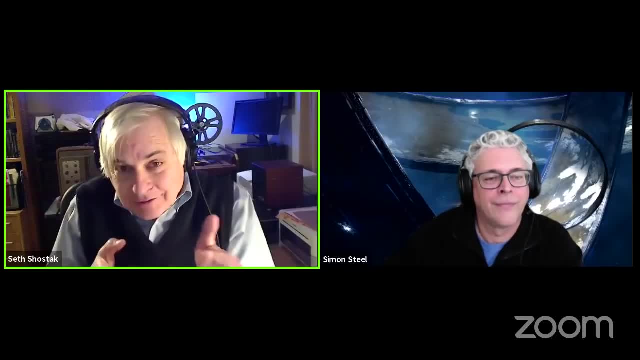 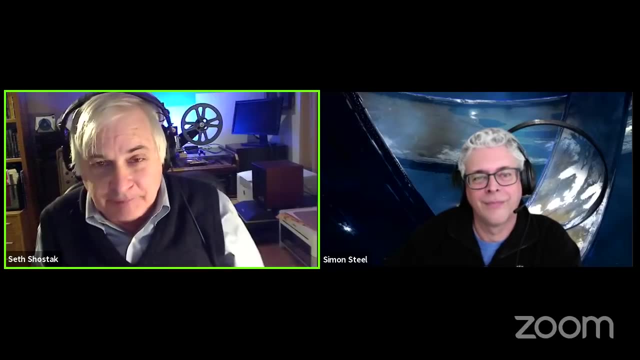 think the radio searches does. in other words, that either they're aiming their lasers at you for some reason, and if they're far away, they don't know. the homo sapiens is here because they haven't picked up our radar tv. so you know, it doesn't make sense for them to deliberately target us. 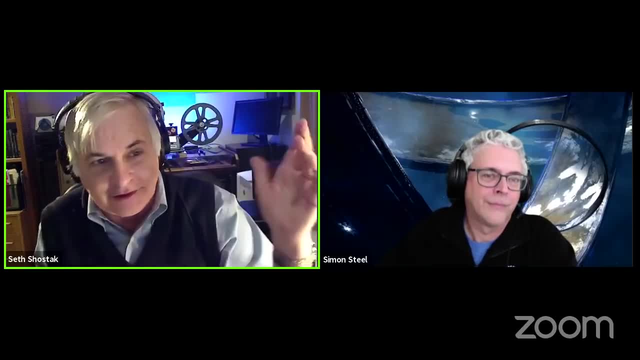 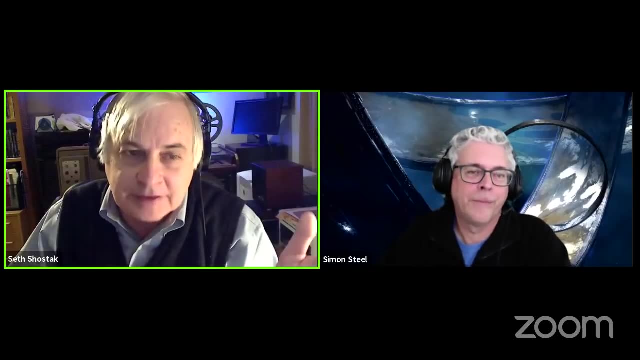 but maybe there's just a bright flashing light like the kind you see on you know the, the way that we see on the wings of aircraft, just to say you know i'm here, don't hit me, kind of thing that could be. but it has the same energy problems: the amount of energy required to make a light that. 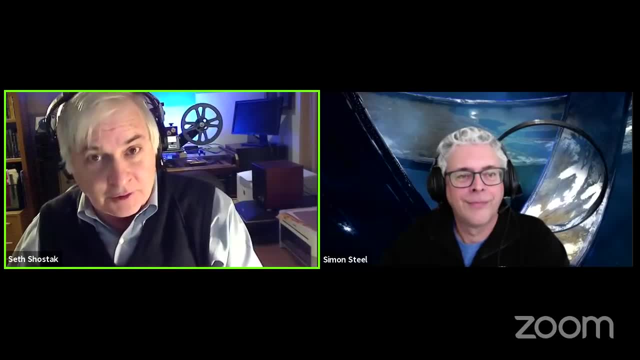 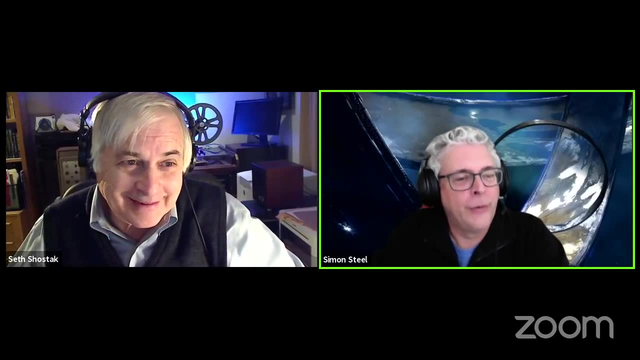 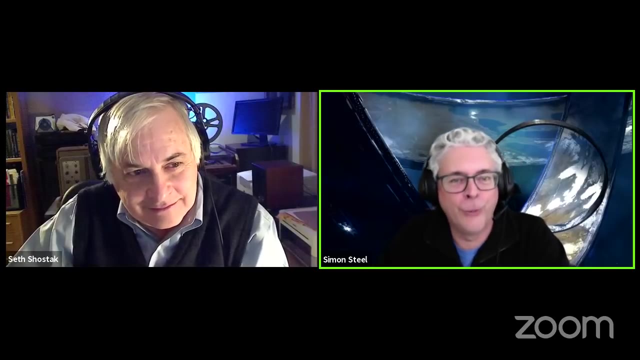 you could see from far away is is considerable. nonetheless, it's certainly worth looking for these sorts of things absolutely. um, there's a long question here and i'll just sort of paraphrase: um, there have been, you know, obviously there's a lot of data coming in from telescopes all over the 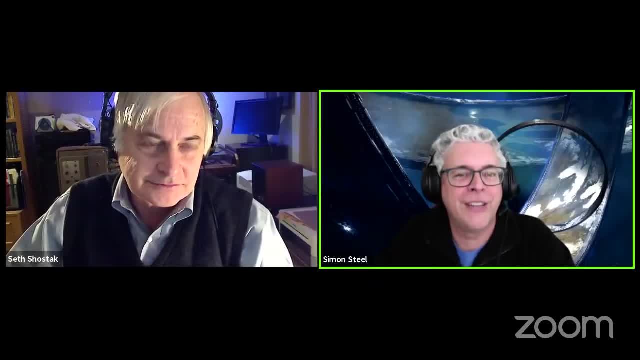 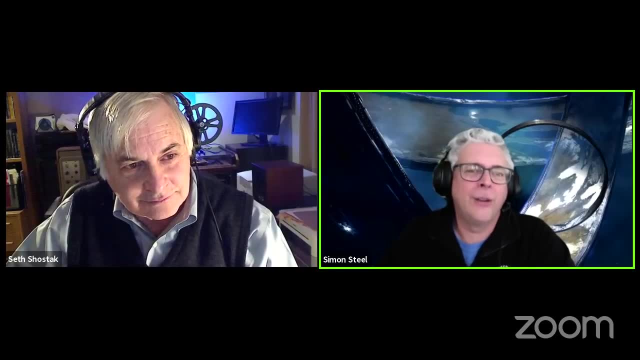 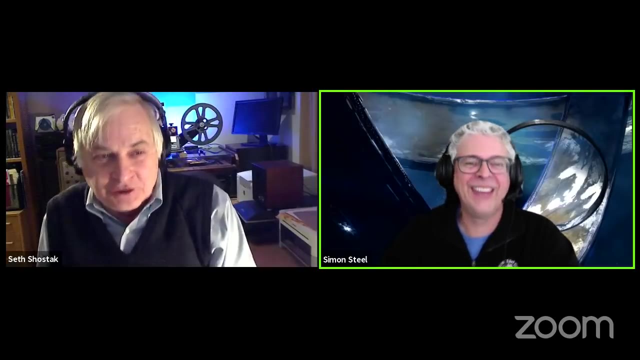 world. there have been some false detections, false alarms for the seti detections, um, are there any sort of things that you know still stick in your mind that you could have said? well, maybe. um, yeah, i do get asked that question. you have a drawer full of well, these are pretty. 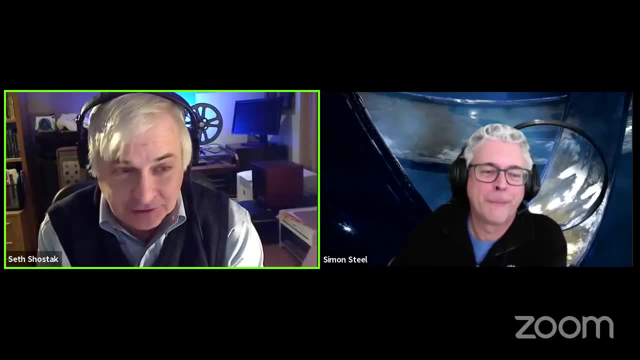 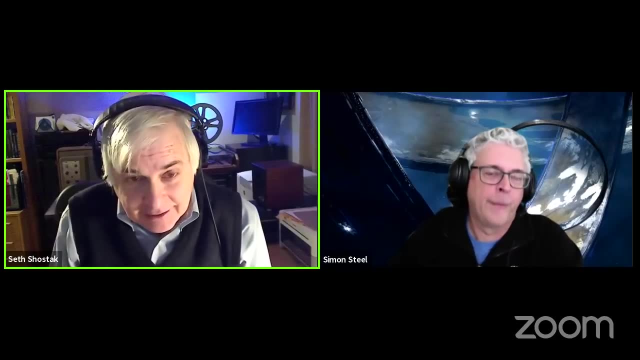 interesting here, bob. well, in the old days you used to get a lot of you know. we're not sure what it was because you would only see it once you know you'd. you're looking at the data, you know the time you. you looked at the data, you know. 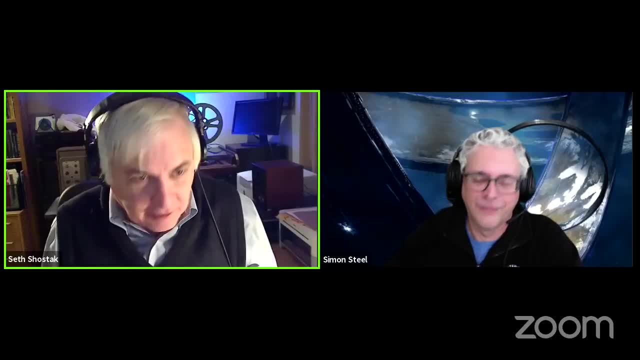 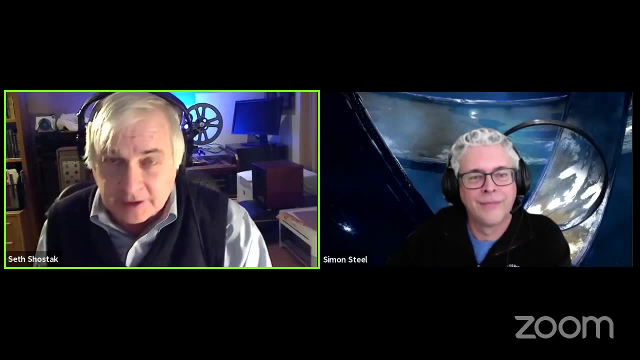 that was you. you took the data a week, a month, a year ago, and now you say, oh, there's something here, but you're not at the instrument anymore, you're not at the telescope, so you can't kind of follow up now these days the kind of experiments that are done at the seti institute. in any case, you 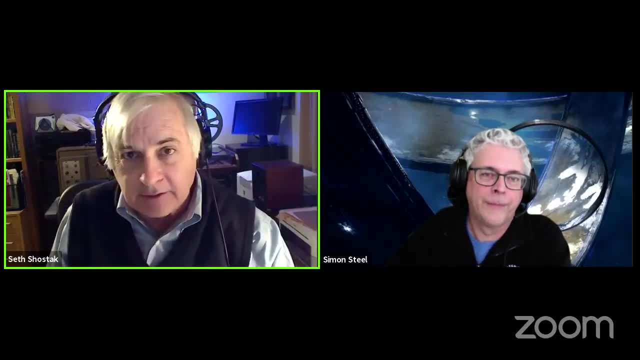 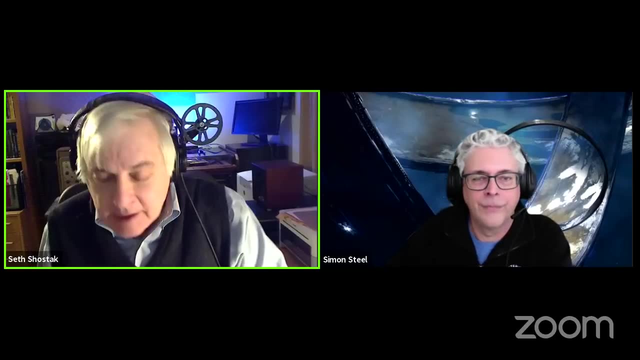 know you follow up right away you find something interesting. you don't sit around and debate whether you should follow up. the machine automatically does that within a minute or two. so you know that that we ever found something. well, people will say: you know, are you close? right, i got a question, you know. 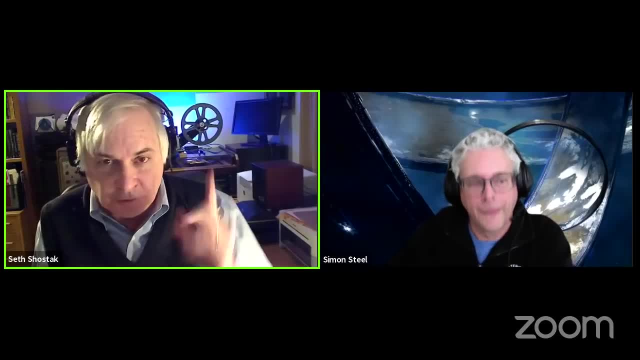 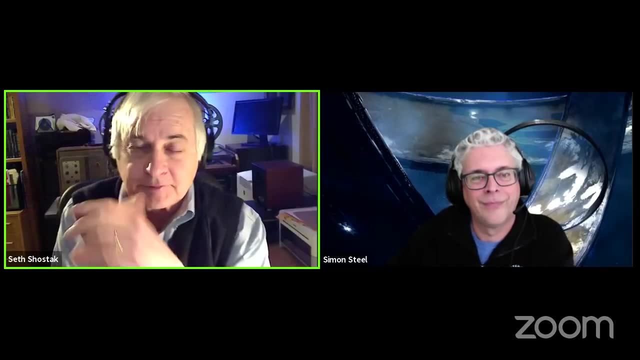 you can't say whether you're close. either you found it or you haven't. this is, this, is it's a one-bit experiment, it's zero, zero, zero. and then it might be one, and i usually say- and this is of course probably unacceptable, but it's like pregnancy, right, you know? are you close that? 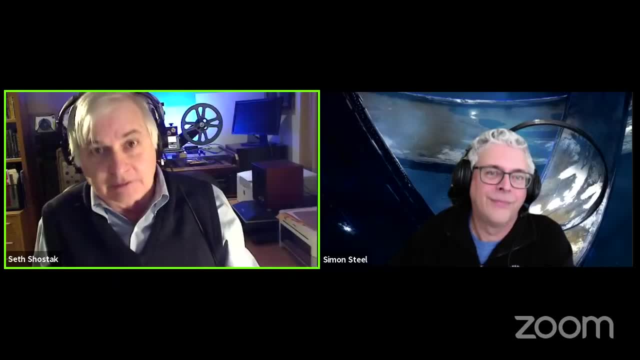 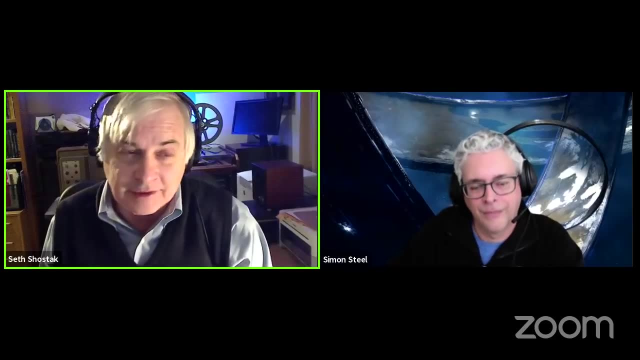 doesn't mean anything. either you are or you aren't, and it's the same thing here. until we find a signal, all we can say is that we haven't. people ask about the wow signal. that's certainly intriguing, but it was only seen once, and until you see it twice, you can't say that you found it. yeah, yeah. 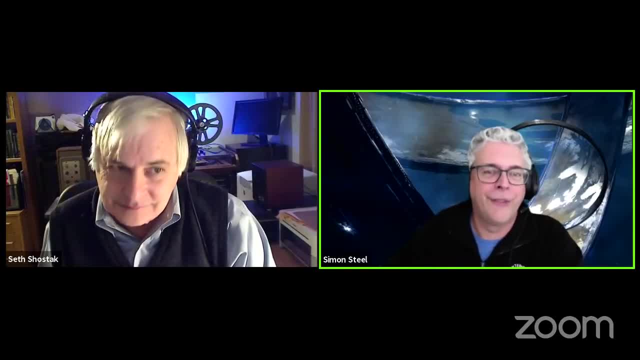 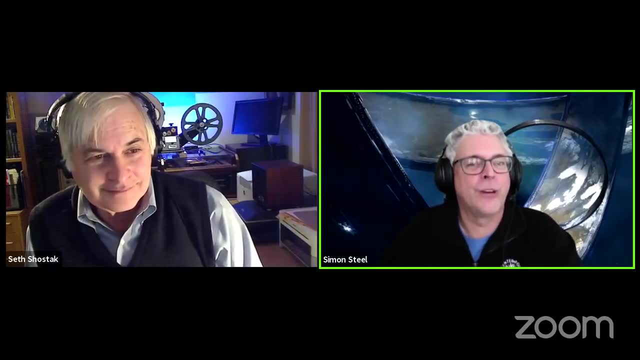 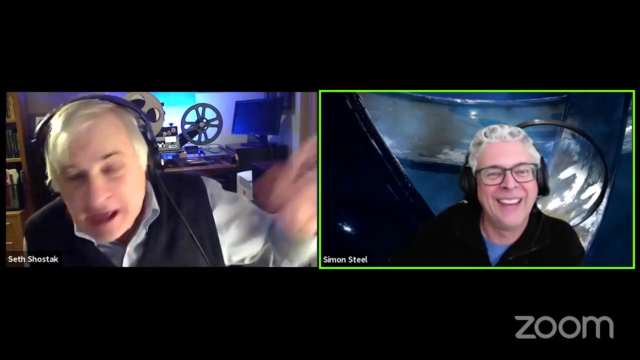 it's just, that's how science has to work. you, you need that verifiable observation and independent verification, and that has not happened yet. um, unless there's one of those files in your cabinet that, uh, that has a very big padlock on it, i must say, but, um, anyway, if i had that sitting here. 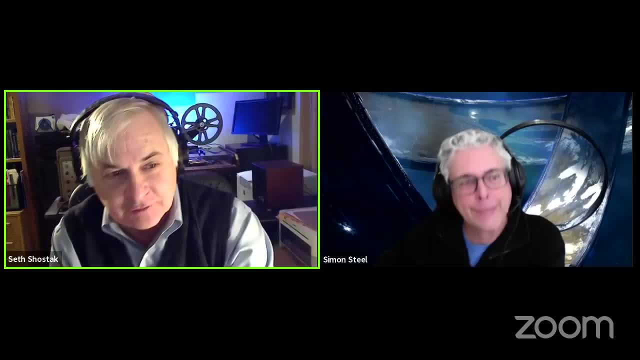 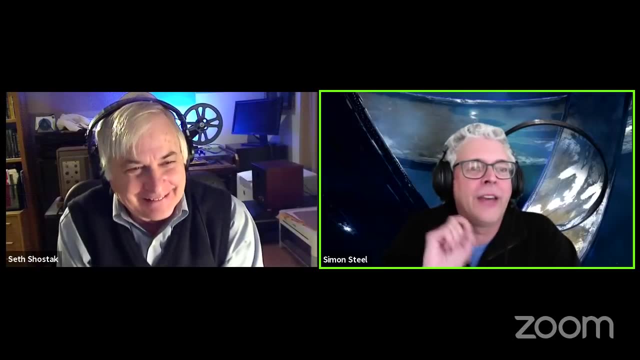 talking with you. i mean, i would open that up and you know, just book ticket to sweden and collect the nobel prize. yes, and that brings me to one last question for the audience, and that that is, uh, the process of, of, of, of announcing a discovery, um, and this obviously, 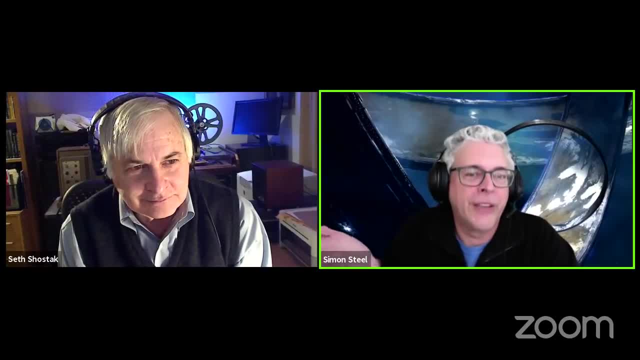 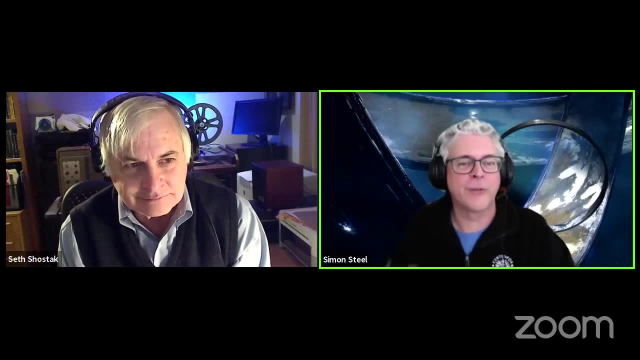 as we've just said, you can't just just detect a signal one night and then then go out and make an announcement: um there's, there's a process there. and uh, what sort of process would we need to to go through? well, there is an official protocol, but it's not terribly helpful because it simply says: 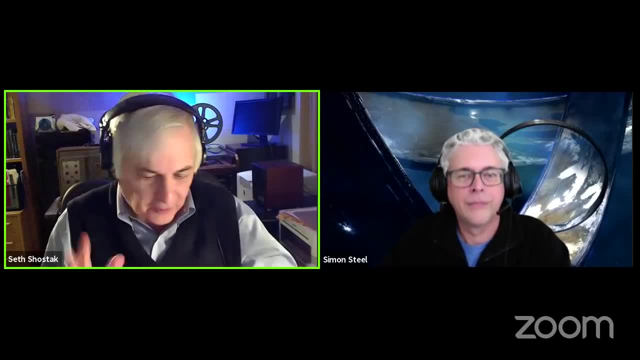 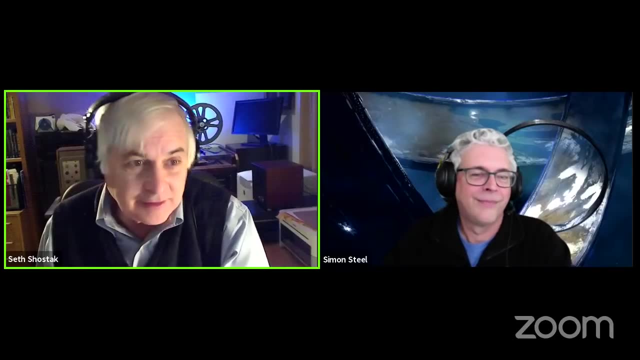 you know, check it out and tell everybody and you know, don't broadcast anything back until you talk to other countries or whatever that kind of thing. those protocols do exist, but they're they're just sort of a, you know, like signing the pledge on your exam book, on your blue book. 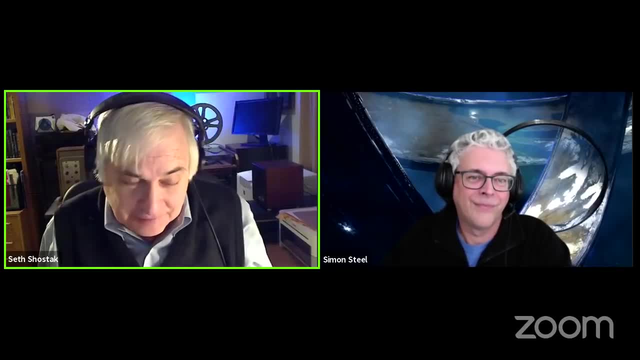 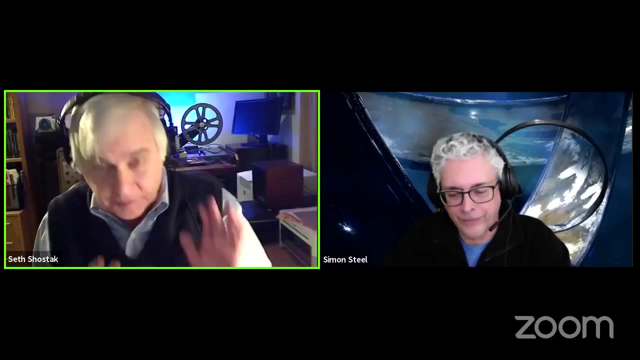 i will not cheat. right, i mean it, it might help, probably does help, but it doesn't guarantee that you didn't cheat. so what really happens- and i know people have a hard time believing this, but what really happens- is if you find a signal that looks good immediately. 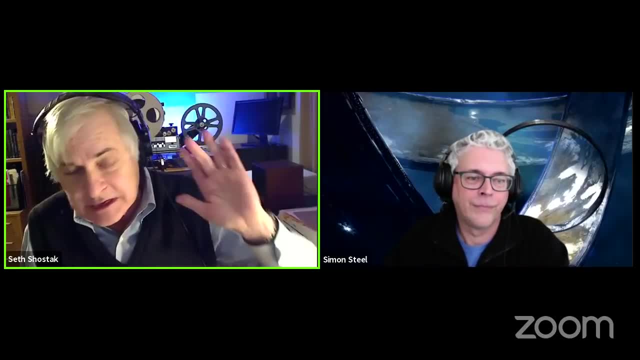 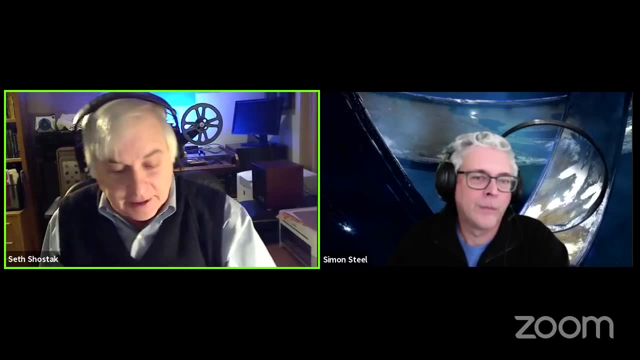 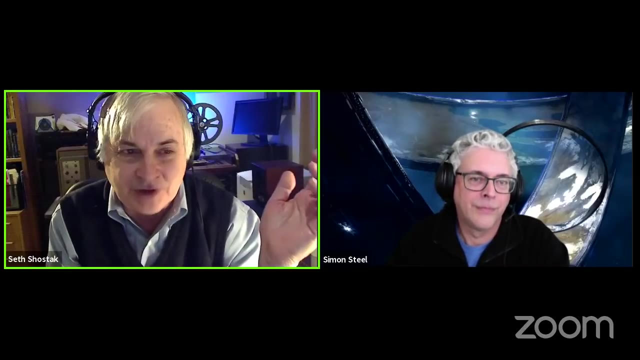 the media, you know the local tv stations or radio stations, the, the newspapers, the bloggers- everybody starts getting in touch with you because there's no policy of secrecy. so everybody is, you know, messaging all their friends: hey, we got something interesting here, even though it might turn out to be nothing a day later. so the way it will be dealt with is that it will simply 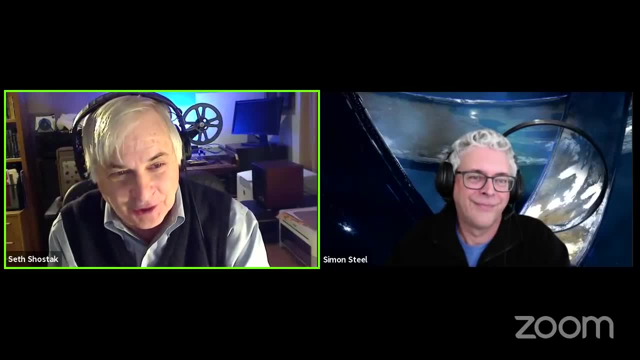 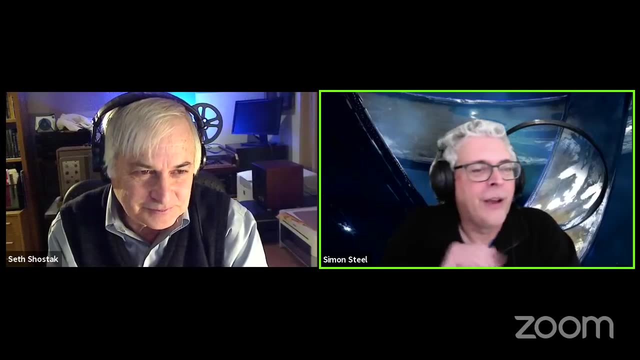 be a big story, and then everybody in the world who has a telescope right will start looking in this direction. you can be sure of that. yeah well, thank you very much. i see another donation, steve. thank you very much, steve um, wherever you are, that's. 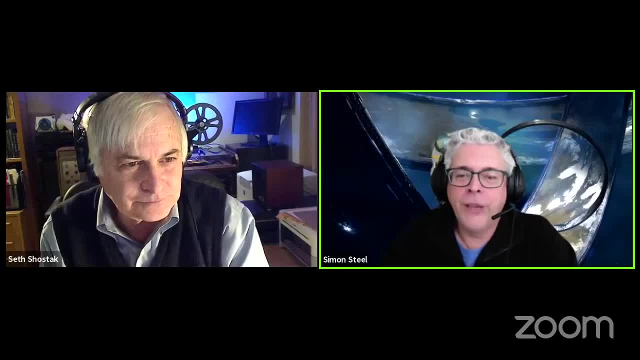 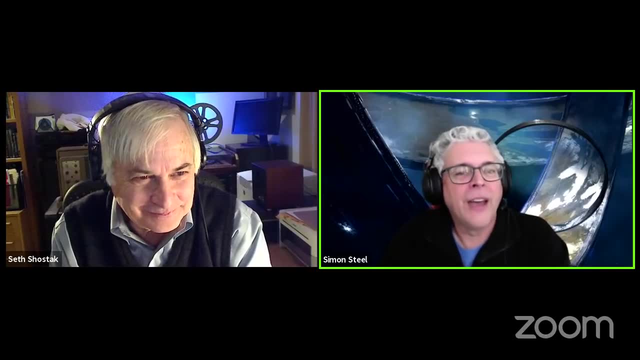 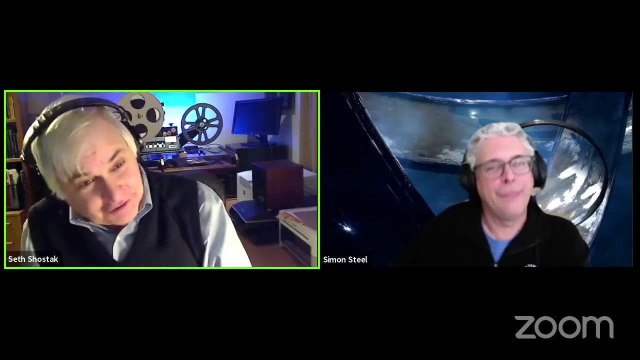 wonderful. um. so, seth, if i, if we gave you quite a large budget and, and, uh, not much limitation on real technology, what would you build? uh, to leave a legacy, a visible legacy for humanity. yeah, well, oh, you mean something. yeah, something big, something big. yeah, gotta be big. well, i mean certainly, 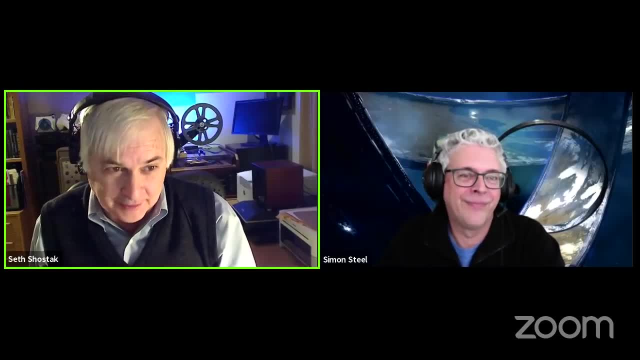 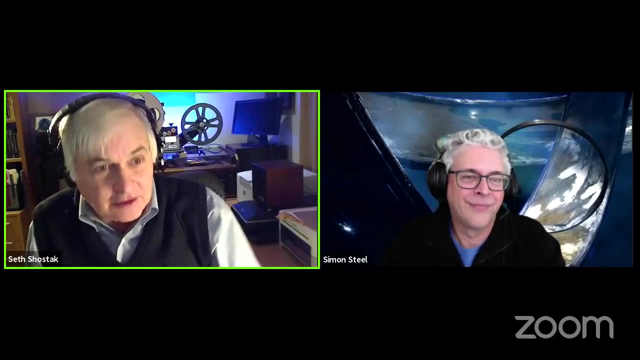 infrastructure, where there's enough energy comfort up there's real energy consequences, where you have wind and a lot of things, which i think is the extremely obvious thing: putting a lot of power sats into orbit. that's been talked about for at least 30 or 40 years, and keep in mind that. 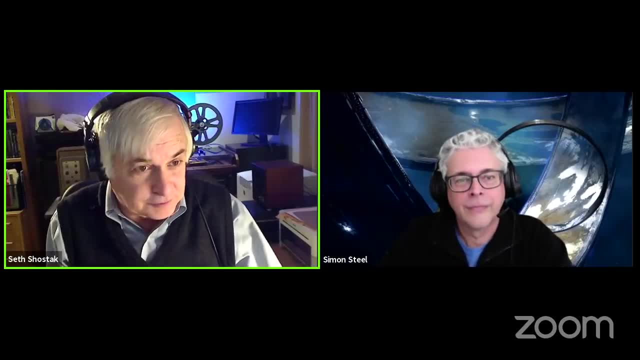 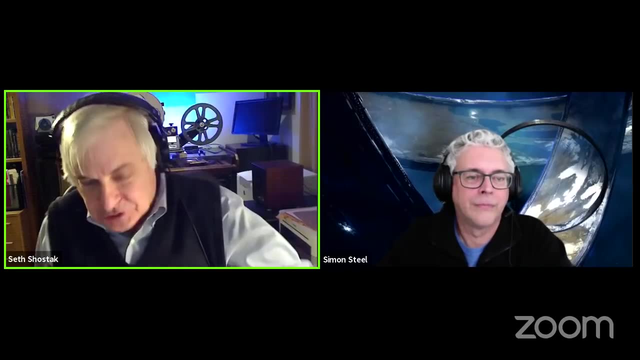 it has the advantage: not only can the energy be inexpensive, because to make another kilowatt hour of energy doesn't cost any more than the last kilowatt hour- you don't have to burn anything, you just collect sunlight, and of course it produces no pollutants to the atmosphere in the 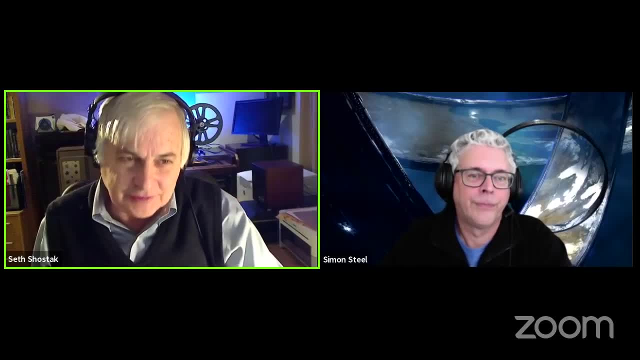 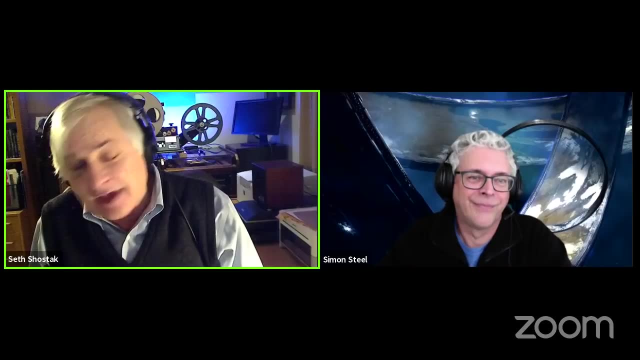 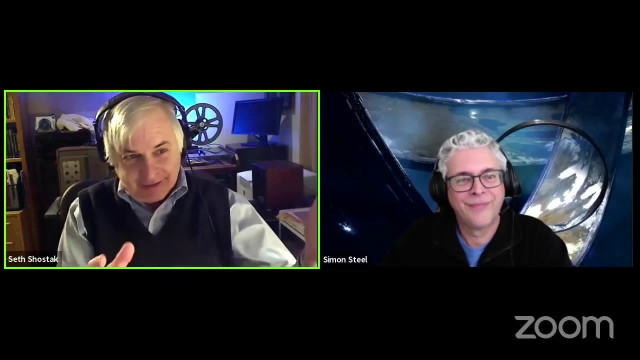 usual fuels it's, it's the capital cost, it's just a money of sorry, a matter of economics. but what i would build to la to, i suppose i would put, i would make a reporting of the entire internet and put it on some sort of medium that could withstand the cosmos for a billion years.